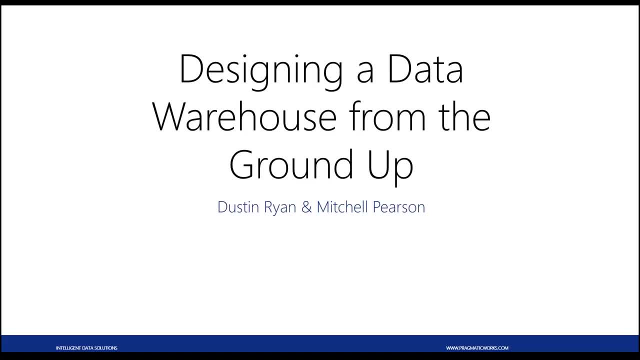 You just want to keep in the back of your head when you're designing your data warehouse for analysis services. Now, if you're not going to be using analysis services for your data warehouse, that's okay. You're still in the right place. We're just going to point. 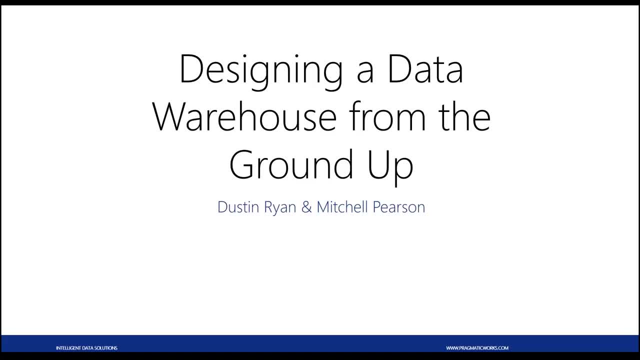 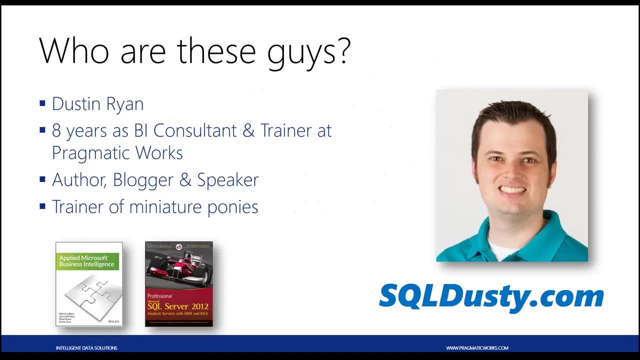 out some extra things along the way for those of you in the audience that will be looking to leverage, really, the strengths, the reporting strengths, of analysis services. Okay, All right. so my co-presenter today is C Dustin Ryan. He's been at Pragmatic Works for eight years now. Now, what you might not 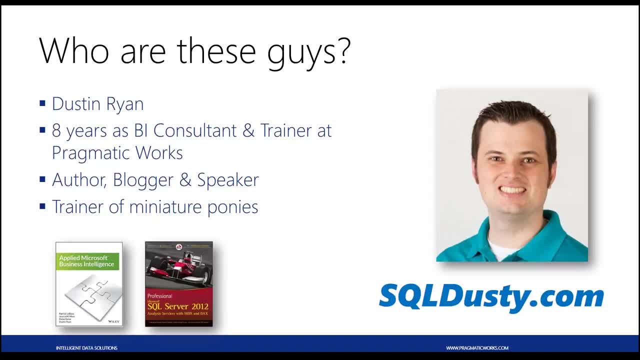 know is he spent the first six and a half years as the janitor but fortunately for him he's learned a lot in the last year and a half and he is a BI consultant here at Pragmatic Works. He's also a trainer. He teaches our SSAS master's class, our MDX class. He's 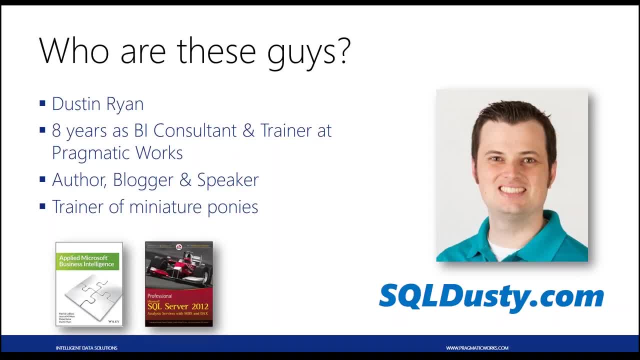 a wealth of knowledge. If you go to his blog, you'll see he has over 100 blogs on just those two topics. He is an author, a blogger and a speaker. He's written two books. You'll see them on your screen here. He's written two books. You'll see them on your screen. 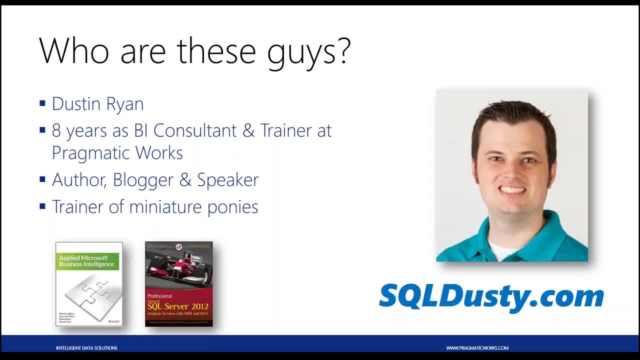 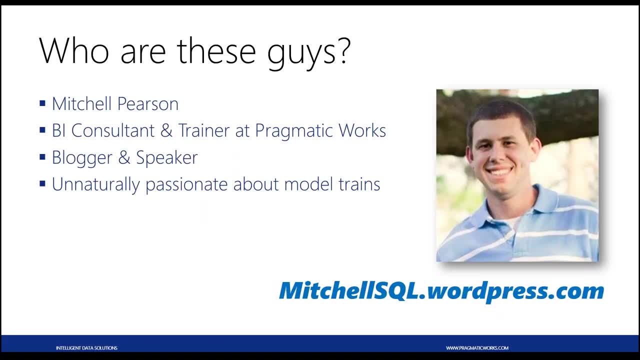 here. and he is also a trainer of miniature ponies. I can't make this stuff up. They're so cute, They're so precious. and this here to my left, here is Mitchell Pearson. He's also a BI consultant and trainer at Pragmatic Works. He teaches the intro to SSIS class. 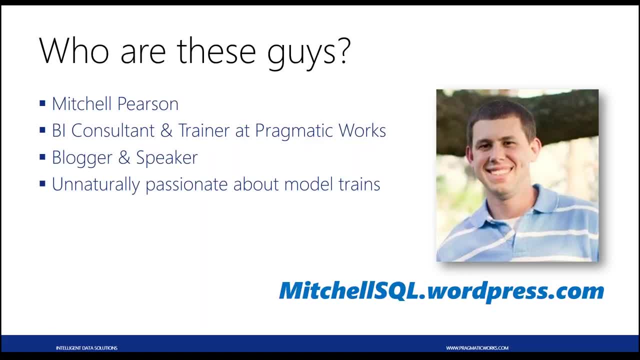 He also teaches the SSIS master's class, so he knows a lot more about me than SSIS Great resource there. so if you have any questions about SSIS, you definitely need to look up Mitch. He's a blogger, speaker and he really has this very uncomfortable, unnatural passion. 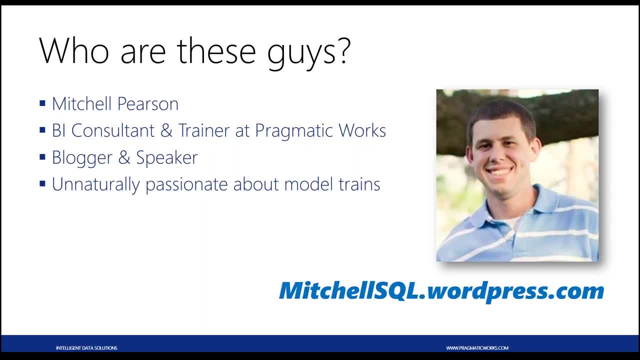 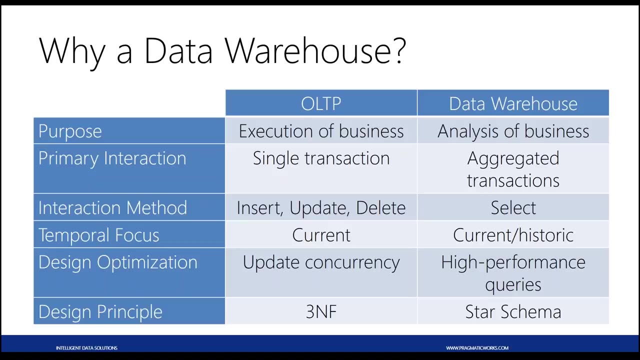 about model development. He's got costumes and everything, so I don't want to go too much detail into it, but throw that out there. You can find his blog at MitchellSQLwordpresscom. We're going to get started with talking about before we get into designing a data warehouse. 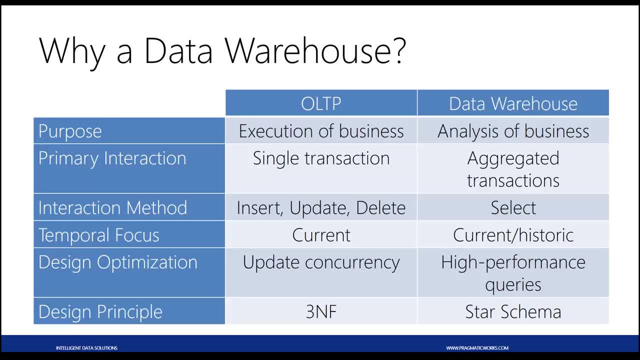 why do we want a data warehouse, Mitch? can you think of any good reasons why we might want a data warehouse? Actually, I'll give you a little story. I like stories. I like stories too. Once upon a time there was a little bank. This bank was a little. 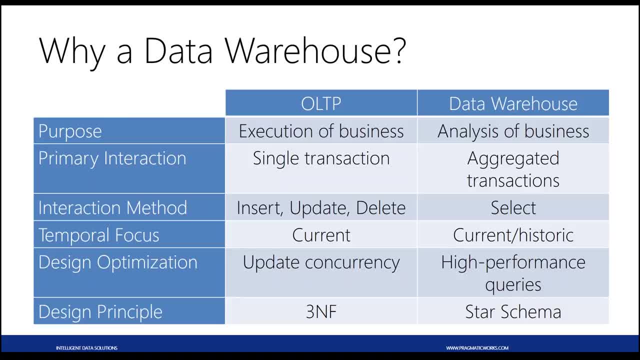 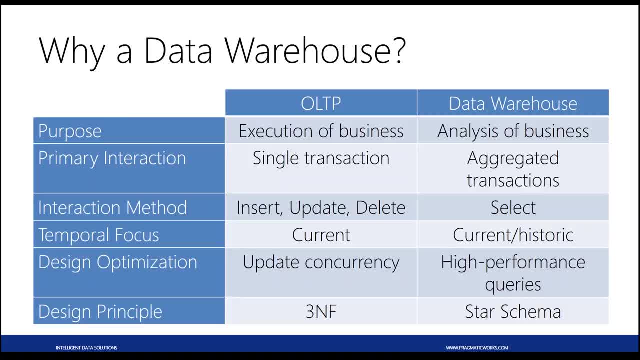 Hey you guys, Can you hear me? You just lost sound Guys. Hey, We're having some audio. Yeah, Can you hear us? okay, Yes, I can hear you. All right, I'm not sure what the issue is. Excellent. 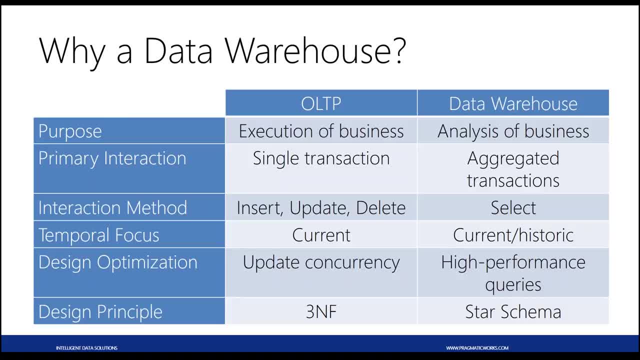 Excellent, were telling a little story. I'll start over from the beginning here. once upon a time there was a little bank and this bank wanted to have these awesome reports for analysis, but unfortunately they didn't have a data warehouse. and this is a true story. we won't name the bank- and this bank built these reports. 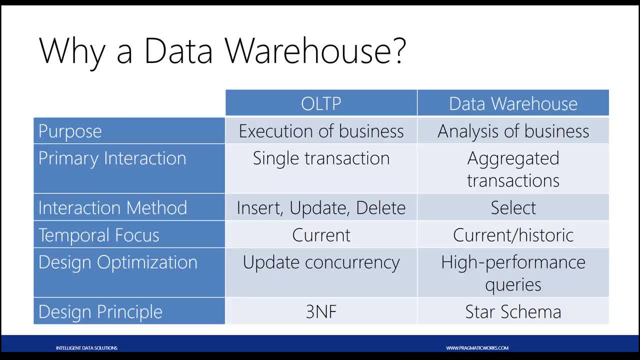 off of their transactional system and, unfortunately, when they built these reports off of their transactional system, their transactional system crashed and it took down all of the ATMs for the bank. the end: okay. so what you're telling me is that somebody went home early that day, permanently, permanently. 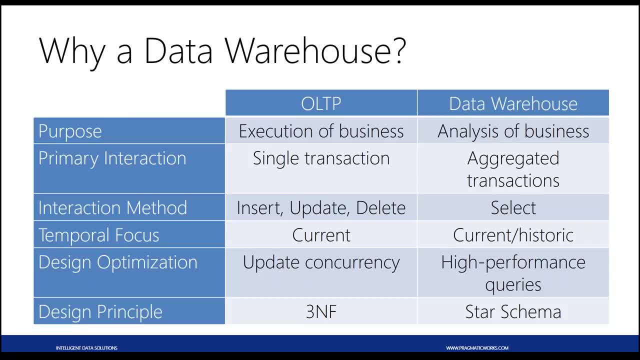 okay, so that that is one really good reason why a data warehouse is something that you want right for reporting, right historical reporting, you know what? there's certain reports that you definitely don't want to be running off of your data warehouse now. so that's a kind of a scary story, but those kinds of 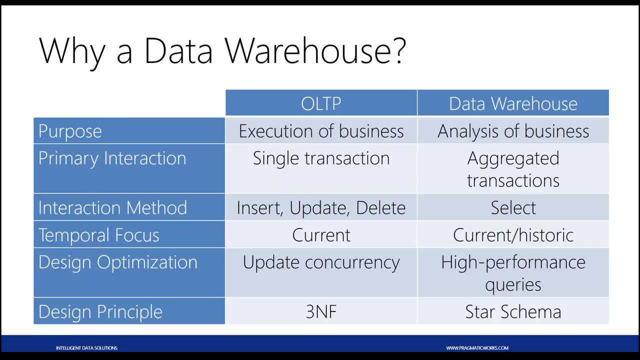 things happen, and so that's a. that's one of the really good reasons why we want to consider using a data warehouse. now, when we're talking about data, data really boils down to two different types. you have data that supports the execution of the business, and then you 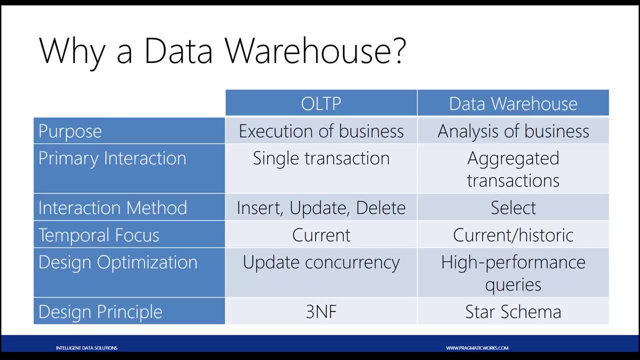 have data that supports the analysis of the business. so, when we're talking about data that supports the execution of the business, it can be, you know, a retail business. it can be a banking, be transportation, energy, manufacturing. it can be any type of business, and we have data that supports the business. so 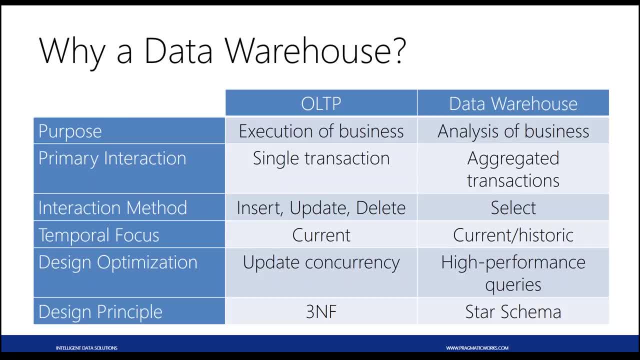 somebody is buying products, somebody is logging inventory, somebody's doing something that helps the business run, helps the business make money. so that's the execution side of the business. then we have the analysis of the business. how many cheese balls did we sell last quarter? what are the account balances that we're looking at right now? 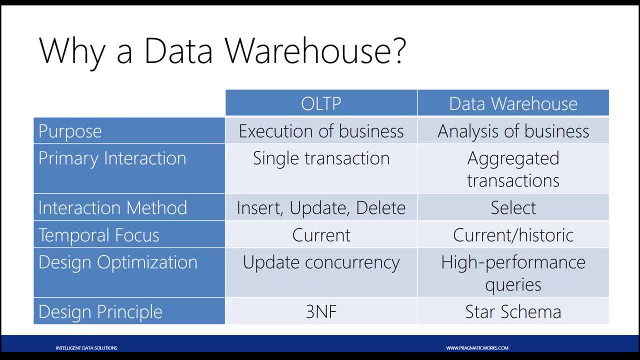 how much freight did we ship or how much freight are we going to ship. so that's the analysis side of the business, and so that that's two of the main differences between the OLTP, or your transactional system, and your data warehouse, your dimensional model, your star schema, whatever you want to call it. that's the 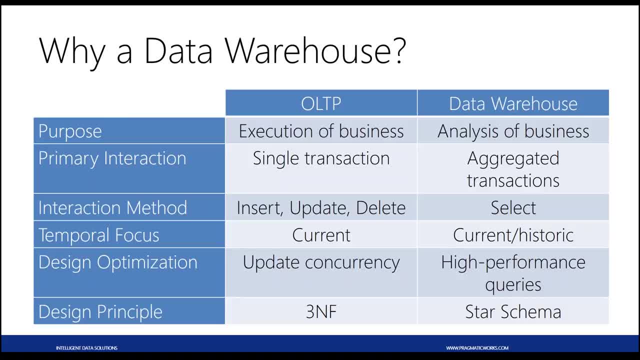 analysis side of the business, so huge differences there between a transactional system and the data warehouse also have. how does the user interact with that, with those two different systems? that that's another big difference between systems. so when you have a transactional system, primarily the interaction is going to be at a very 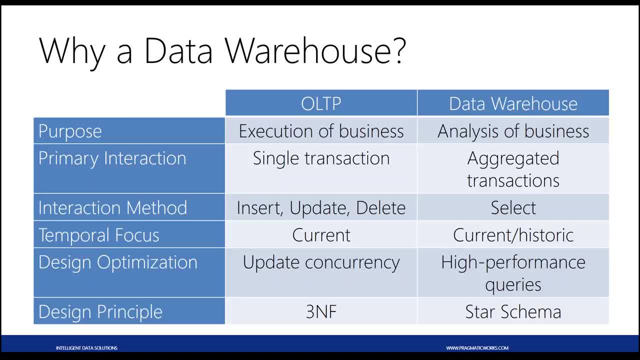 atomic level or a very granular level. somebody's going to insert a new transaction. a customer walks into a store, they buy a product, they say: give me a cheeseball. we insert a record into the database, into the transactional database, because some- a new customer- has bought another sheetball. okay, that's the 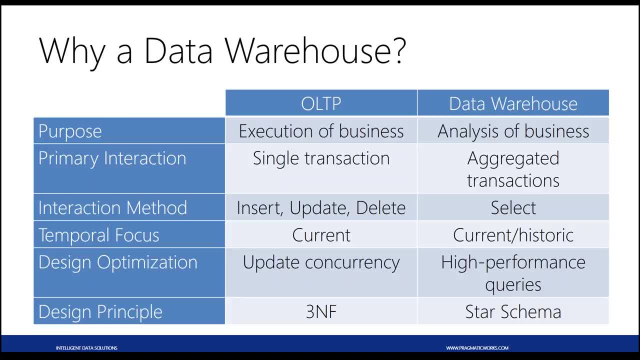 transactional side. now, with the data warehouse side, the transactions are going to be a lot different. right, we want to be able to upload all of yesterday's transactions, which could be 50 million, 100 million, whatever the number might be. we want to insert all 50 million transactions from yesterday up. 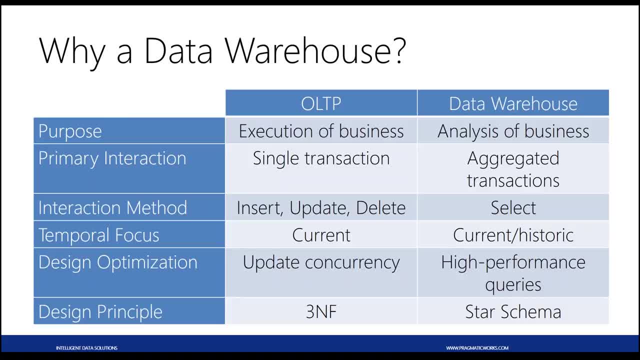 into the data warehouse so that way we can be in reporting off for reporting on it. now it could also be we want to read a 50 million records so I can figure out how many cheese balls that I sell yesterday. so the user interaction is going to be different now. the, the, 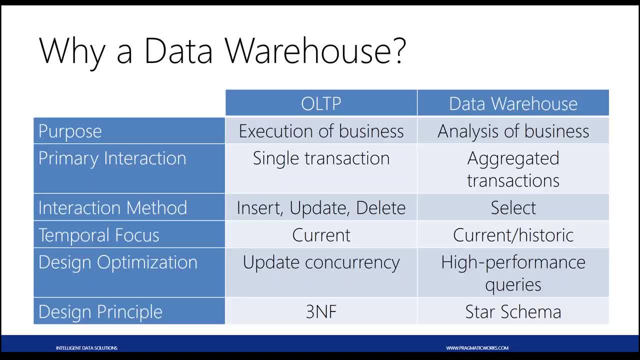 management section is going to be different, so we're going to need to. method of interaction or the types of queries that are going to be run are also going to look a lot different. When we're talking about a transactional system, you're going to have 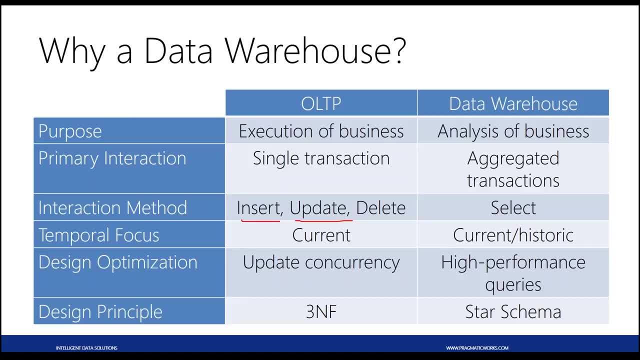 atomic inserts, atomic updates, deletes. We're going to insert one record at a time, update one record at a time, delete one record at a time, And the primary method of interaction with the data warehouse is going to be select. Yes, you're going to have inserts, bulk inserts, right? 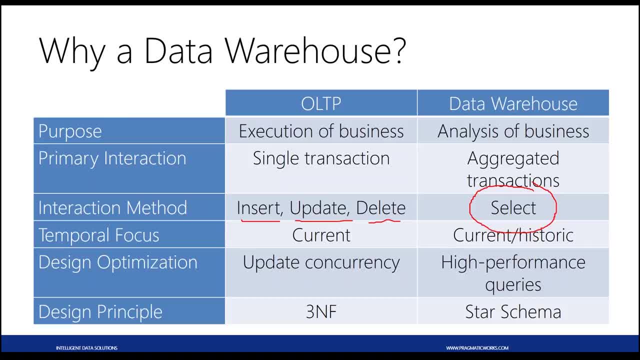 We're going to insert 100 million records at one time from whatever happened yesterday in the business, Or we're going to select 100 million records at a time because our users are running queries that they're asking: Show me how many sales transactions I had yesterday or how many. 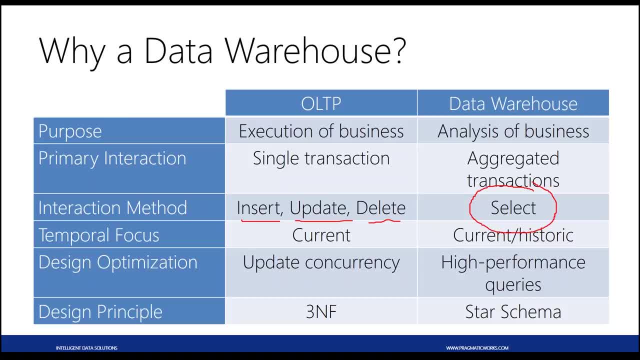 cheese balls. I sold yesterday Those types of queries. Another difference between your transactional system and your data warehouse is going to be the temporal focus right. Usually in a transactional system the temporal focus is going to be what's happening now currently in the business. We're not tracking a lot of history in the business outside of. 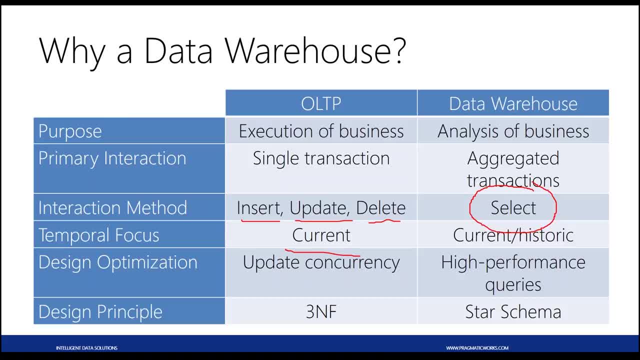 what's happening in the business. So we're going to select 100 million records at a time. What's necessary just to keep the business running. With the data warehouse, we're going to have what's going on currently right, And there may be a little bit of latency there. Maybe we're 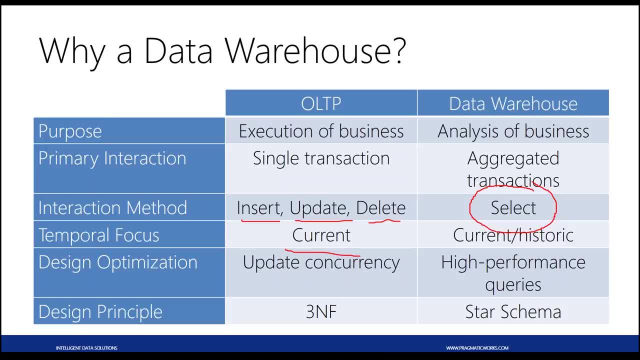 only keeping. maybe there's like a day latency. We update the data warehouse daily And so it takes a little time for the current data to make its way into the data warehouse. But we also keep history right. Maybe you want to keep three, five, 10 years history. I don't know Whatever. 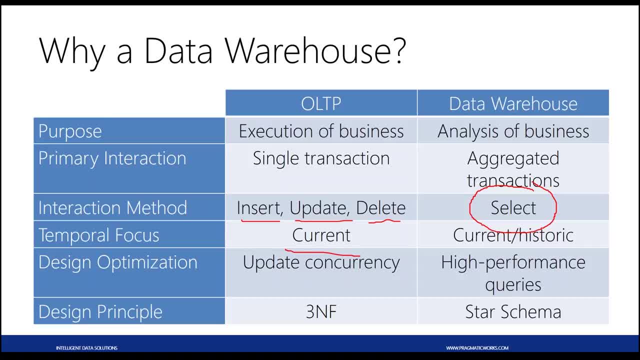 your business determines is appropriate. You want to keep that history in your data warehouse as well, So that way we can do analysis over time, And then we're going to have a little bit of time. So are we selling more cheese balls this year than we sold three years ago? Now also the 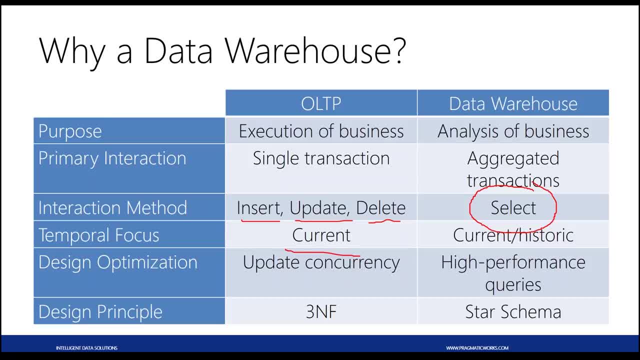 difference between the transactional system and the data warehouse is going to be the design optimization right. Typically with a transactional system you use a third normal form type of design because we want to be able to optimize lots of inserts happening at one time, So we may have 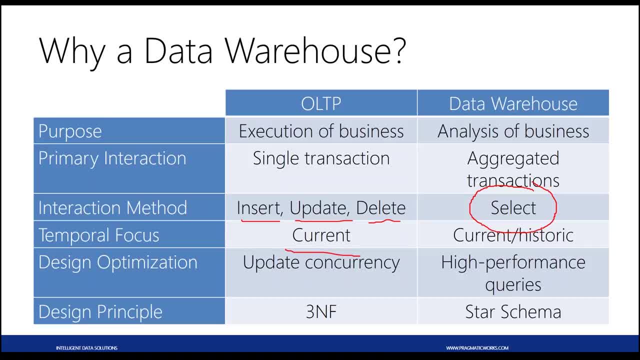 10,000 purchase orders coming in in a given hour, And so we want to be able to insert and update those all at the same time. So we want to be able to optimize those all at the same time. That's how we'll optimize our transactional system. Now, with the data warehouse, we want to optimize. 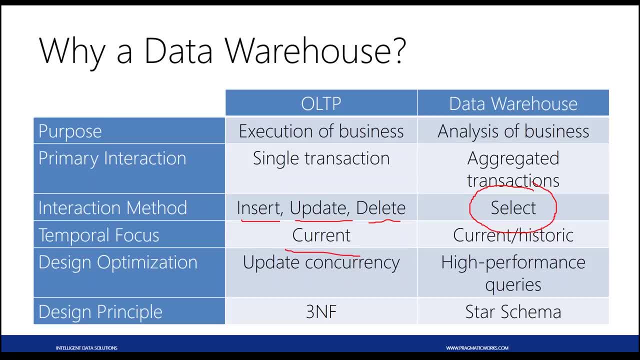 for high performance queries, And that's really the main purpose of designing the data warehouse. the way that we're going to talk about is we want to be able to get the data out of the data warehouse as fast as humanly possible, So that way, our users' queries don't have to run very, very long. This is also important. 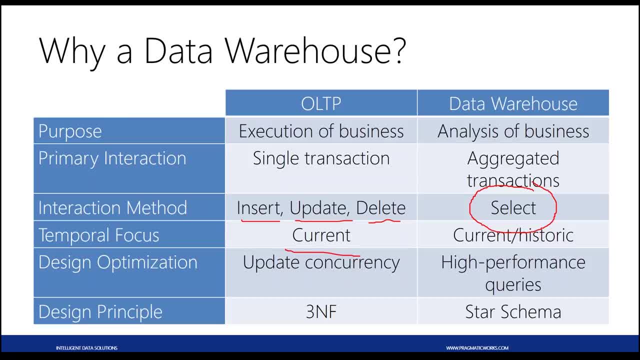 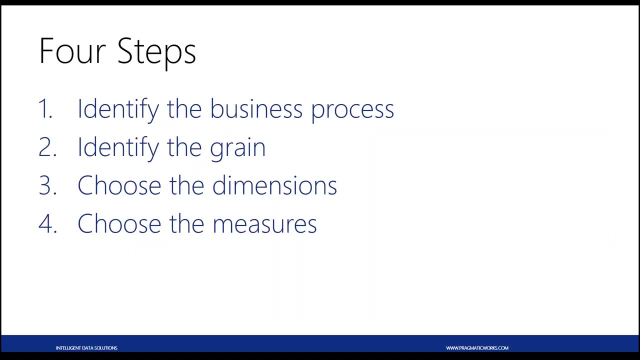 for analysis services, processing, And we'll talk about that a little bit here later. Okay, Now, the four steps that we're going to talk about are identifying the business process, identifying the grain, choosing the dimensions and choosing the measure. So these are kind of the 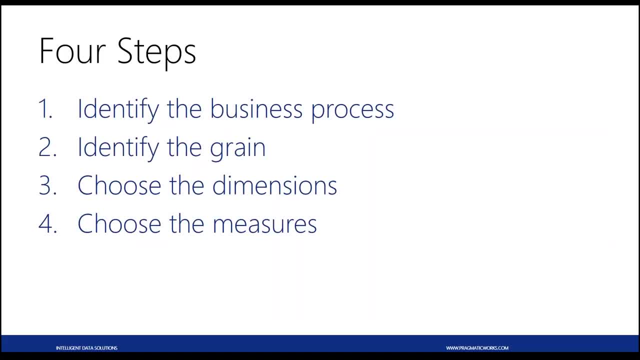 four can steps that you can use when you start approaching either building a data warehouse from scratch or enhancing a data warehouse. Maybe you want to bring in a new business process into your existing data warehouse. Maybe in your data warehouse you've got retail stuff already and 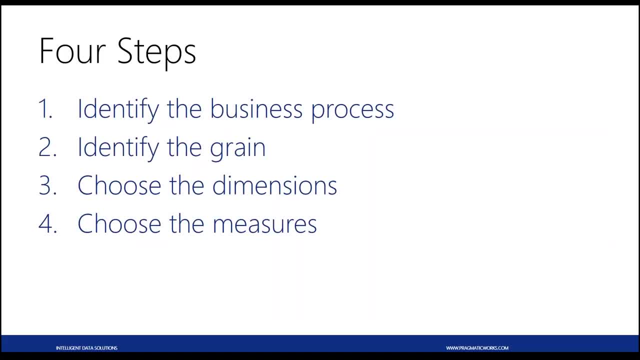 you want to bring in some marketing, marketing facts, so you can use these four steps to kind of approach enhancing a data warehouse as well. and and as we're going through these steps, I want you to think about and remember that the the purpose of a dimensional model, a well-designed dimensional model, or star. 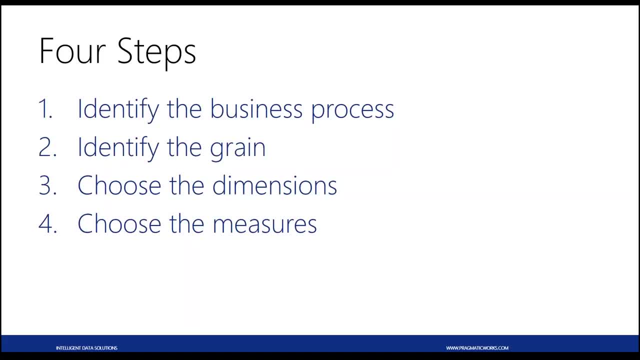 schema is. we want it to be simple, right. we want it to be easy to use. we want the ETL to load these tables to be as simple as possible. we want our queries to perform well, and we want this to perform also perform well with SSAS. so let's. 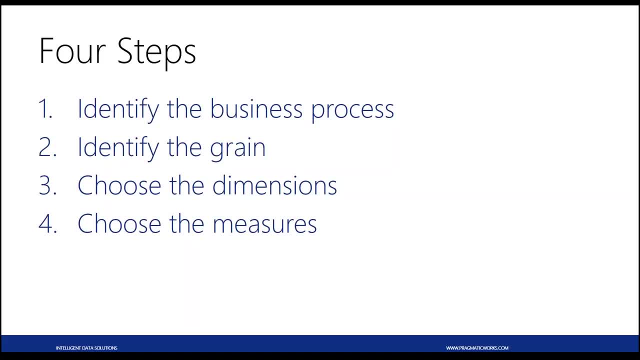 start walking through these, these four steps here, and and as Mitch and I go through these steps together, one thing we're going to we're going to do is we're actually going to design a data warehouse together. so we've got this kind of imaginary business, a very successful business model. you've 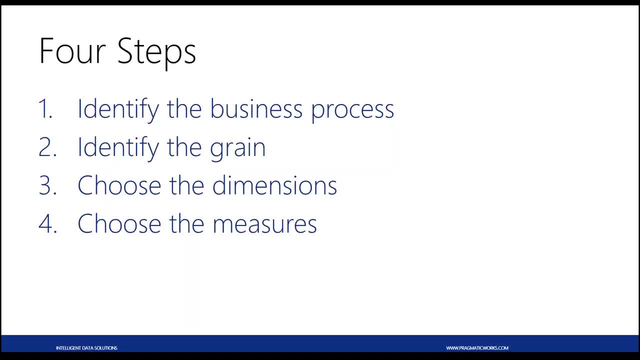 probably heard of this company. you've probably heard of this company, Buster Block. they said they sell a rentals to VHS movies- very successful in the past, and so that's kind of our imaginary scenario we're going with here. we're going to design a simple star schema for this business. okay, and so. 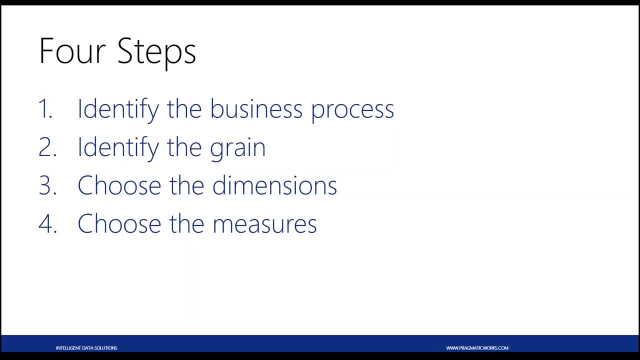 we're going to walk through these four steps together, keeping in mind that we're designing a star schema for Buster Block, all right, so remember that. and so we're going to kind of approach it from that standpoint. so that way we can talk about these four steps, but you can also kind of see it in practice and you can. 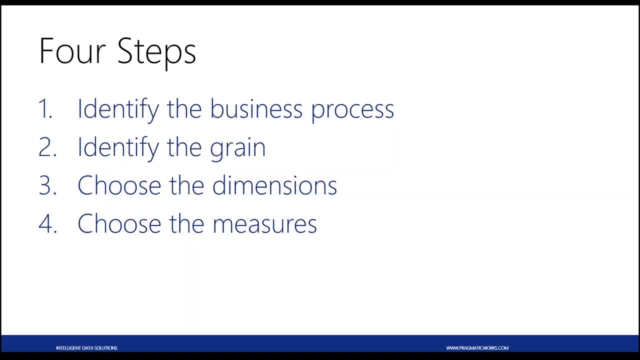 kind of have a good example of you know using this in your particular environment. now the the reason we're going with a retail example here is that we don't want to be complicated. everybody understands how kind of how retail work- somebody's buying a product right- and so we don't want to get lost. 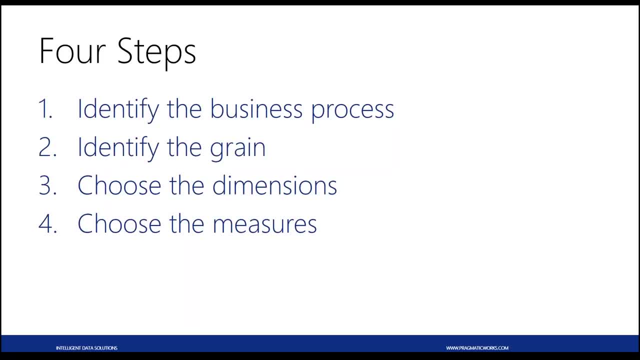 in the minutiae of you know how the business actually works, or you know the, the technology or from that kind of standpoint. so we want to go with something simple, so it's easy to understand and we can focus on actually learning the concepts of Buster Block. 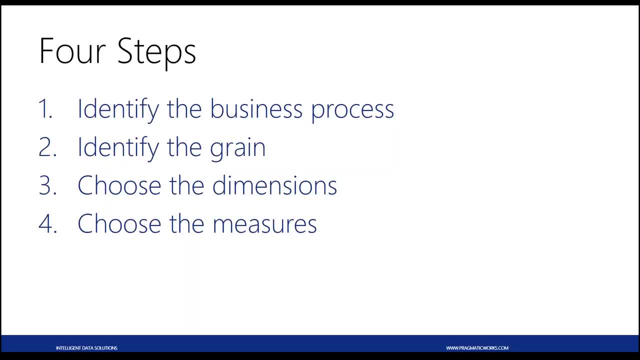 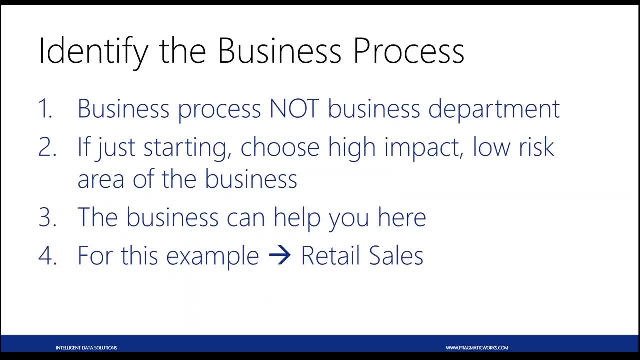 here, so we're going to start with identifying the business process. all right, thank you, Dustin. so identifying the business process is going to be the first step in designing our data warehouse, and the question we want to ask there is: what is a business process? a business process is a natural. 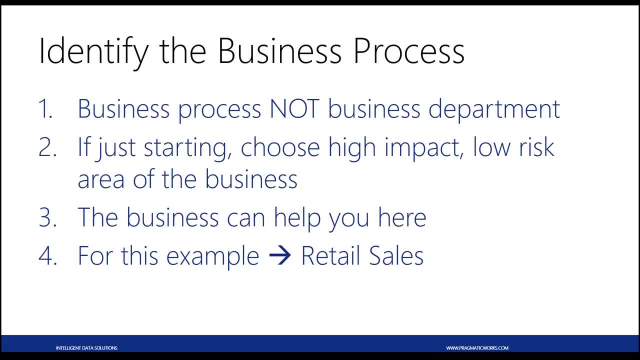 business activity performed in your organization that is supported by some form of data collection. it's important to focus on the business process as opposed to the business departments, because this will allow us to deliver information across the business process, and we're going to talk a little bit about. 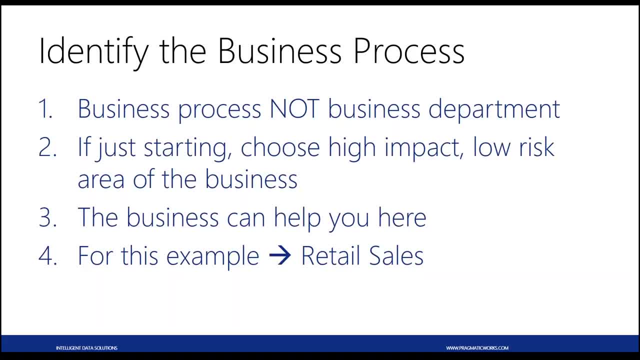 that, and then we're going to take a look at the data warehouse. and the data warehouse and what it does is it allows us to process the data in a more consistent manner. otherwise, we may duplicate data. if you think about having a data warehouse in multiple locations in your business, for example, having a 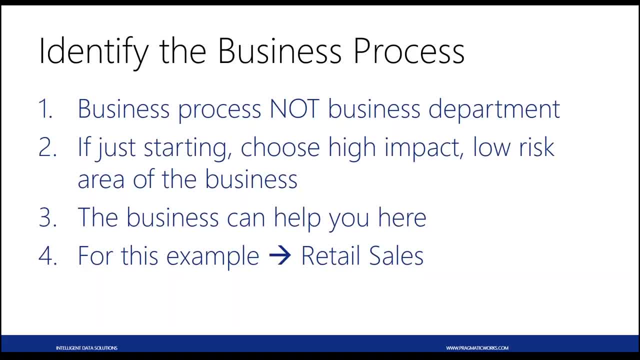 retail data warehouse and marketing, and then a retail data warehouse and sales. we may have duplication of data. that's not necessary and we want to have one centralized location for that information. so what you're really talking about here is having that one source of the truth, right? we want to. 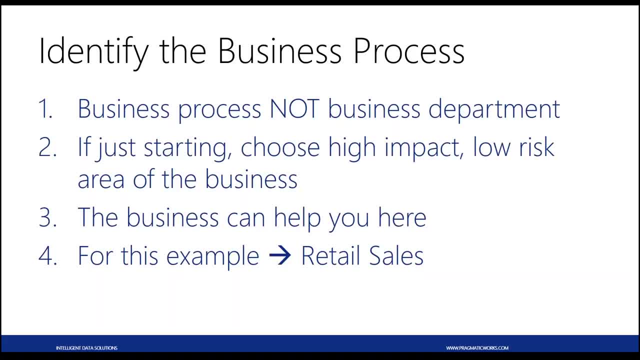 focus on business process, not business department. what we don't want to happen is to have marketing have their own data warehouse, manufacturing have their own data warehouse, and then everybody showing up to the same meeting saying, well, this is what our profit should be for this past quarter and everybody's. 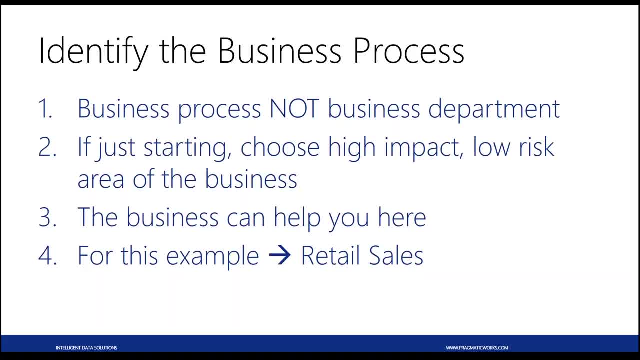 got different numbers, so we're talking about focusing on the business process that may span across business departments. exactly. good job, Dustin, all right, so we must first decide what business process we want to model. there's two steps that we want to identify when we're modeling our. 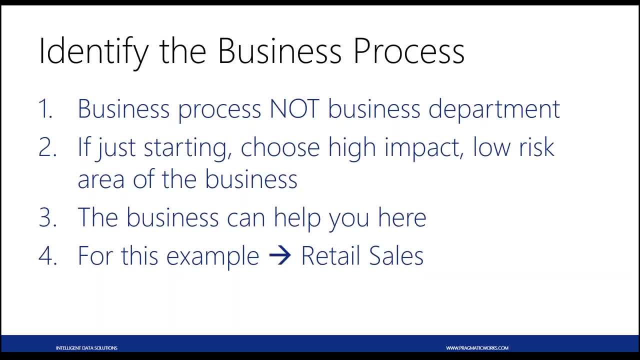 business process. we want to look at the impact that this business process is going to have in our data warehouse and we also want to look at the risk that's associated with this business process. so the impact is going to be reports that your business want on a daily basis- very common everyday impact. 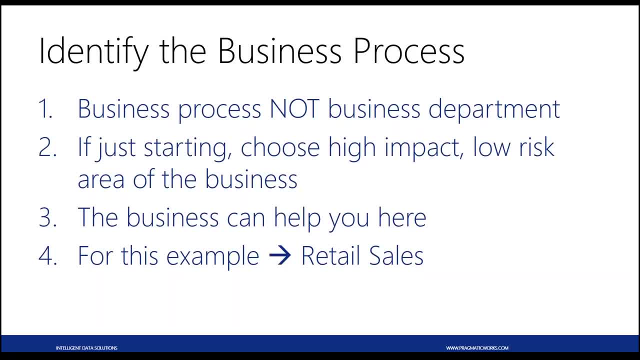 high availability reports. the risk associated with this business process are going to be things like data availability. can we have access to the data or is it going to be difficult to get? do we have data quality problems? you might want something in your data warehouse, but when you look at the data, 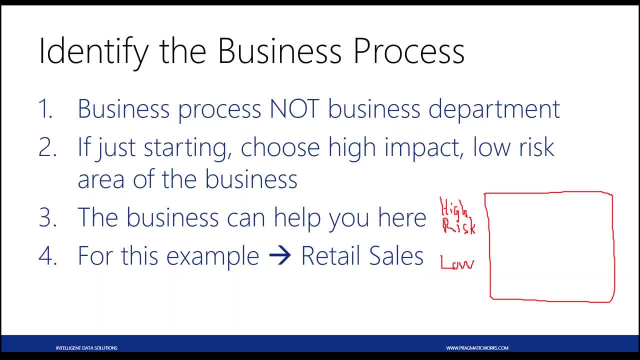 it's very unclean and it's going to take a lot of work to get that clean for your data warehouse. the third thing there is you might have very complex business logic that has to be applied to actually get that data warehouse up and running and it might be difficult to get that information from all the different 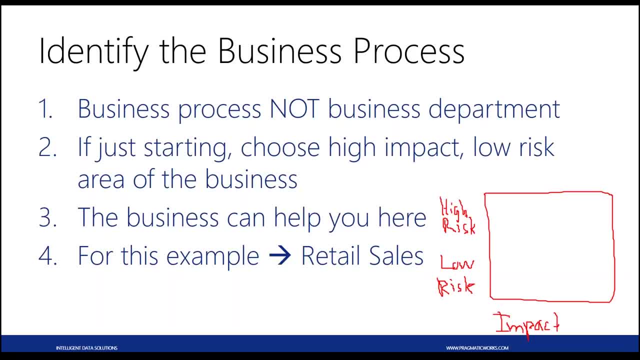 departments. so we need to assess the impact and the risk, and both of those have to take place as part of choosing the proper, choosing the proper business process. all right, and the other thing we want to do is we want to make sure we choose the business process that has the most impact from the beginning. we want 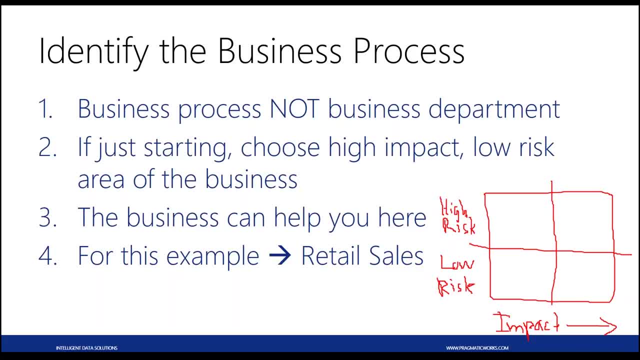 to get that low-hanging fruit. so when we start our data warehouse project, chances are we're going to have multiple business processes that are going to be identified. we're going to have more than one. we're not going to have, you know, just one process. we're going to see three or four or five different. 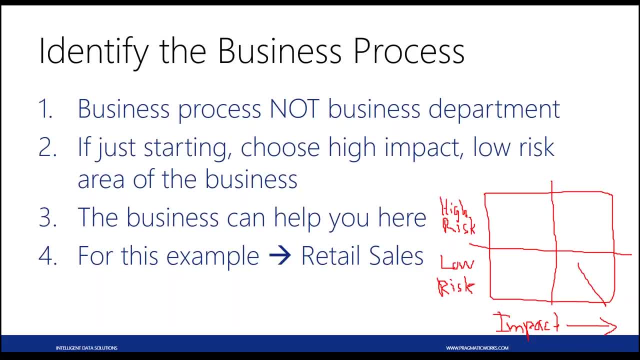 processes that we're interested in. all right. so chances are we're not going to be able to fit all of those business processes into our data warehouse. we're going to have to choose one or two or three or a couple of those, but we won't be able to fit all of them in there. this is where I mean: what's that? what's the? 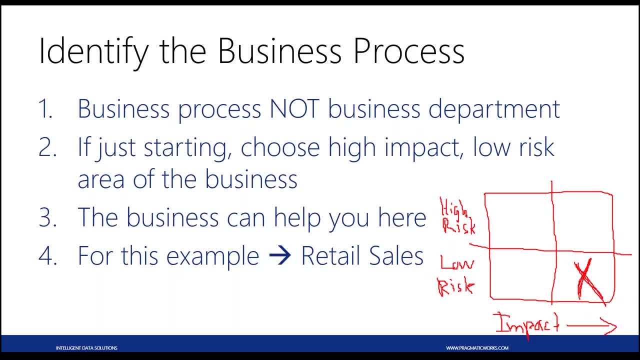 best way to decide what is the business process. we start with it first. if we've got people out there that are starting a data warehouse, scratch, how do they pick? what business process do we start with? it's a great question, so a lot of times what you're going to find out, especially when you're 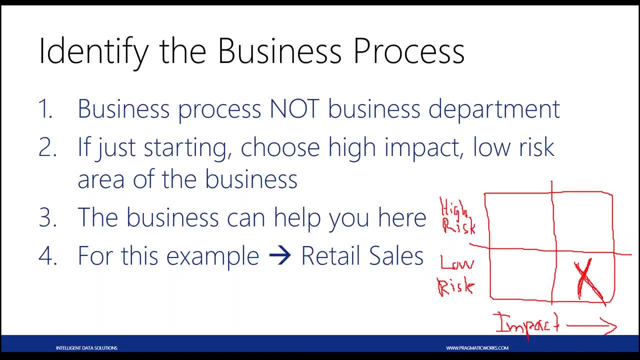 at a client, so chances are the business is already going to be telling you what those high-impact items are. if you're working in a BI environment now, then you probably have a user or a group of users that come to you on a regular basis and 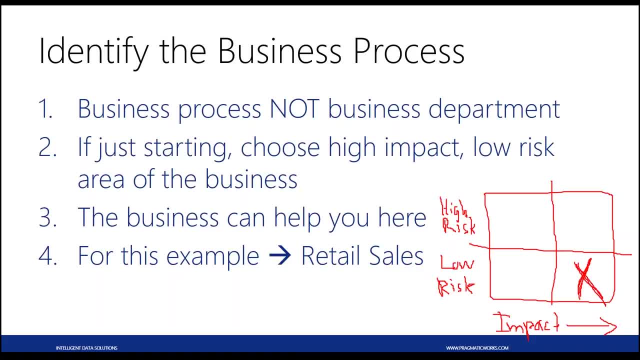 they say: can you send me that report again that shows me my profit margins by category? or hey, can you give me that report that shows me my freight that was delivered today? and what they're really asking me for what they're really telling me is that these are high-impact business processes. 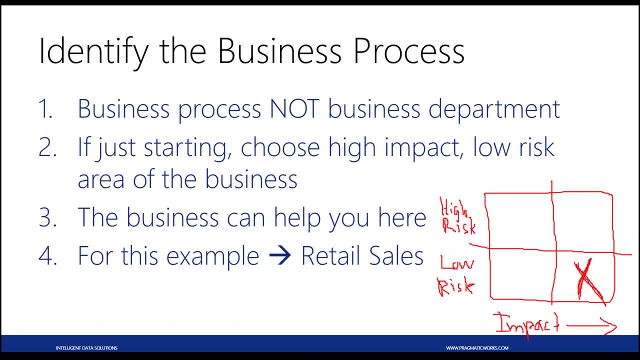 that I need a lot of visibility into. so chances are, if you don't have a data warehouse in your environment now, then you're probably going to have users that are already telling you that they need lots of visibility into these specific processes and they're high impact for the business. so a lot of times the 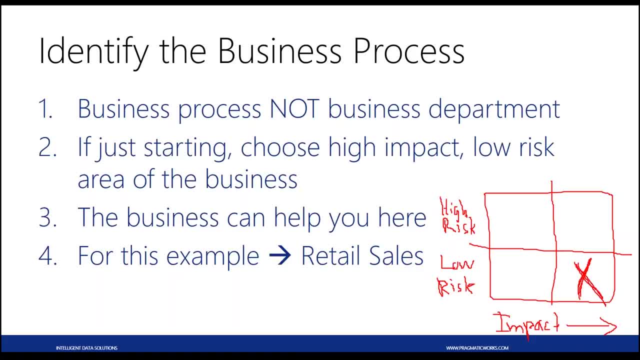 business is already going to have reports. they want that, they're asking you for, and it's going to be kind of obvious what you want there. now you're going to have to do a little bit of additional research to figure out. is this a high risk item or is this low risk? is the data going to be? 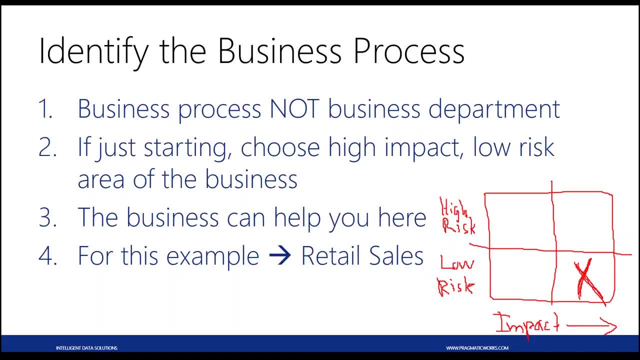 readily available? is it going to be dirty? data is, are we going to be able to get the business calculations and the business logic that we need? so that's going to have to take place as part of that process, and so that's good. another thing that we want to consider, Dustin, that we previously touched on, is that 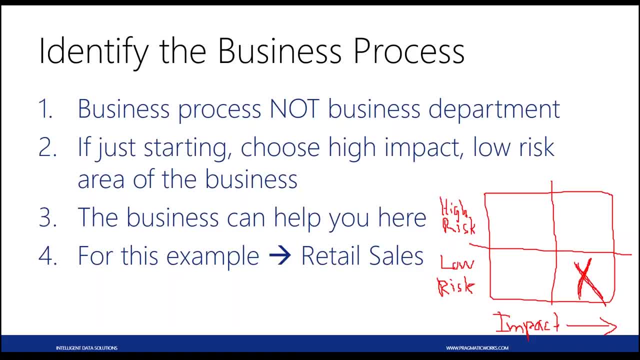 when we say identify the business process, we're talking about business processes for the company, not for an individual department in the company, and what we mean by that is you might have a retail data warehouse in your marketing department, and Marketing department is going to come to that meeting that Dustin was talking about with their own set of numbers. 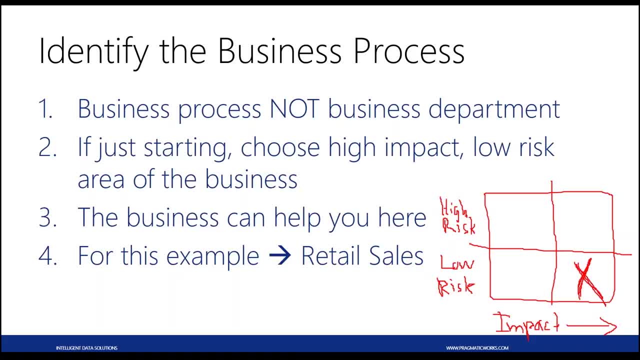 And then you have another retail data warehouse in your sales department and they come to that same meeting And they say, well, we've had this much in sales and marketing says, no, We've got this much in sales and we have conflicting numbers in our company. 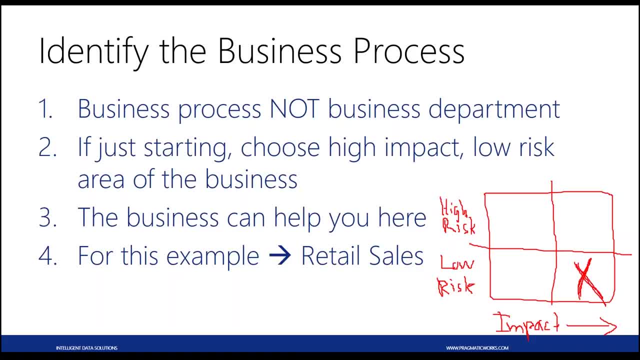 So we want to have one centralized data warehouse, one version of the truth from marketing, manufacturing, sales and retail. We want to have all that in one data warehouse. so that's something that we want to consider there. another way we might determine our business process is: 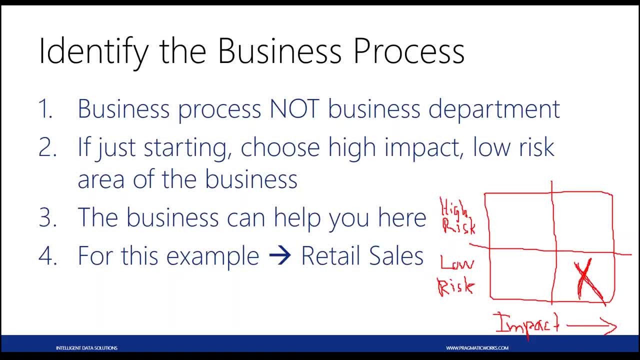 By listening to the questions that our business users are asking us. so a lot of times We're going to hear questions. They're going to say: what are the gross profit margins for our product categories for the previous month? What are? what's our average account balance? 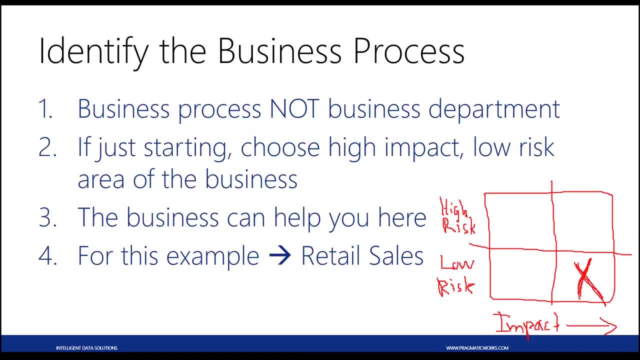 What is the average rental quantity? we're talking about block Buster, block, So what is our current rental quantity? and those are questions the business is going to ask us. and when they're asking us those questions, If we pay attention and we listen closely, Then we're going to know exactly what those business processes are that they're looking for, that are going to have high impact. 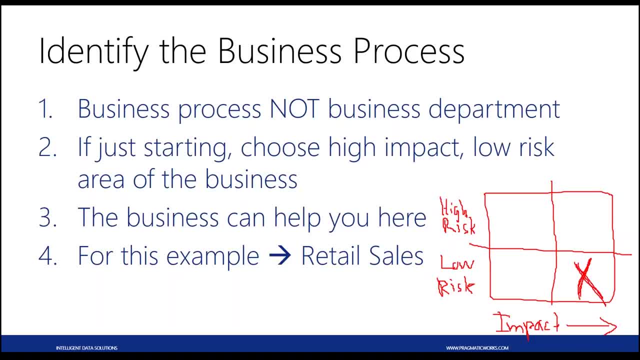 on the business Immediately, kind of that low-hanging fruit in the company, right? so if you've got, if you have, you know everybody's got that. one user that Always comes from says, hey, can you give me that report? Hey, I need that report again. 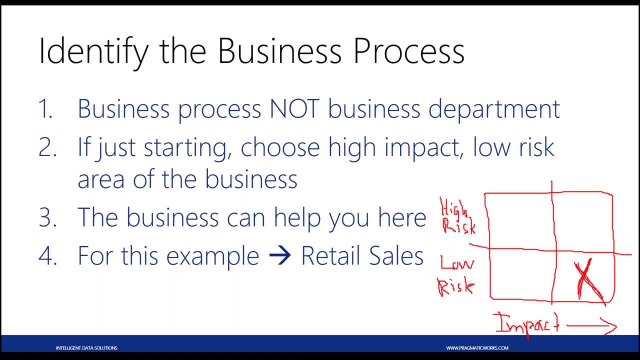 Hey, I need a report. you probably all have users like that. the ones that they're coming and asking me for the most are probably the Processes that have the most impact on the business, because they're the ones that that are going to know what's going to be high impact. 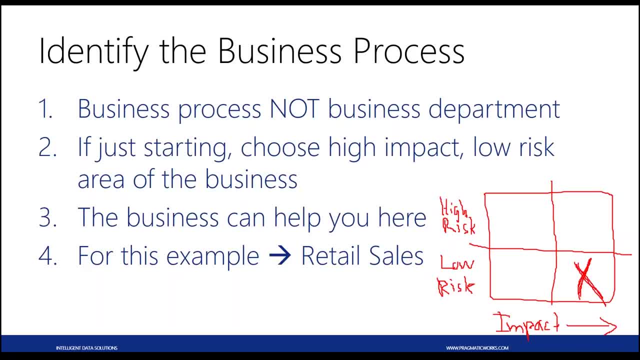 So what I hear you saying, Mitch, is: we want to look for that low-hanging fruit. We want to look for Those business processes that are going to have high impact for the business either: Make a lot of money for the business, save the business a lot of money, make the business more efficient. 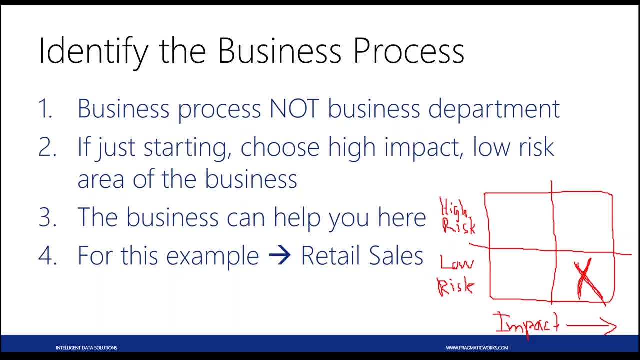 Whatever, but it's going to be low risk, We can get the data, We have people who can help us figure out the logic, those kinds of things, Absolutely exactly Okay. so in this case, We've already identified our business process. our example in this case is foster block right, our video rental store. 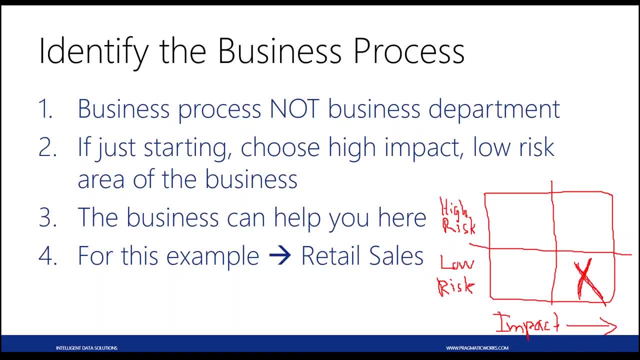 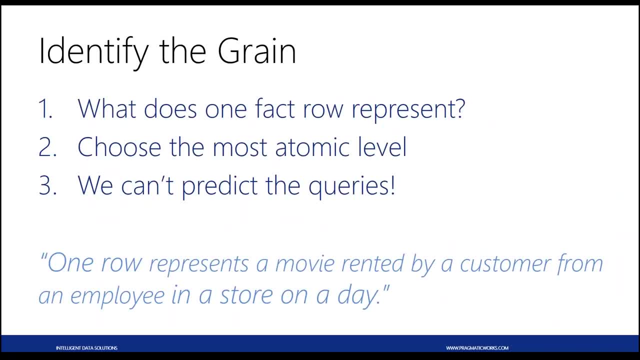 And so we're going kind of with a retail business process here for this example. Okay, so Now the next step here is: we want to be able to identify the grain of the fact table Now. this is the most important decision that you will make in your design process. 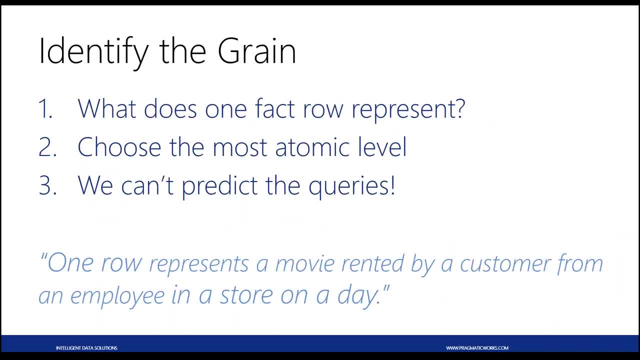 We need to identify what is going to be the grain in our fact table. Now, if you're new to data warehousing, you may not know what a fact table is. A fact table is a table that's going to be at the center of our star schema. 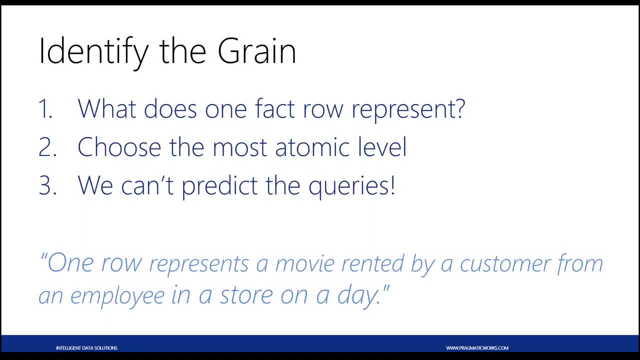 and it's the table that contains all of the facts about the business: how successful the business is, how many sales did we have, how much quantity do we move those types of things. So facts are measurements regarding the success or failure of the business. 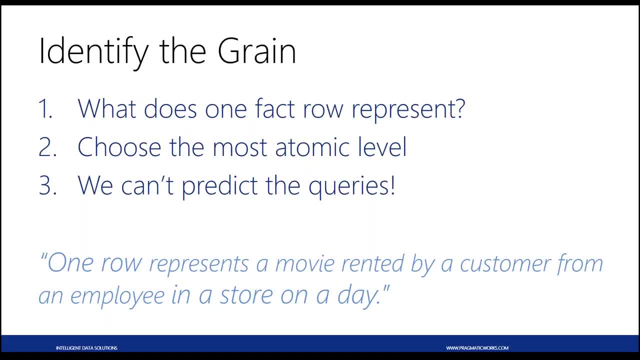 depending on what type of business process that we could be modeling. Now, when we identify the grain, we want to determine: what does one row in the fact table represent? Okay, so if we're working in something, There's some type of retail scenario here where we want to identify, you know. 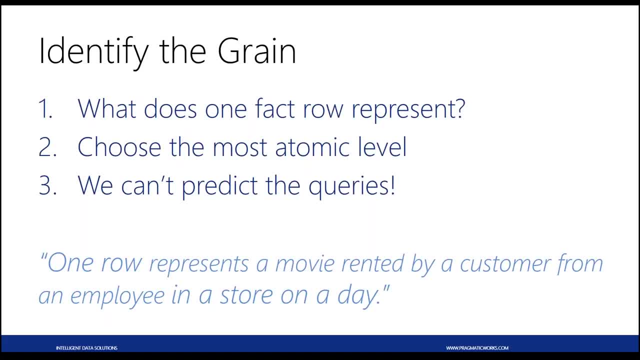 what does one row in our sales fact table represent? In the case of Buster Block, it might be a line item in a transaction. So for this business process, we're going to decide. you know what One row in this fact table represents: a line item in a single transaction. 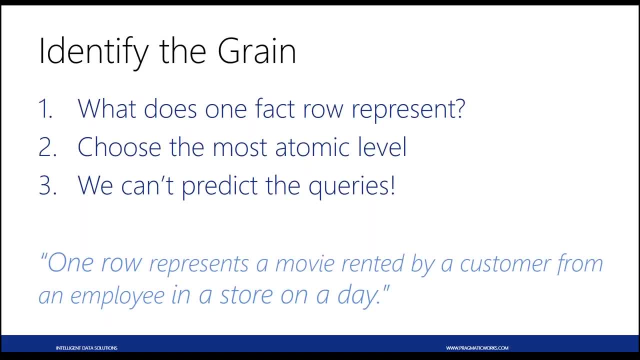 So that could be an example in a retail scenario and that's what we're going to go with for this example. Now, if you're working, If you're working in some type of you know business process where you want to track inventory, 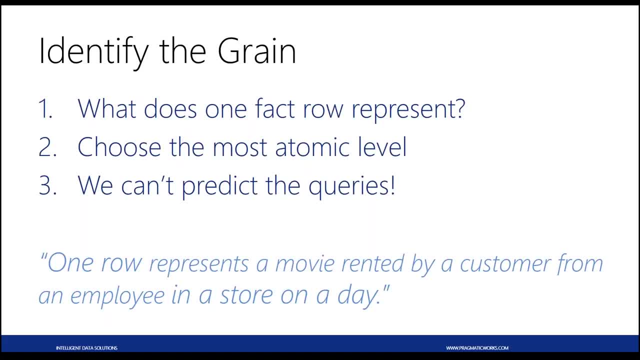 maybe you're deciding that you know what One row in this fact table represents a record of inventory on a particular day. So every day we go out to our data warehouse, we figure out Or not our data warehouse, our physical warehouse, and we determine: okay, we've got. you know what. 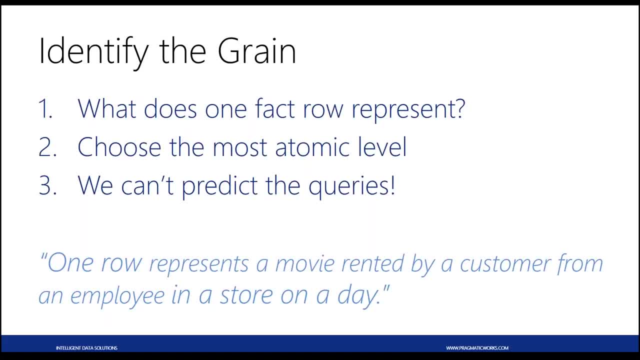 We've got 500 cheese balls sitting on the shelf. We've got you know a thousand boxes of cereal or we've got you know whatever is in our warehouse and we want to log that every day. We want to log that every day into our fact table, so maybe in an inventory example. 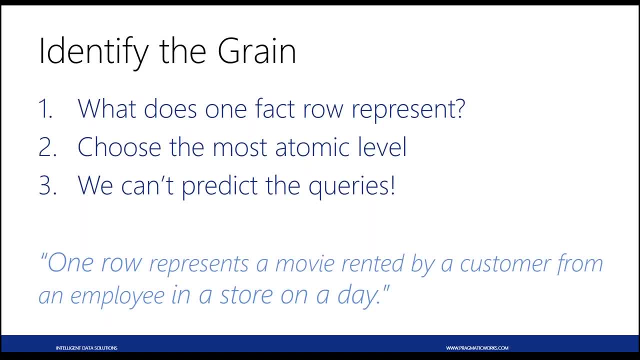 one row would represent a- you know, a record of inventory on a given day. But when you determine what one row represents in your fact table, it's important to go with the most granular level. You want to design your dimensional model to support the most atomic or granular level that you have with your data. 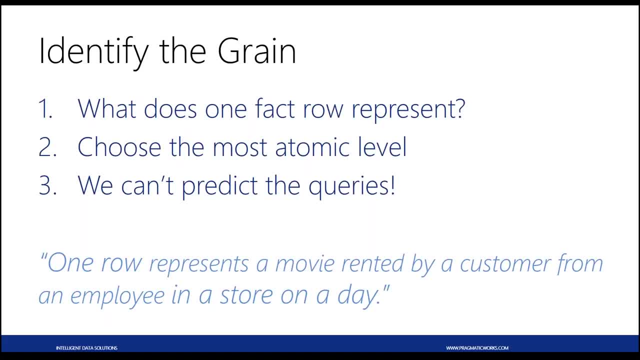 Now, when we're talking about Atomic- the most atomic level- we're talking about data that cannot be subdivided anymore. We can't break it down anymore. This is as low as the data goes. We can't subdivide this anymore, and the reason we do this is because data that is at the most atomic level can be rolled up. 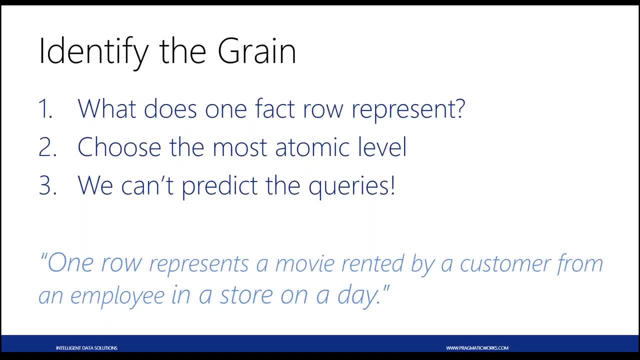 it can be aggregated, it can be sliced, it can be diced and pretty much any way that the users want. okay, And this is really good for ad hoc queries, because the bottom line, The bottom line here is that we can't predict how the users are going to query the data warehouse. 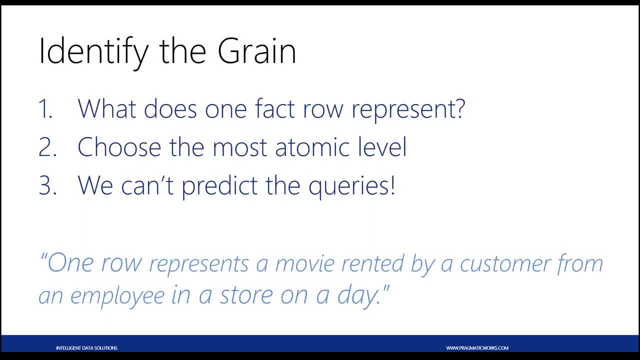 They might tell us that, look, we want a report that does XYZ or shows XYZ, right. But the moment they realize that, okay, well, we can ask other questions of the data warehouse, or we can ask other questions of the cube, they're going to start firing all kinds of other queries. 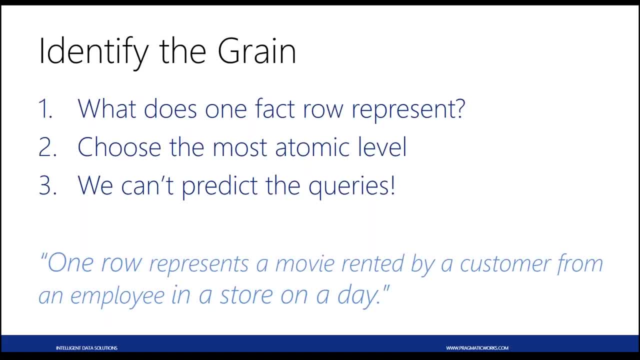 They're going to connect to the cube with Excel. They're going to slice and dice in ways that you didn't really expect, and so that's one of the reasons that we want to store this low data at the at the most atomic level. 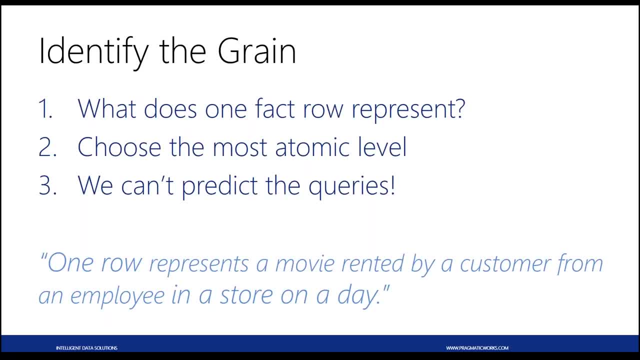 If we decide. you know what you know. I've worked in situations where a client said we really only want the data at the month level, We don't care about it at the day level. You usually still always want to go with a granular level because eventually they're going to ask you. 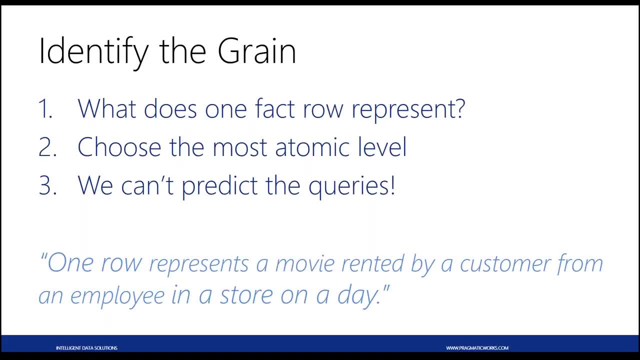 hey, can we look at this? what happened? you know, we see an anomaly at the month level, right, And so, okay, well, we want to figure out where this happened at. Well, we can't right, Because we've aggregated. 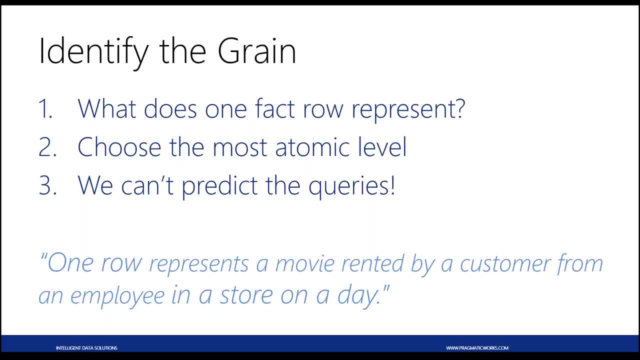 We've aggregated our data warehouse up to the month level, so we can't roll it down, and so that's always something to be aware of. So I've got a question for you: How much work would it take to rework that? 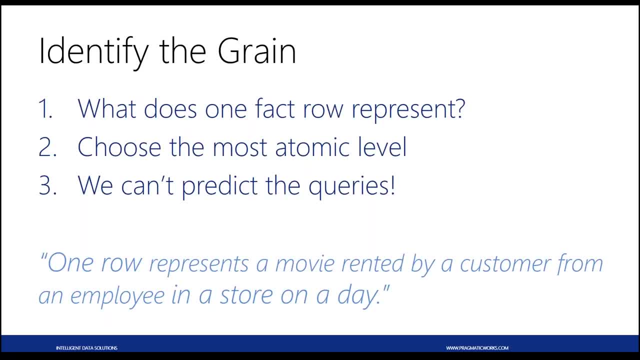 I mean, if you build your entire data warehouse on a monthly level, or maybe a weekly level or a daily level and you want to go more granular, how much work would that take? I mean if you've designed your whole data warehouse to be at the day level, or I mean at the month level. 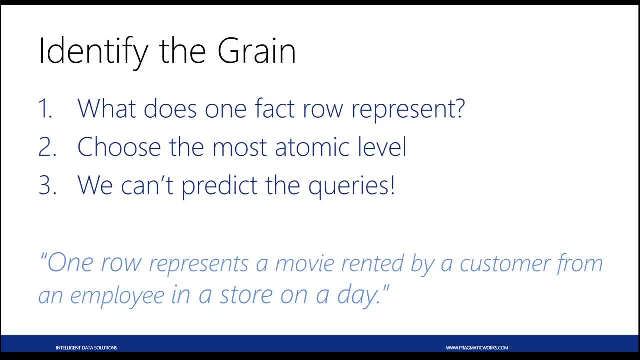 and then later on down the road, you know what. we want to take this fact table and we want to roll it. We really want to change it to the day level. If you don't have that history somewhere else, you know what we're going to have: to change it to the day level. 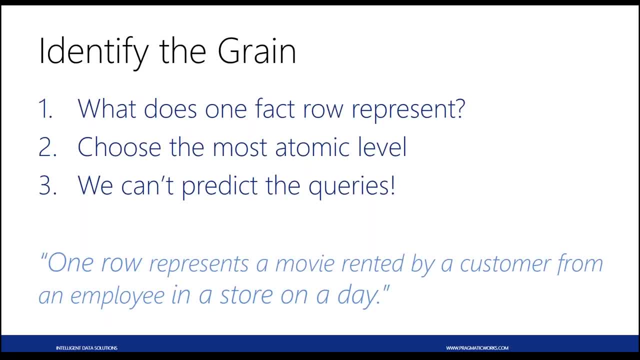 If you don't have that history somewhere else, you're not going to be able to get it Okay. so that's a problem for one. But if you can, it's going to be a lot of work because then you're going to have to rework the fact table. 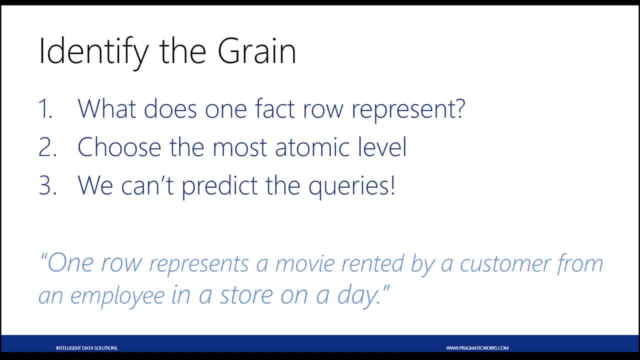 You're going to have to rework dimensions. You're going to have to rework ETL. You're going to have to do a lot of rework there. So that's kind of why I said at the start of this that you want to focus on getting this step right. 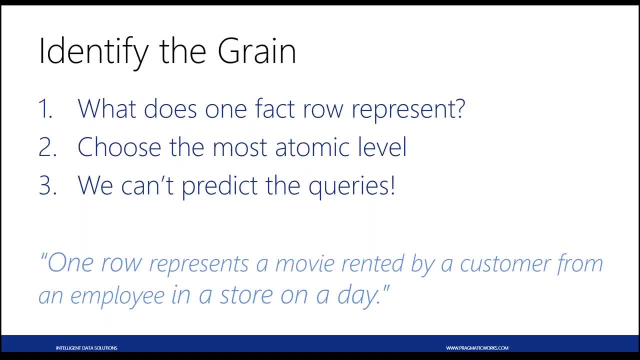 because if you mess this step up, it's going to cause problems for you later on down the road. Okay, so the bottom line here is: we can't predict What queries the users are going to run against our data warehouse, So we want to store it at the most granular level so that way they can ask any questions they want. 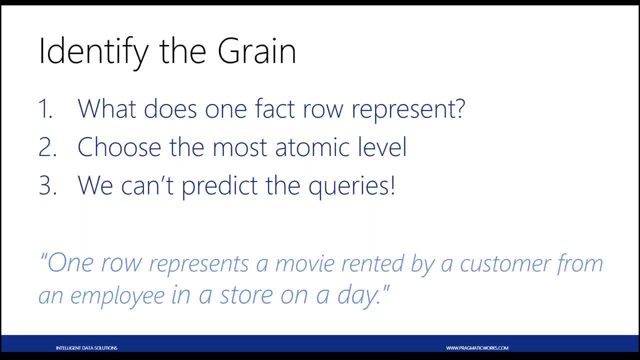 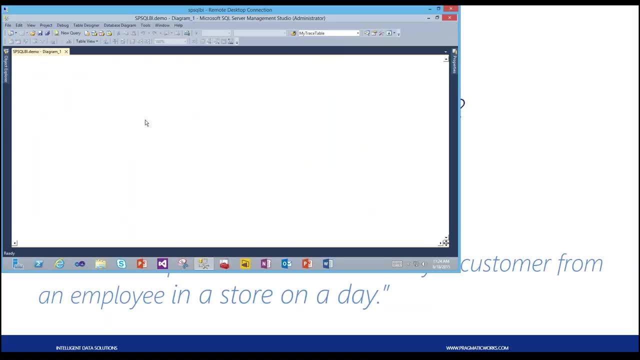 All right, so in this particular case, let me bring my virtual machine over here so we can kind of do this together here. All right, so we're going to stub out here a data warehouse design together, And so what was our brain statement? 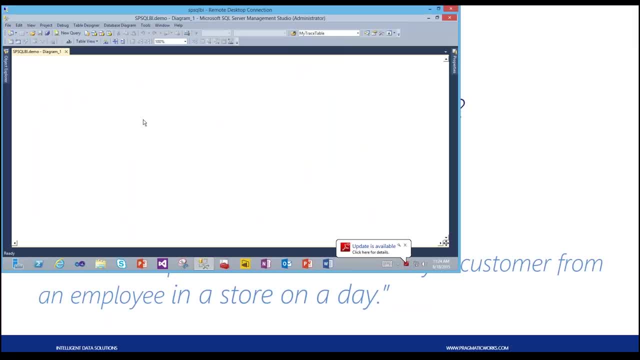 One row represents a line item in a transaction at a BusterBlox store. Okay, and so we're going to start here with a new table and we're going to call this fact sales, because we're going to give it the fact moniker, because this is a table that is going to contain our fact data. 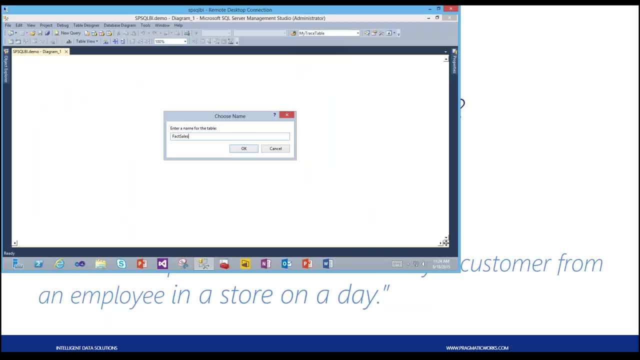 those measurements that the business has identified that they can use to tell how much success they're having in the execution of the business. Okay, oops, I already created that one, So we'll call it fact video sales. How about that? Okay? 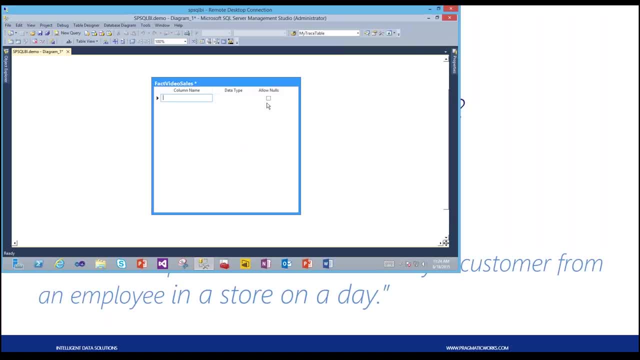 All right, and so when we determine the grain of our fact table, based on that grain we can determine what kinds of dimensions- which we're going to move into here in a minute- we can determine which kinds of dimensions that are going to be related to this fact. 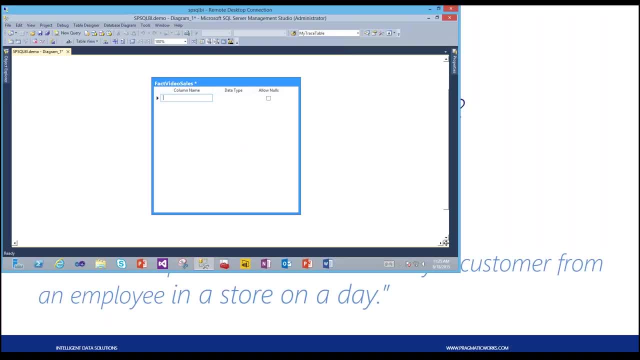 So if we know it's a line item on a transaction in a store, so we know that there's going to be a product related to this right. Somebody's renting a movie. Maybe they're renting you know a movie, You know? Gone with the Wind, Dances with the Wolf, Saving Private Ryan in Mitch's case. all about miniature trains. 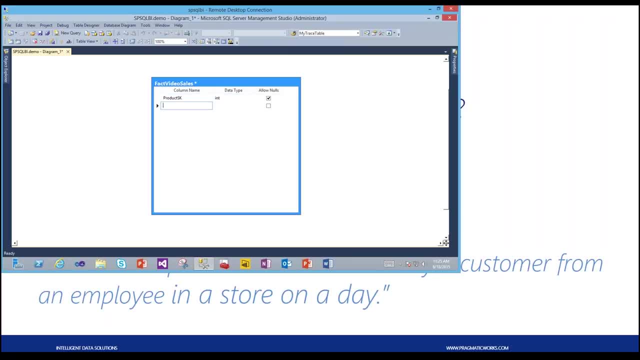 So we know that we're going to have a product dimension that's going to be related to this. We also know that a transaction is going to occur on a given day, right? So we know that there's going to be a date associated with this. 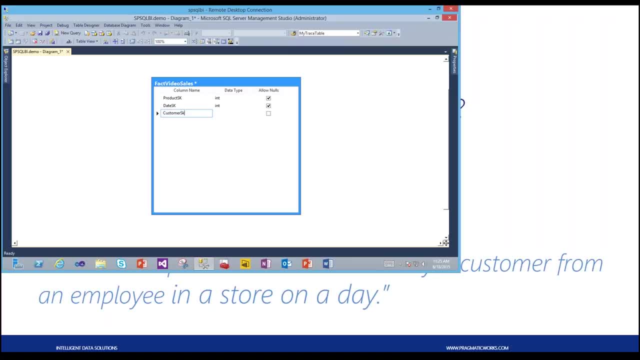 And a customer is going to be associated with the transaction, so that we know we're going to have a customer, Okay, And we're going to discuss what an SK is here in a second. And then also, we've got product, we've got date, we've got customer, and what was the other one we said we were going to do? 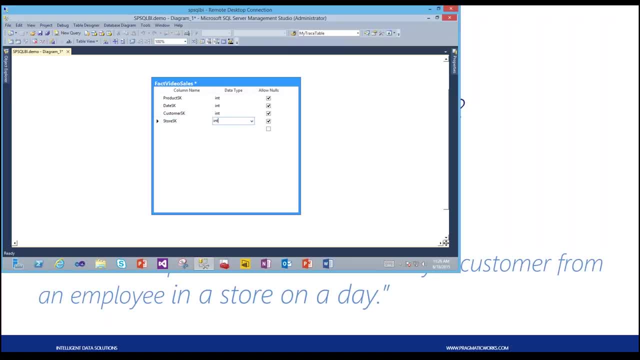 And we've got store right. This is going to be happening in a store, Okay. And so this fact table here kind of embodies what our grain is right. This is a transaction that's occurring with a product on a day, with a customer at a store. 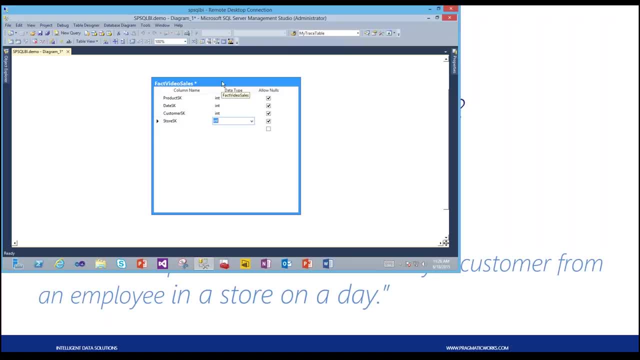 And so, based on this, we can do analysis on how many products are we going to sell. How many products did we sell in a store last month? How many products did we sell on this day? How many products are bought by our top 10% of customers? 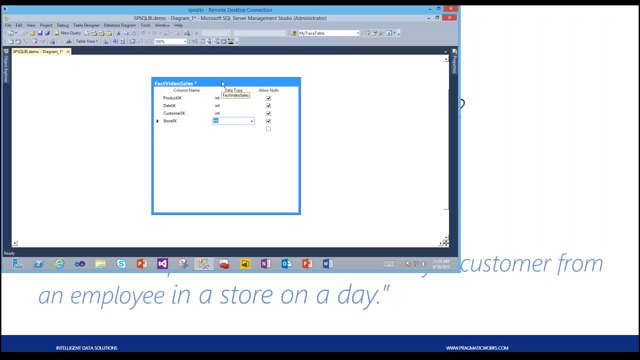 How many products are our store selling by store? So we can do all kinds of different analysis based on this particular grain. So now that we've kind of identified what is going to be the grain of our business process that we're modeling here, Now it's time to move into identifying. 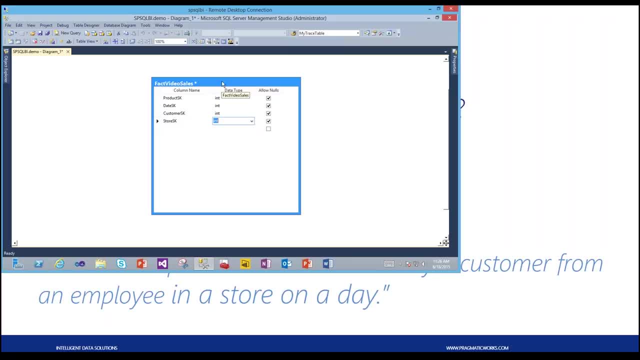 The dimensions. what are the dimensions that are going to be related to this particular grain? All right, thank you, Dustin. So what is a dimension? A dimension is going to contain descriptive information regarding our data. If I told you that we had $5 million in sales, you're probably going to have some questions. 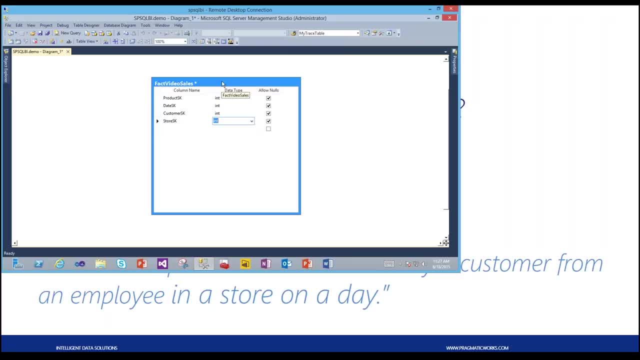 about that. You might be excited that we have $5 million in sales, but it's not very descriptive. It doesn't tell you anything about our data. So what we want to do with our dimensions, we want our dimensions to answer those questions. 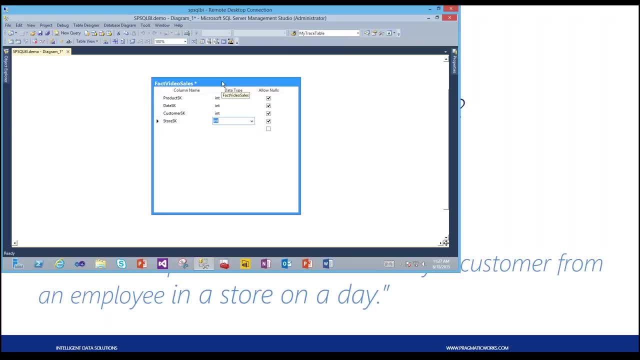 that we might have Questions like: what is the breakdown? What is the breakdown by product category? Which one of our stores had the highest amount of sales? How much did we sell last month? And we can break that information down by using those dimensions. 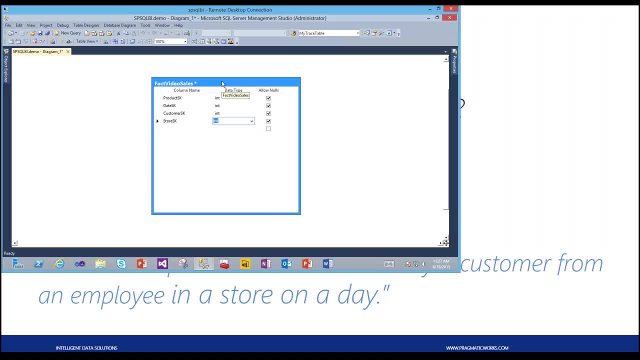 Now, these are questions that we answer with dimensions and, if you've correctly identified the grain, this step is actually going to be very easy, as Dustin just showed you. The related dimensions will be easily identified. For instance, our grain statement, once again, is going to be: one row represents a line item. 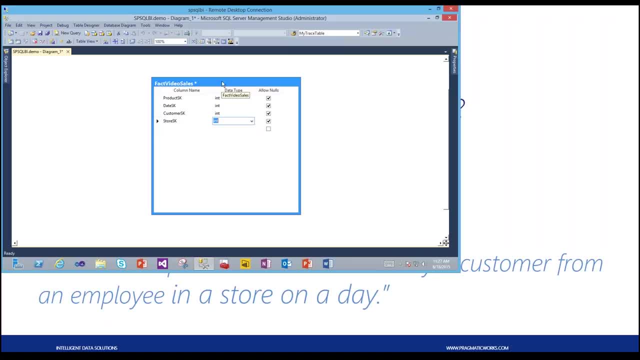 on a transaction. We know the transaction had a product that was rented. we know there was a customer involved. we know that it happened on a specific date and at a specific store, So the grain is very important And everything else that we're going to do in this section is going to be related to. 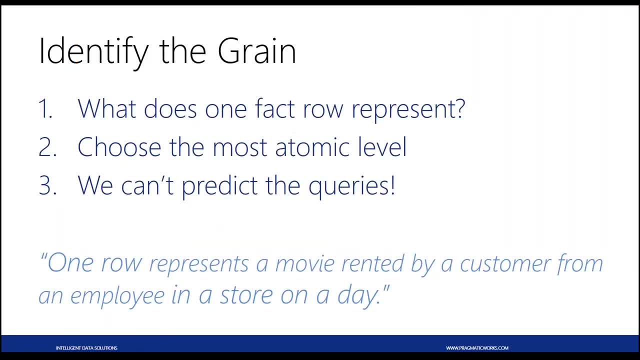 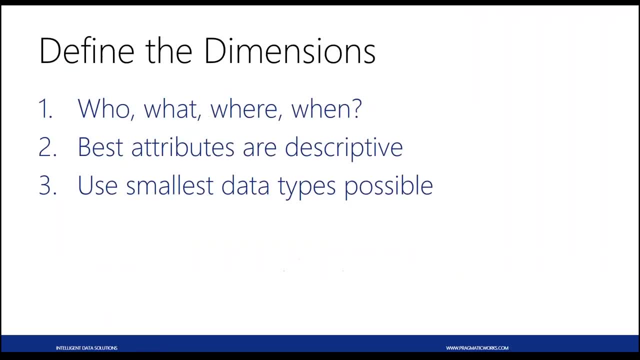 that. So we're going to be looking at the grain statement and actually working through this data warehouse. However, if you're going through this and you identify a dimension, if you're looking at your grain statement and you identify a dimension that is not correctly represented, 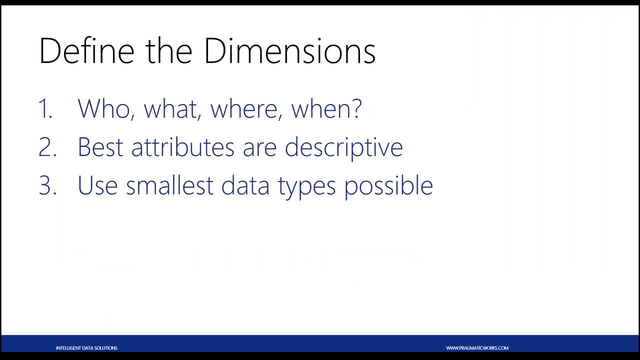 in our grain statement, then step two in the process identifying the grain must be revisited. We have to go back to step two. So, Dustin, this is actually a good little segue here to ask you: do you see any chance that our granularity identified can actually be subdivided further? 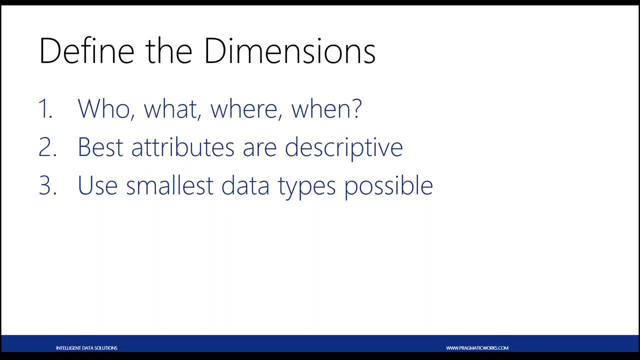 Because it's pretty low right now. Yeah, that's a good question And it's something that we're looking at. It's something that you have to take into consideration as you're going through the design of your data warehouse. So, in this particular case, we've determined that one row in our fact table represents. 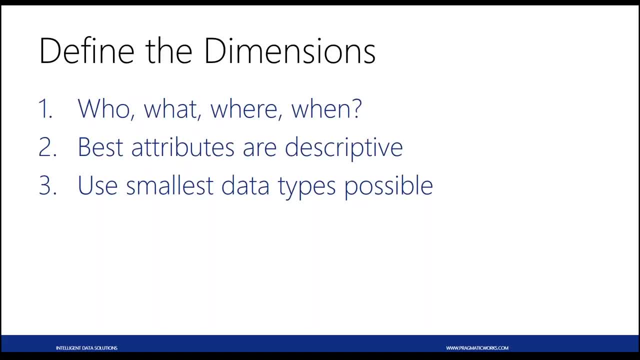 a line item on a transaction, right. But if we get into identifying the dimensions and our business users come to us and say, hey, we want to be able to tie a particular transaction to a special that's going on a coupon that the customer used, what is some kind of promotion? whatever might be going. 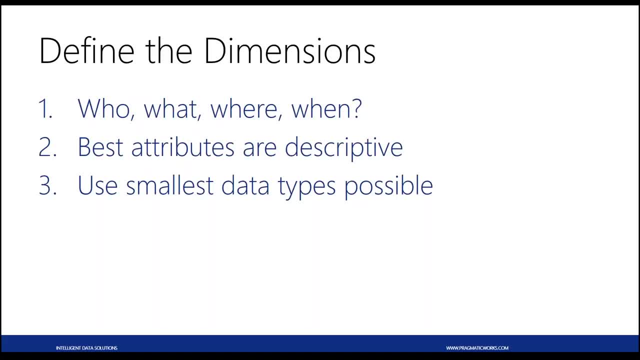 on in the business, So that way we can analyze a promotion effectiveness. Now, if we do that and say, okay, well a customer could. there could be one promotion or more than one promotion associated with a single transaction. So maybe there was a deal going on: rent one movie, get one free, kind of thing. 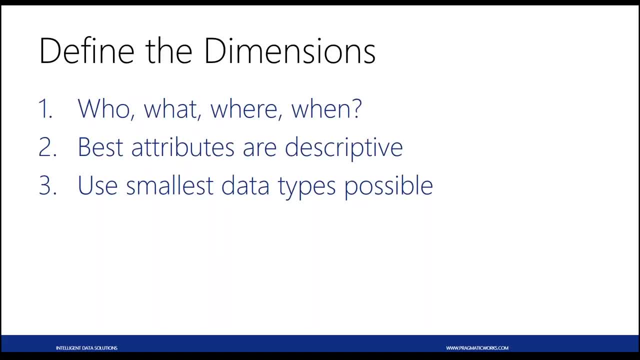 But they also had a coupon for a bag of Skittles or something like that. So you've got a customer using a coupon and then you've also got a store promotion going on, And so each of those promotions has an effect on that sale. 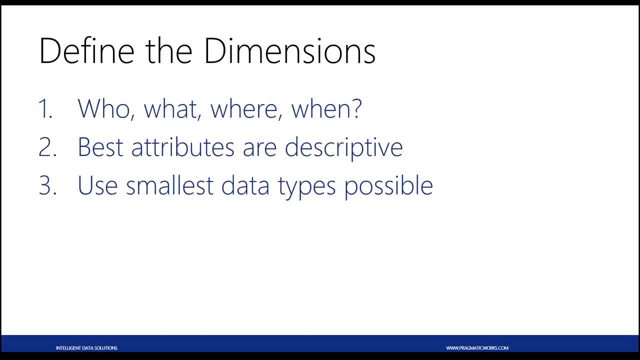 And so we may determine that you know what the grain of this fact table isn't really one line item, it's a coupon. one coupon per line item, So we could have multiple coupons associated with a line item. So if that kind of happens, where you decide that you know what the grain of our fact, 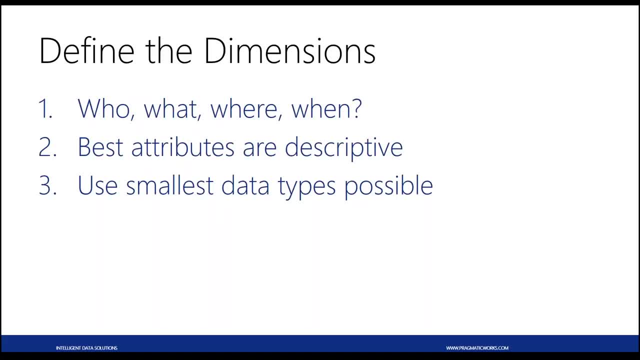 table is not correct, we've got to go back and revisit this. then it's important that at this stage you go back to step two, because we've got to get the grain nailed down. This is the most important step because, like I said earlier, if you mess up the grain, 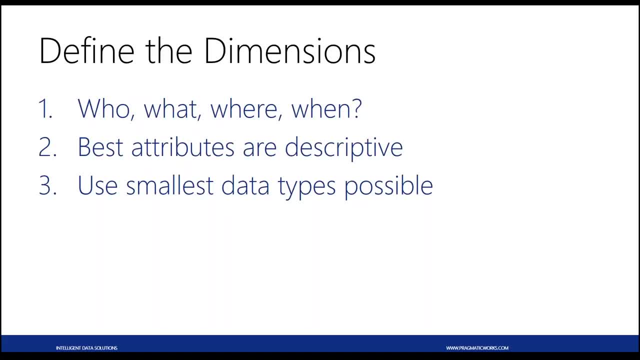 and you find that out later, it's going to cause a lot of rework. So if you get to identifying the dimensions, or if we get to step four, identifying the measures, and you determine that you know what our grain statement is, not completely. 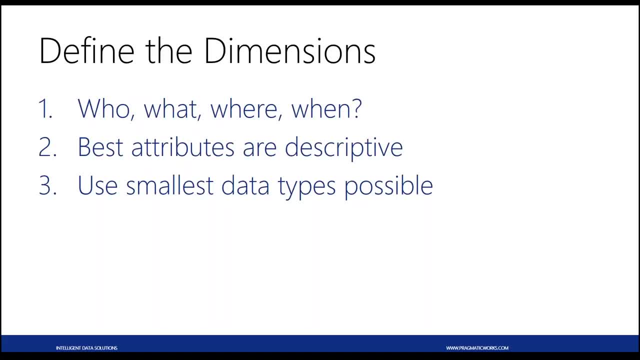 correct. we need to go back to step two and revisit that So that way we can get that correctly, because this is really going to lay the foundation work for the rest of the data warehouse and the cube as well. This is going to play an impact on the cube. 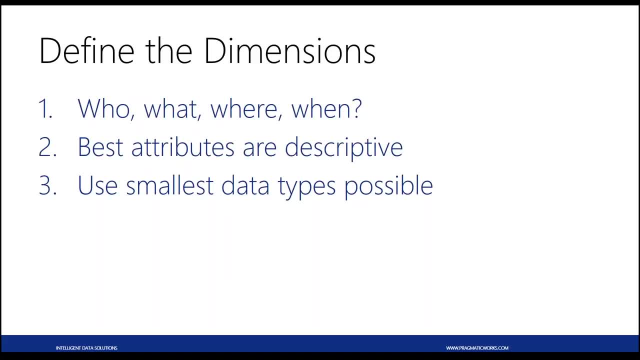 So if you find out you've done the grain wrong- and you're already done the grain wrong, you're already into the cube part of it- then you've really got a lot of work to do. All right, good job. Thank you, Dustin. 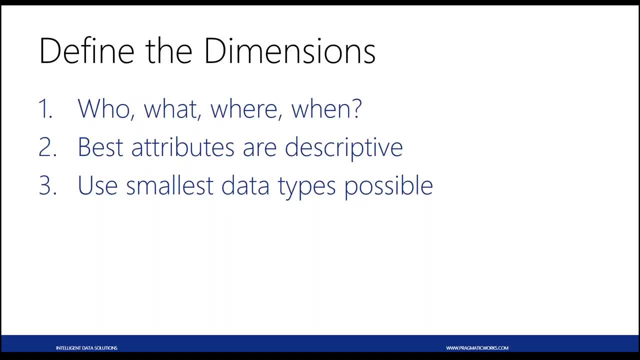 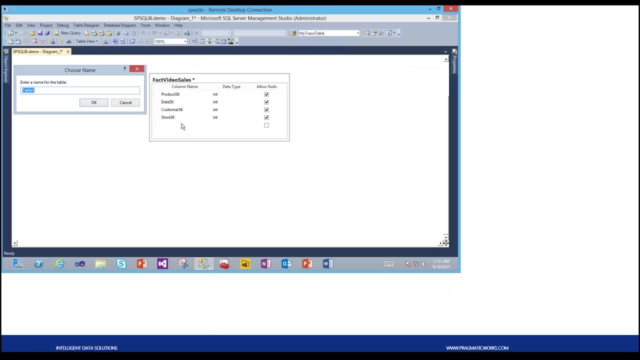 All right, we actually have a couple questions here. A lot of people in the webinar noticed that we did not add the employee dimension, and they're letting us know about that. So if you want to throw that in there, you can. And then also the next thing that we had a lot of questions on is what is a surrogate? 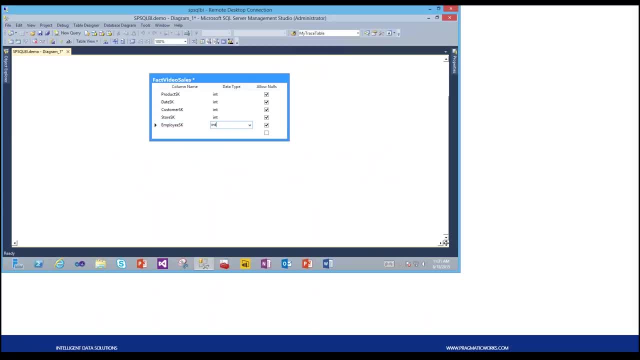 key. So I'm coming to that point in just a second Man. it's like they're reading your mind. I know they're ahead of me here. We've got to talk faster, Okay, So in my product dimension, the first thing we're going to do here in this dimension, 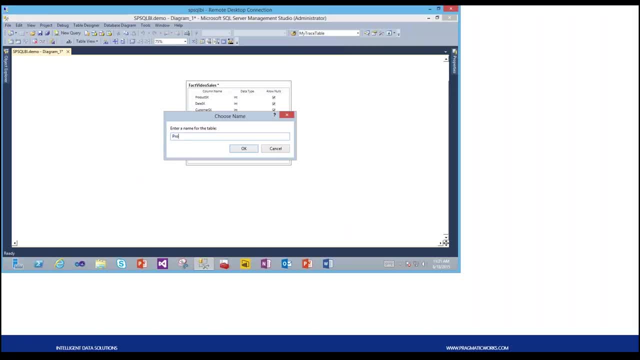 is we're going to add a database Key for the table. The database key is an identity key on the column and this is called a surrogate key. This is going to help us with modeling the relationships between the dimensions and the fact tables. 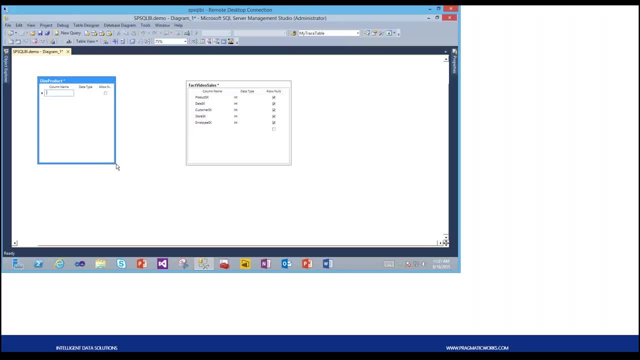 Now, the reason we don't use the business key is if we use the business key, then we're going to be vulnerable to things like source changes in the transactional system, And that might not mean a whole lot to you right now and we don't have time to get deep. 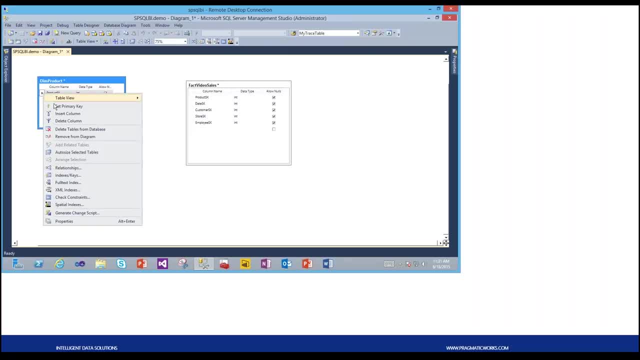 into detail on that. But if something changes in your source system, like a metadata change, the data type of that changes. It's going to affect all the relationships between your dimensions and your fact tables. So we want to insulate ourselves from those kind of changes. 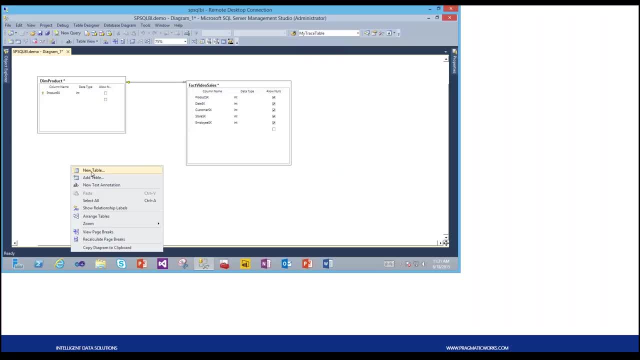 And that's what the surrogate key is going to give us. So, as we import data out of the transactional system and into our data warehouse, if there are any changes in the sources, that could definitely cause a lot of problems for us. So, aside from just insulating ourselves from any of those issues in our source system with 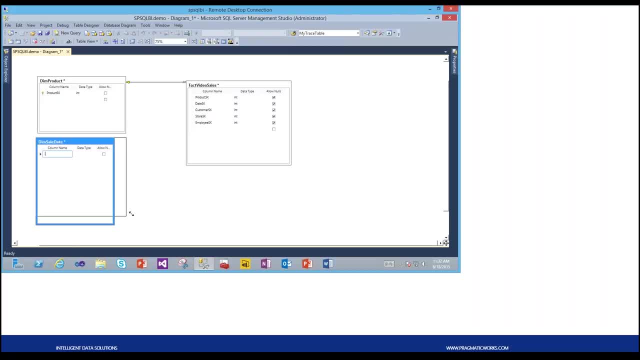 our data warehouse. we're also going to create a database key. Okay, I'm sorry, We're going to go ahead and create our product key or our product ID on our product dimension as well. I'll let Dustin kind of catch up here. 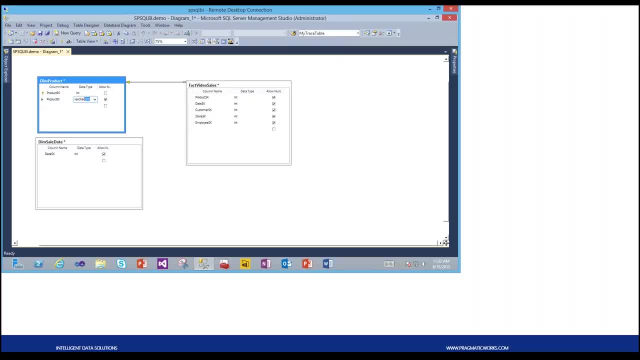 So the product ID is going to be the business key. We just moved from our surrogate key, which is that primary key in our data warehouse, but that business key that's critical to our business is going to be the product ID. The product ID is going to be how we can essentially go from our data warehouse back to the transactional. 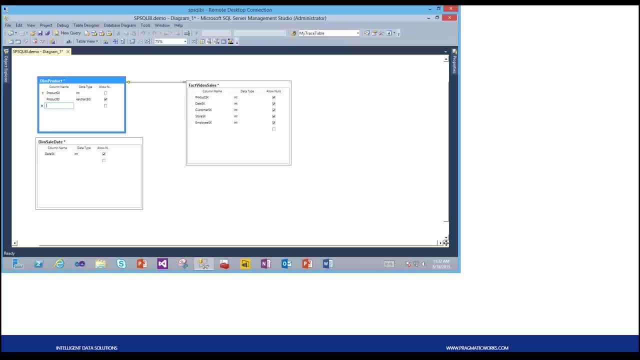 system and we can kind of track and trace exactly where that product came from and we can see exactly what that product is, any of the transactions around that product. So the business key relates back to the transactional system, but that surrogate key does not. 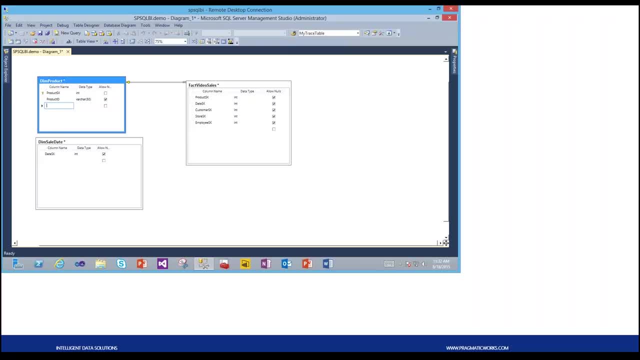 That unique identifier in our data warehouse does not relate back to the transactional system, And there's also a couple other reasons why we want to have that surrogate key other than just insulating ourselves from changes in the source system. One good example is it's going to actually optimize the joins in our fact tables and 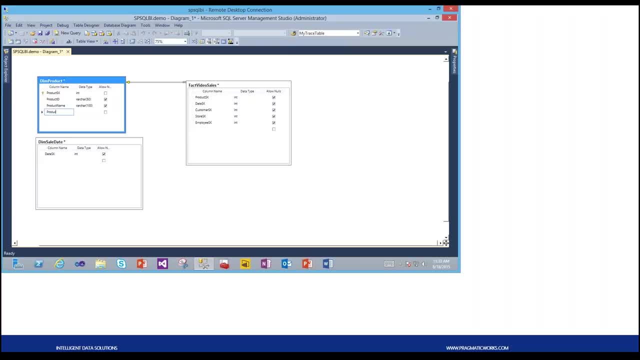 our dimensions. So now we're going to be joining our fact tables and our dimensions. We're going to be doing that on single integer columns, on these simple integer columns, instead of strings or any of those other data types, which is going to simplify our model and improve. 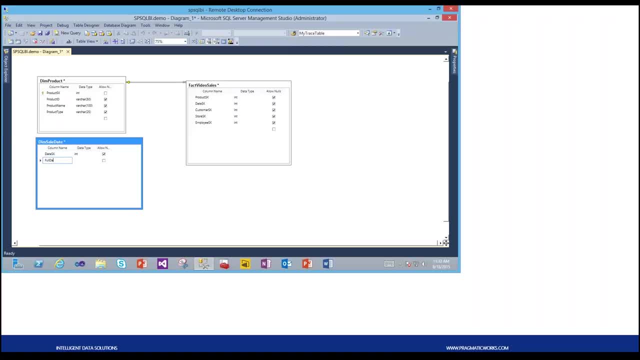 our join conditions. Surrogate keys are also going to allow us to keep historical information in our dimensions over time. So if you're building a very robust data warehouse and you want to be able to track cells- when you were selling a product at $5 and when you were selling a product at $6, and how- 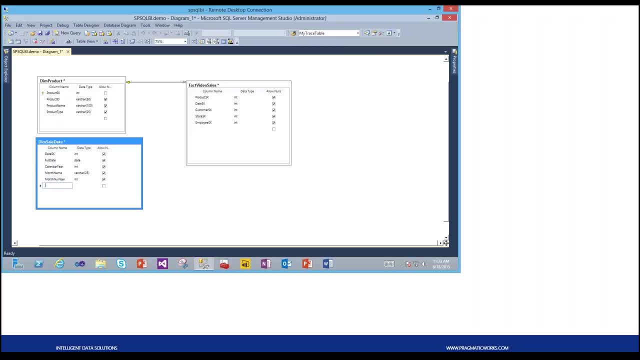 much did we sell? Did sales increase or did they decrease? We can keep that kind of information in our data warehouse By keeping a history of the price that we sold that item at or that we rented those rentals at. So that's what surrogate keys give us. 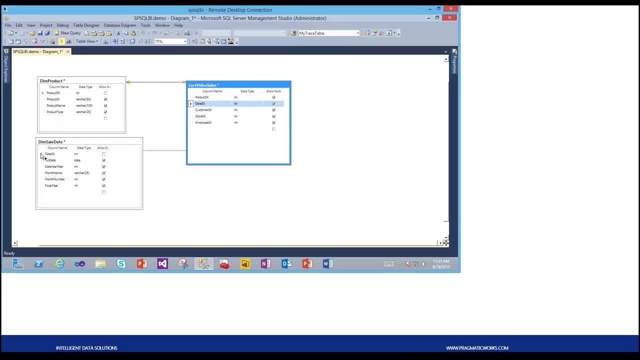 We can't build a slowly changing dimension that changes over time using business keys. The other reason that we might want to use or not use the business key is that we might have two different departments in our business that have different product IDs for the same product. 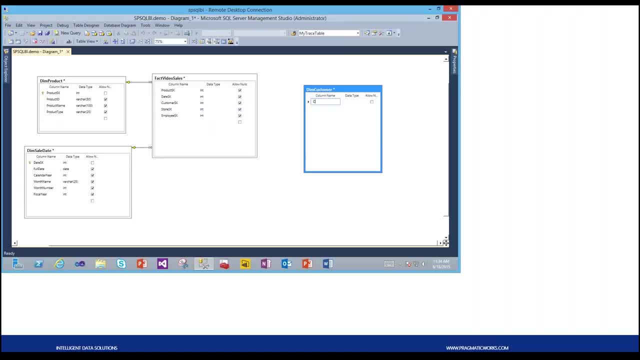 So you might have marketing that simply calls all baseball bats, just baseball bats, but then our manufacturing department might have a product ID that simply calls baseball bats. So you might have marketing that simply calls all baseball bats, just baseball bats, but then our manufacturing department might call all baseball bats. 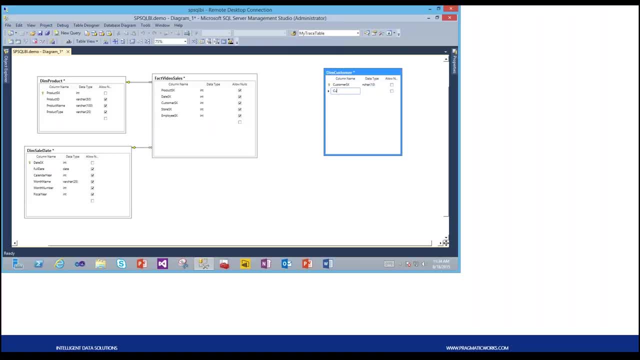 So if you are a marketing department, you might use a product ID like ABC 123. Those IDs don't necessarily relate between those two departments, but by creating that surrogate key now we can have that one consistency in our data warehouse. Those are three other reasons why you might want to ask for a service key, or this should. 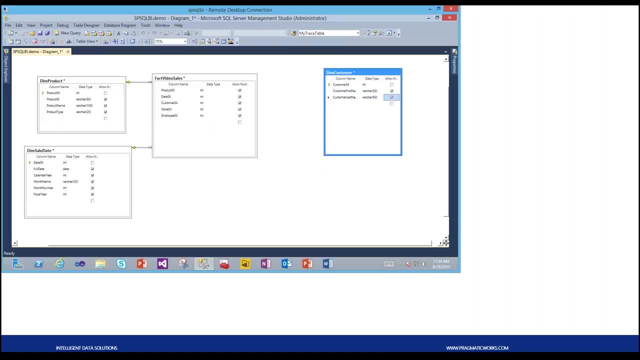 absolutely have surrogate keys in your warehouse, So Dustin is going to tell me about your dimensional model right here on the board. so in our product let's see what we have. here We have Product ID, changing the name of a product. this a little bit simpler for a one-hour webinar. we're not putting everything in. 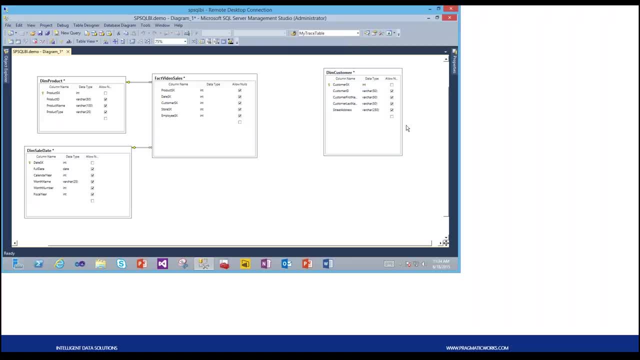 there. but just imagine what else you could have in your product dimension. you might have product size. you might have the date that you started selling the product. you might have the list price of the product. how much do we sell this product for? these are all things that we can track over time. that's related to: 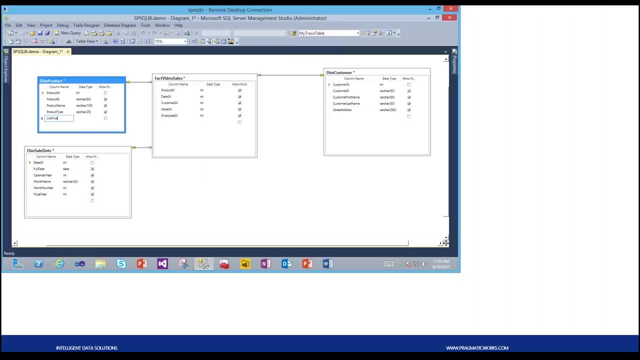 our product. that's a good one. list price, this price, especially for historical, slowly changing dimensions. right, I'm going to track over time. I see you have the sell date, you have the customer. are we going to put the store in here? yep, in there, all right, all right. so in the customer dimension, we have our 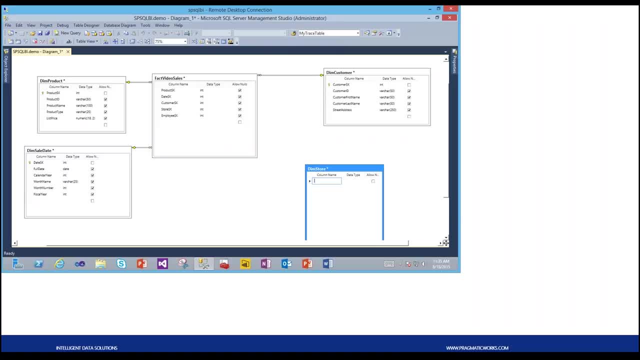 customer first name. customer last name. the address is very important. where are our rentals coming from? what zip code are we getting our rentals from and we can break that down. that can be information that we give to our marketing department. that's very important. we might do some other things. 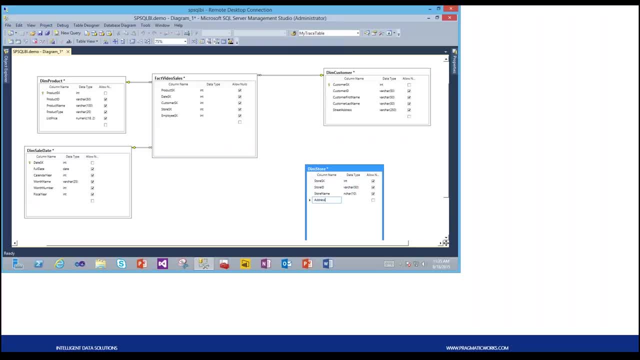 in customer as well, though right, we might do. gender, we might want to know if they're married or not, we might want to know their date of birth, so we can kind of get a an age of our average customer and the genres that they might be coming in there and and 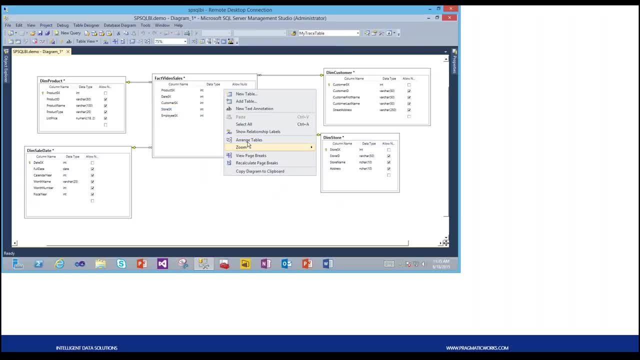 renting from us. so that would be very good information to have all right. and now you've thrown the store in there. so in the store, we're going to have some good information in there as well. we're going to have the store name, we're going to have the store address, we're probably going to have some stuff like maybe the 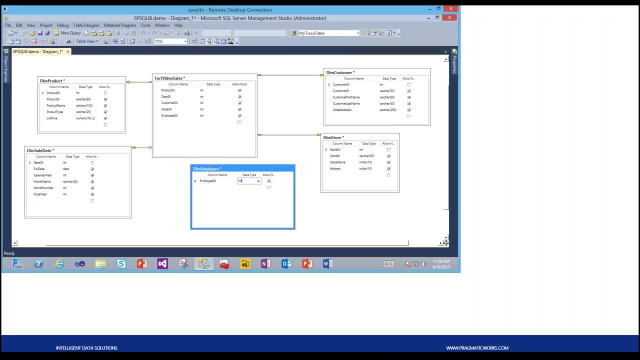 store manager. now, as you get into a little bit more advanced data warehousing concepts, you might break the store manager out into a separate table, but we want to keep this as close to a star scheme as we can. so you can- you can- add the store manager in there, absolutely, and dustin's also going to add the. 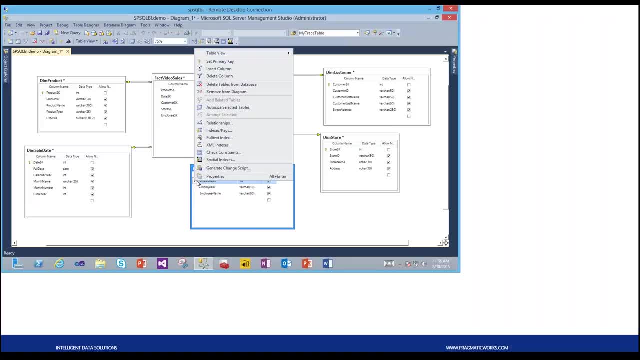 employee dimension. now, I was actually interested in the date dimension that you added over here. Dustin, you got some. we could add a holiday in there, right, the information would be pretty interesting. yeah, exactly now. one thing that I mentioned here with the attribute selection is that the best kinds of attributes that you're going to have in 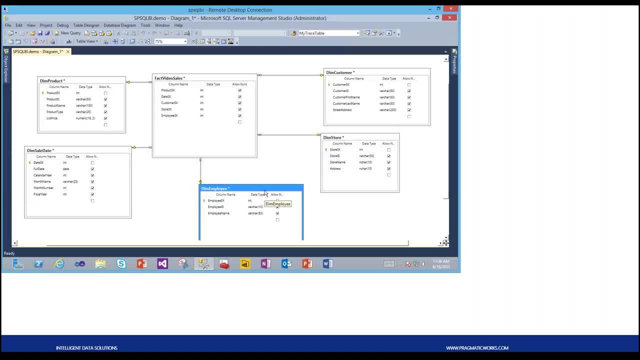 your data warehouse are going to be those attributes that are most descriptive, right? so what you don't want to happen is you don't want to have a dimension like store- right? that, only that is just full of IDs, right? so you've got like the store ID, maybe you've got the the you know geography ID, or you've got like all. 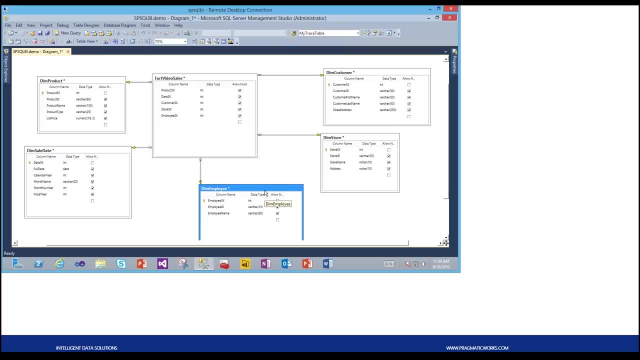 these different types of IDs, that are just all these integer values. so the best kinds of attributes are going to be very descriptive types of attributes that the users can look at and they don't have to ask a lot of questions about that. what you don't want is you don't want your user to have have to. 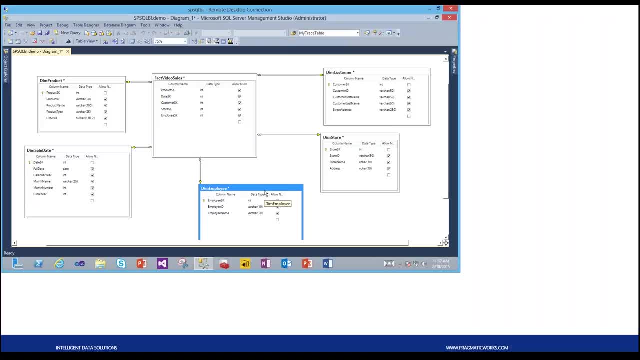 have sticky notes all over his monitor because he's trying to figure out. okay, store ID number 12 is the one that I've been watching lately, so I need to have that written down somewhere so you want them to be able to look at the attributes and to have a very clear understanding of you know what the data. 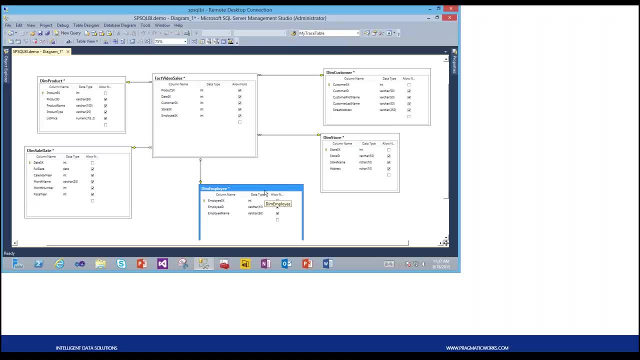 is what it, what is what's included in there, and they don't have to come to you with a lot of questions about asking you know, what does this mean? right, you want it to be kind of intuitive from that kind of standpoint. now I want to point. 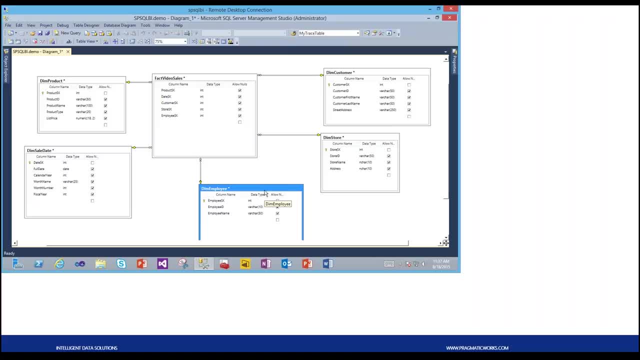 out now that we've kind of we've identified, you know, we've kind of we've identified our dimensions here based on our grain statement right, and so we've determined that on at a transaction item level, we can, we can, we can basically understand: there's a product associated with that, there's a date associated with the sale. 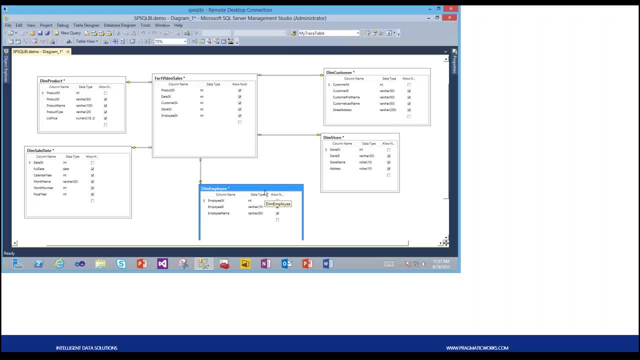 an employee. you know, work with the sale would work with a customer on that sale. that happened in a store and a customer bought that product right. so we've- we've been able to identify our dimensions there and I want to point out a few things to be aware of. 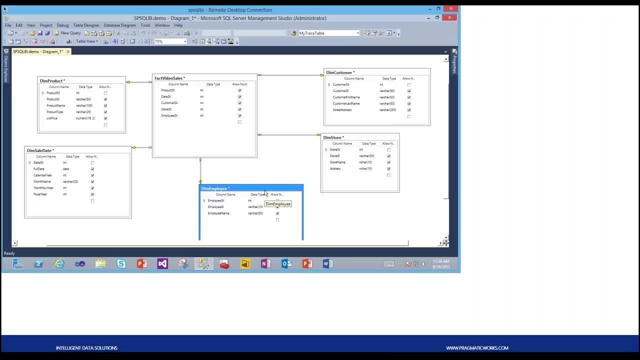 when. regarding SSAS: okay, you'll notice here that I included a date dimension. this is very important for analysis services, and so you want to make sure that you always include a date dimension in your data warehouse. and some of you out there may be thinking, okay, well, that's silly. yeah, we want a date dimension. 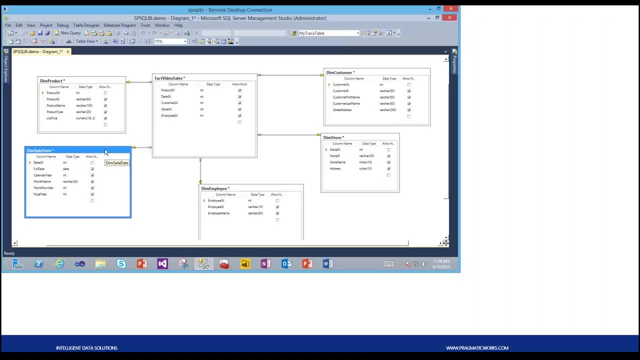 or data warehouse, but I have. I have seen data warehouse and I've seen cubes before that didn't have a date dimension, and so it was always. it was always just kind of known by the users that, okay, this is just a point in time, right, there's the date is going to be what. 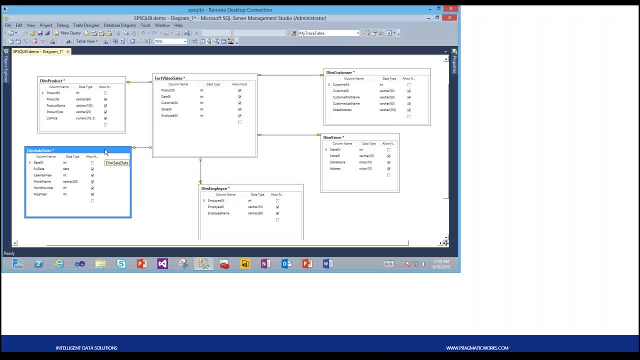 ever is the last current date available, which is not exactly all that useful because if you don't have a date dimension, you can't track things that you know that aren't aren't included with. you know basic t-sql functions like company holidays or fiscal calendars, those types of things. so we need a date. 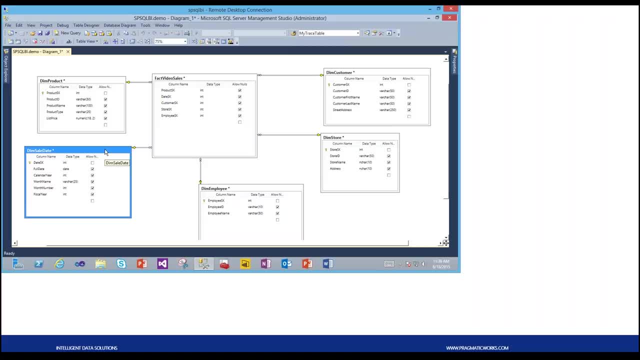 dimension to track those kinds of attributes, but also in analysis services, if you want to do any types of time calculations, like last year, last year, what, how many cheese balls do we sell last year? or or how many movies did we rent last year? or if we want to do any type. 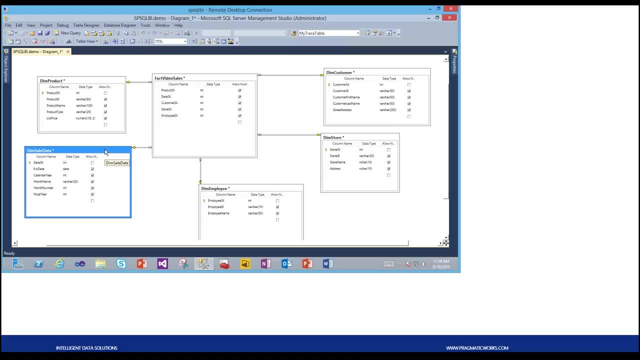 of year-over-year growth analysis or if we want to build any trend reports or anything like that, we're going to need a date dimension analysis services to do that now, as I've kind of gone through the dimensional model here, our star schema here, and I've put in the attributes into the tables I've just 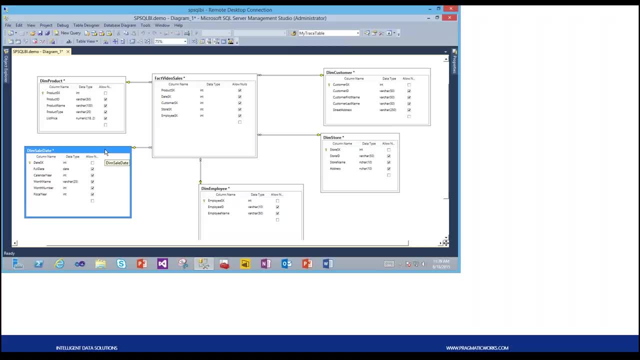 kind of used generic data types, and so this is just from a purely you know, exercise standpoint. and so the data types here aren't that important, but in your environment you're going to want to make sure that you have a date dimension. the data types here aren't that important, but in your environment they are very important. you want to. 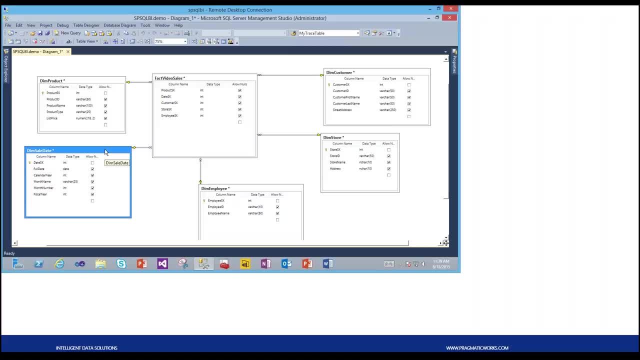 make sure that you use the smallest data types possible, because this is this is going to play ripple effects into analysis services. so if you don't set your data types up correctly and you just set everything in your data warehouse to a string, we're saying: you know what everything is? VARCHAR 50 and. 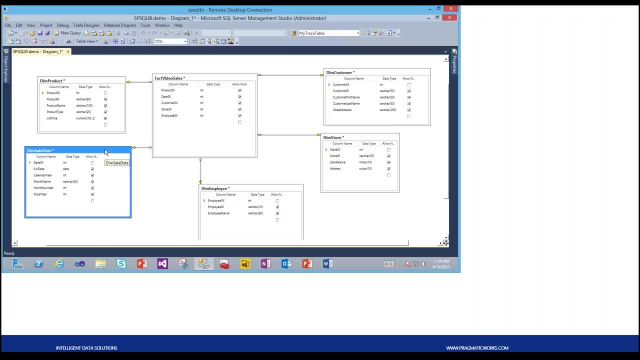 that's what we're gonna go with. this is gonna- this is going to negatively affect the performance of ssafs, and the reason for this is because, in analysis services, your string data is actually stored in a separate file, and so anytime analysis services has to act in a separate data set, it has to act in a separate file, and it's gonna be. 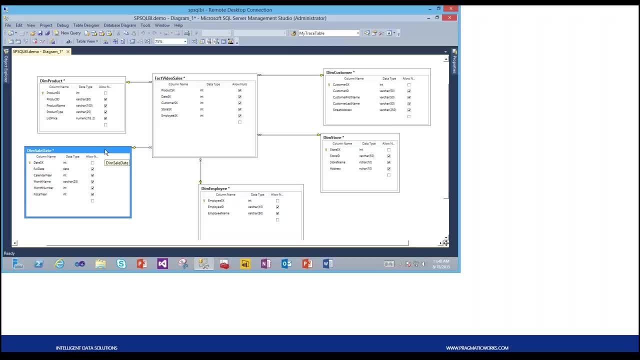 access a string data- whether it's a customer name, a store name, an address, a month name, anything like that- it has to go to this other file, look up that data and then return it to the results. So there's going to be a performance impact to your queries and processing of your cubes. 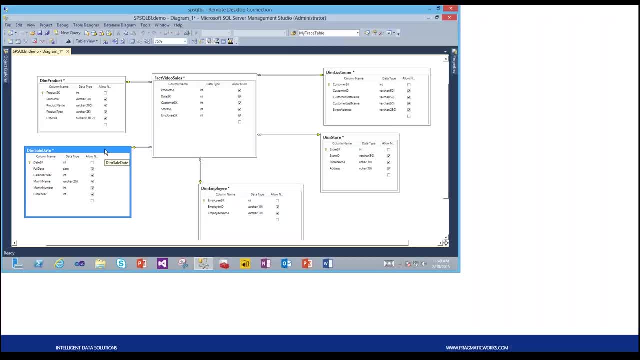 when you use string data. So it's important to use the smallest data type possible. If you can store something in an integer or a big int, you want to do that, because that's going to improve the performance of your cube. Also, it's important to just kind of remember that a single field, non-nullable integer key. 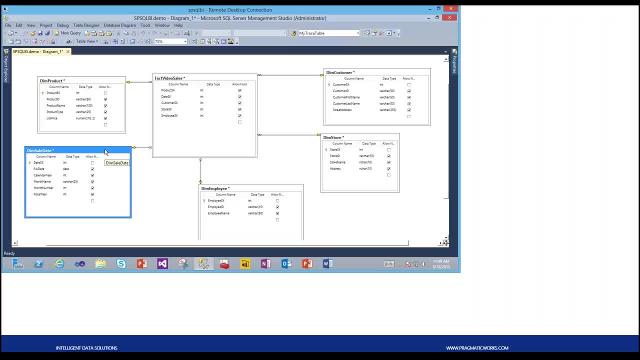 is the best data type we can use. So if you can do that, do it. But, like I said, the best data is going to be the descriptive data. so you don't want to go overboard, You want to strike a balance there. 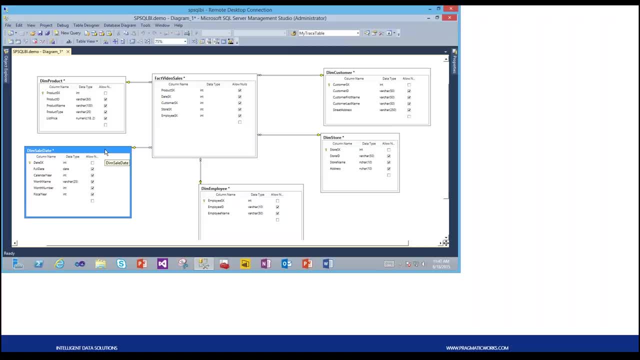 If you can store a customer name and use the customer ID- that's an integer- as the key value for that column, That's something good to do there as well. Also, one thing that you want to keep in mind as you're going through the design of your 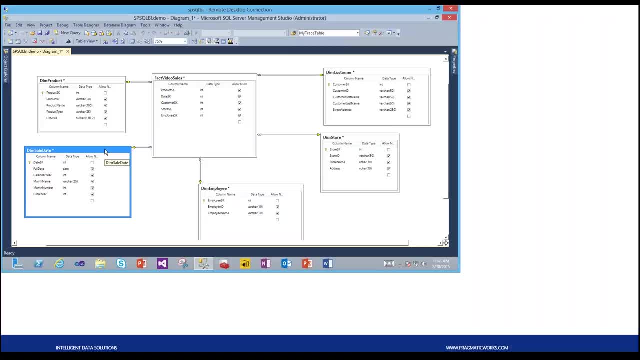 star schema here is: use user-friendly naming conventions. Don't go with. you know, don't expose things like fact video sales to the users. You want to expose it as maybe just video sales in your cube. You know, DIMM employee. they're not going to understand that DIMM is short for dimension. 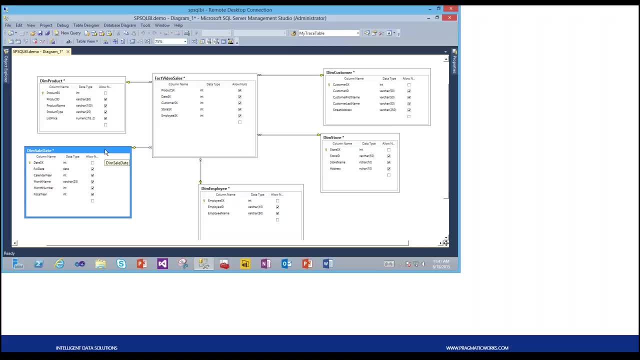 so you want to expose the objects here in a user-friendly way, And the last thing I'll say about this- is I'm going to talk about dimension optimization- is: look for opportunities to build in natural hierarchies into your dimension design, And so we're talking about hierarchies. we're talking about, you know, arranging the relationships. 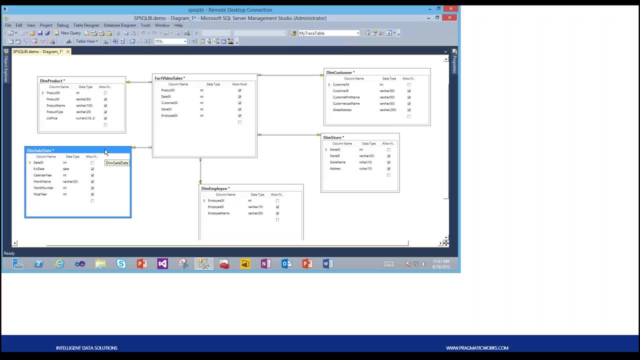 between the data in a natural way, such as you have calendar year at the top, you have months under that, then you have date right. so you have this kind of natural hierarchy, these natural relationships that exist between the data, because you can build those kinds. 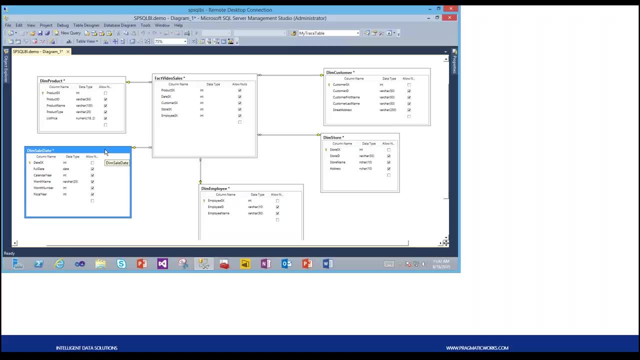 of relationships into a data. You can build those into analysis services, And when you have those attribute hierarchies or user-defined hierarchies correctly built into analysis services, it gives you a performance bonus. so that's something you want to consider as well. 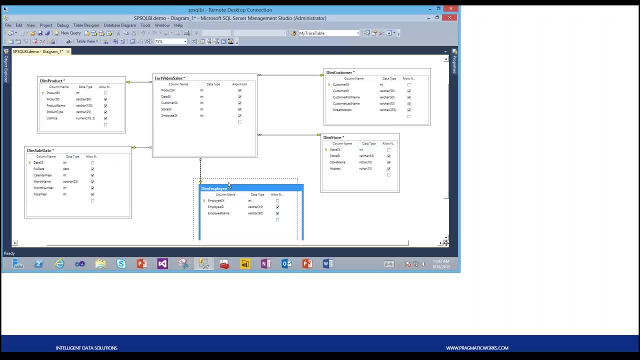 All right, so I don't think I'm going to go any farther with this. I think you guys get kind of the point here of what we're doing with the dimensional model here, And so once we've identified the business process as step one, then we've identified 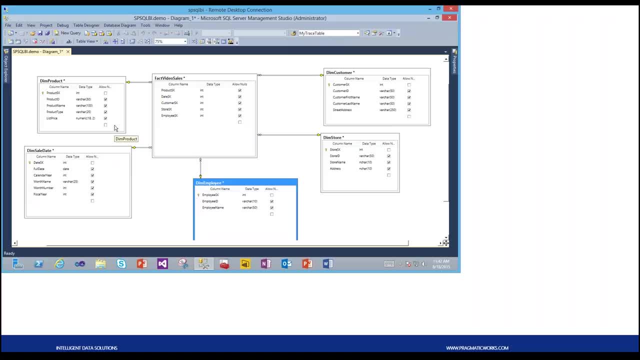 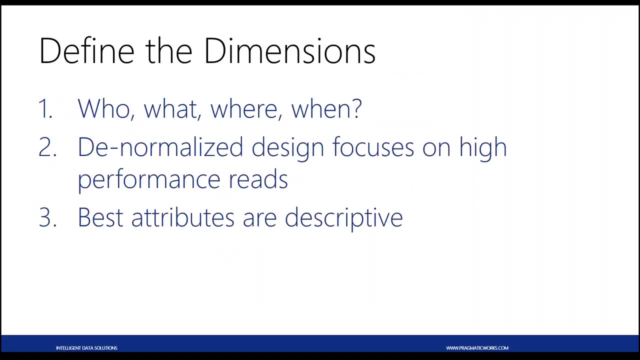 the grain And then, based on the grain, we're able to correctly determine the dimensions and the attributes that are going to make those dimensions. It's time to move on to the last step, and that's identify the measures that we want to include in our fact table. 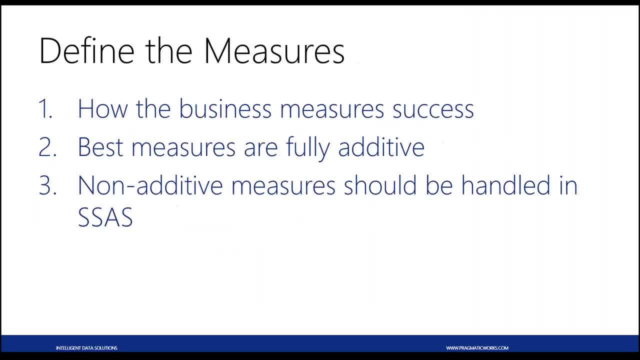 So the measures are going to be: how does the business measure success? So this is going to be. you know, say things like sales amount. You know What was the sale, What was that line item sale amount, What is the product cost associated with that sale? 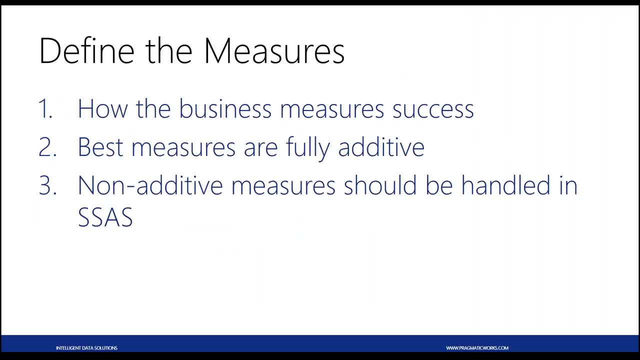 How many videos were on that line item? Did they rent, you know, a DVD copy of, you know, Dances with Wolves and then a VHS copy of Dances with Wolves, You know? whatever the case may be, Or did they get you know, 10 bags of scales for their fat little kids? 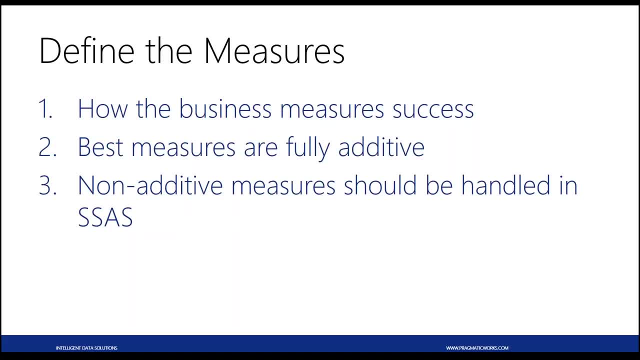 You know. so you're going to have a quantity associated with that too that we probably want to track. Now I'll say the same thing here that I said when we were discussing designing, or when Mitch was discussing designing the dimensions. 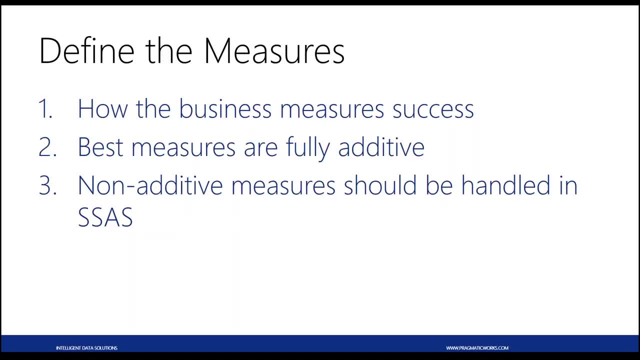 If we identify a measure that violates our grain, what do we have to do, guys? We've got to go back to step two. right, We've got to go back to step two because we've come up, we've identified something. 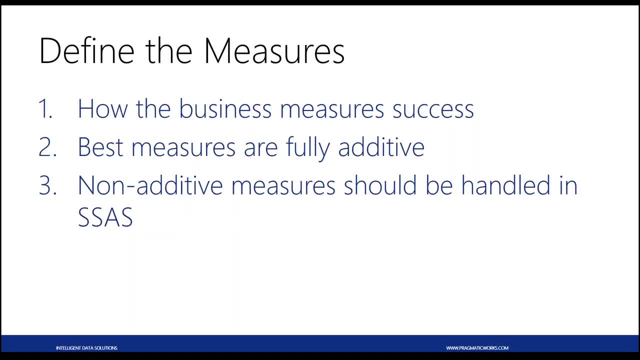 in our model. that violates our grain. so we've got to go back to step two. Let's revisit the grain statement. make sure that we actually have that correct and then we can come back. We can go back to step three. make sure our dimensions are squared away. that's all correct. 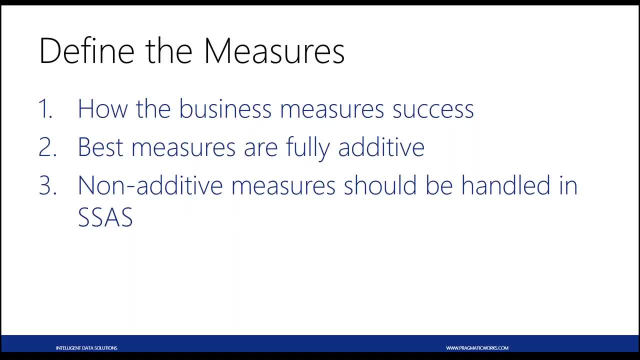 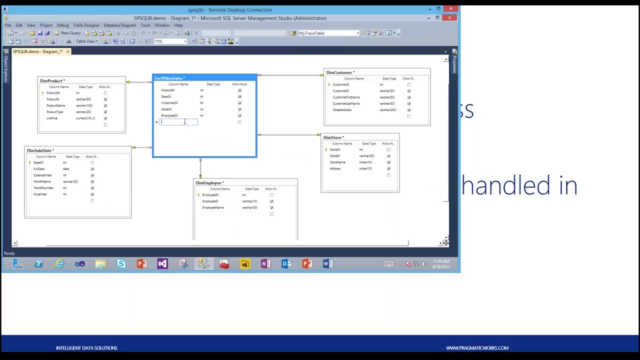 And then we can come back to step four, where we're going to identify our measures, identify the facts. So in this particular case, let me pull back up my dimensional model here. Now we're ready to get started with the step where we're going to build in the measures. 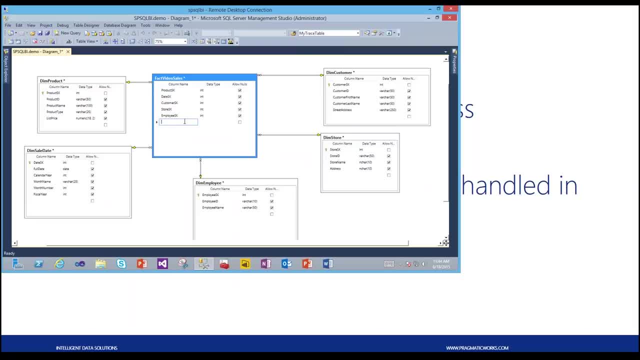 into our cube. So we consult with the business, say, hey, you know what are the measures you guys want to track, What are those high impact, low risk metrics that we want to track here in our cube or in our data warehouse? 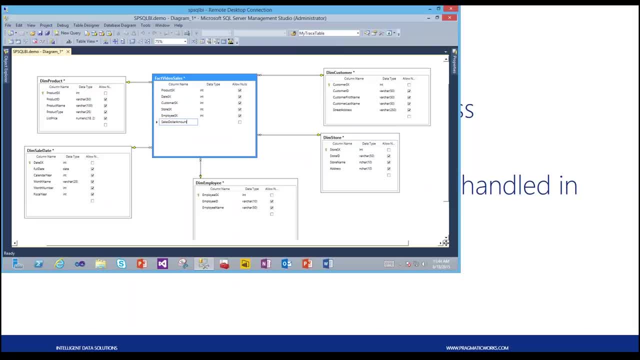 So they may say, okay, well, we want a sales dollar amount, right, That's important. So I'm just going to put these as in, but you know you probably do like decimal or something. There's going to be a quantity associated with that, right. 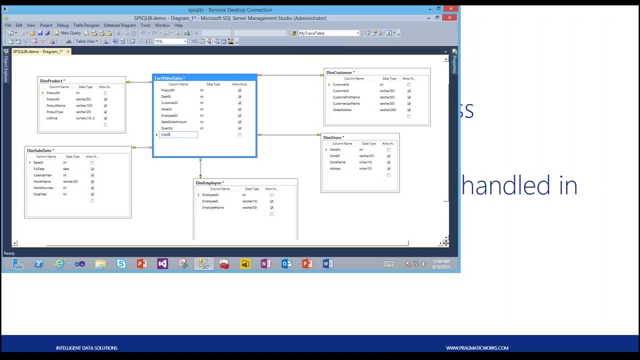 And maybe there's also going to be a cost, a cost amount, right, And that would be important to track if we wanted to, you know, figure out any type of- you know- profit or do any profit margin type calculations. 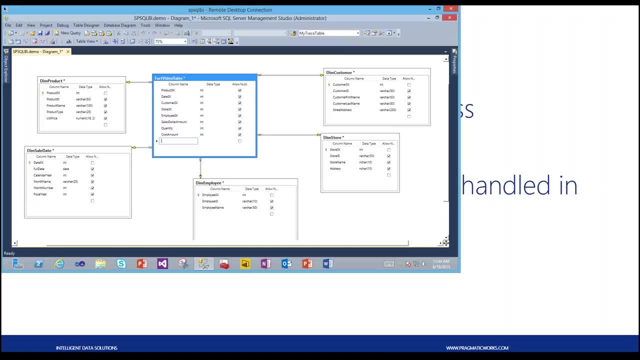 Okay Now, and I'll just go ahead and put those three in and we'll just stick with that, because those are three pretty common measures that you probably have. if you have a retail business process modeled in your data warehouse, you probably have those types of measures as. 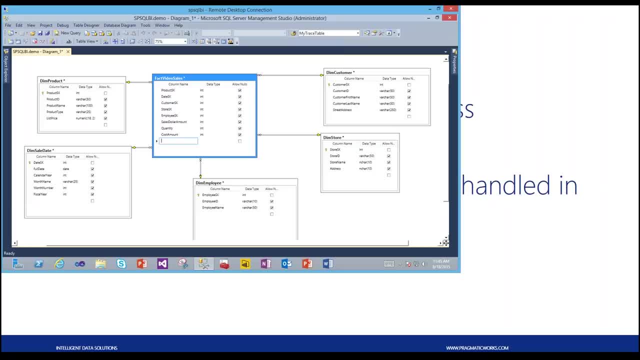 well, But you might have other things like a shipping amount or a tax amount or you know whatever. whatever the case may be, Now, when you're identifying measures for your star schema, the best measures that you can put in your star schema are going to be measures that are fully aggregatable or are 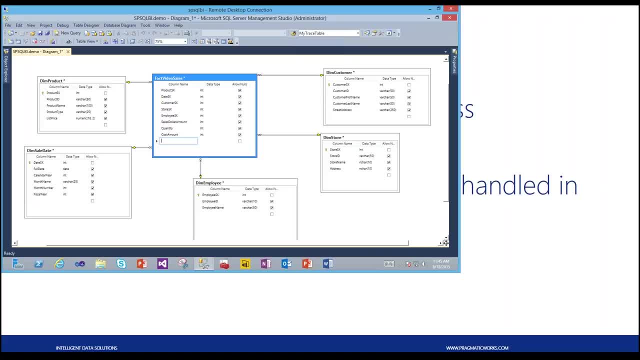 fully additive, And what I mean by that is measures that can be rolled up. they can be sliced and diced in any way, shape or form, and the number always makes sense. So, for example, if we roll up our sales for all geographies, I can see what are my sales. 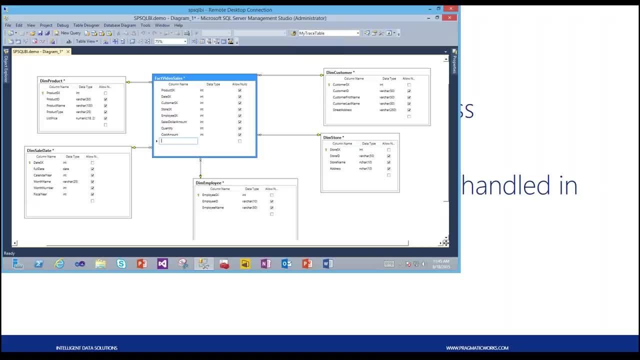 across all of my geography regions. right, That number makes sense. If I want to see my sales for customers, that number still makes sense. If I want to see my sales by month, I can slice it by month. That number always makes sense. okay, because it's a fully additive, fully aggregatable. 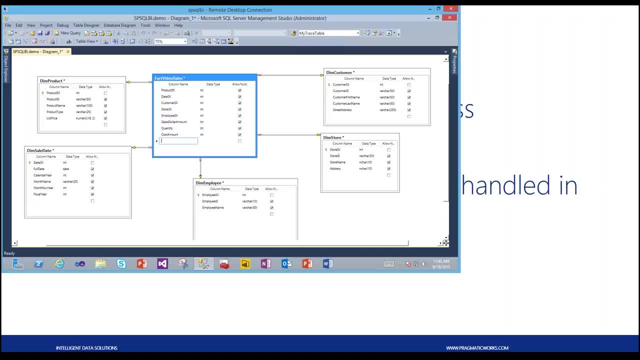 measure. Those are the best kinds of measures to include in your queue, because your user really can't slice that wrong. They have to work pretty hard to mess that up right. So measures that are fully additive, fully aggregatable and that are always valid- no. 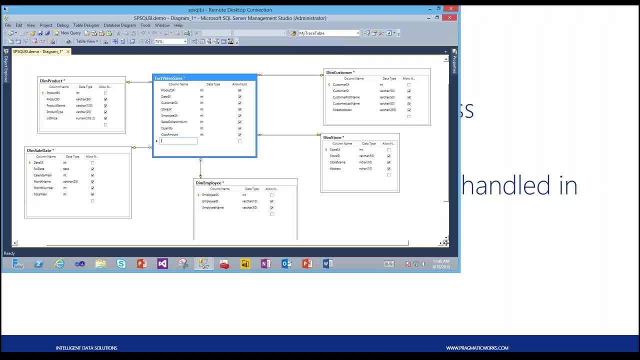 matter how they slice and dice it, those are going to be the best measures to include in your data warehouse or in your queue. Now you may have a requirement for some measures that are not additive at all. You can't add them up and have them make sense. 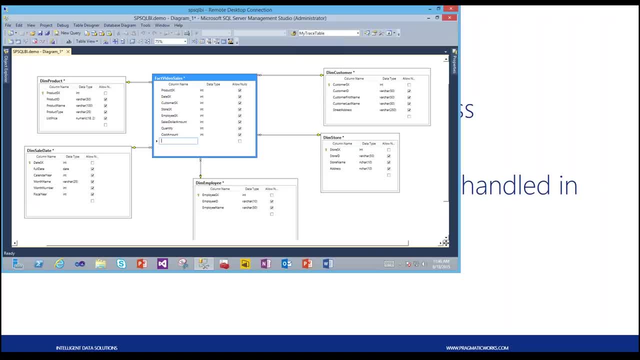 So an example of something like that would be Profit margin, right? So we can't put profit margin in the table and then have the user add that up, because that number would be nonsensical, right? It's not going to make sense to the business or the users if they add up profit margins. 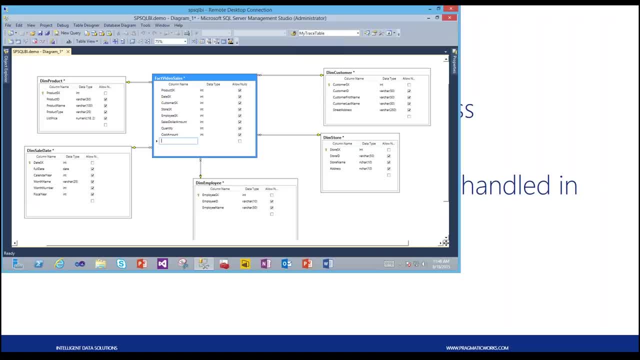 for all geographies and they'll end up with some crazy number that won't make any sense, right? So measures that are non-additive, those are measures that are going to be better handled in the data access tool. So it may not be SSAS. 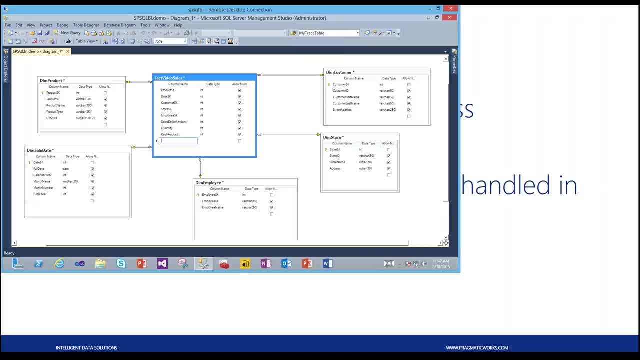 You may not be an SSAS shop, right? You may be using some type of other reporting technology, like Tableau or something, or maybe you're even doing it in Power BI, or you've got something else- Power Pivot or something else- going on there, right? 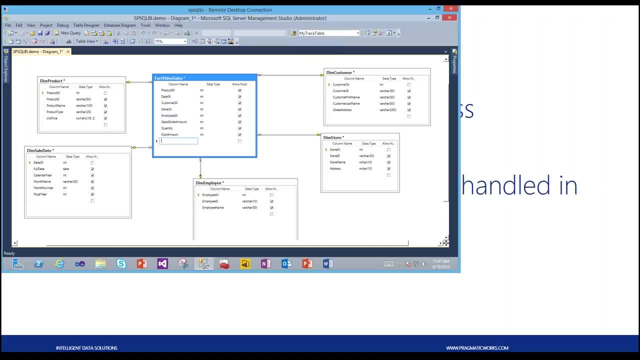 Those types of calculations like profit margin are going to be better handled in the data access tool and certainly SSAS can handle those types of calculations. Also, if you want to do any type of time calculations like sales amount for last year, sales amount. 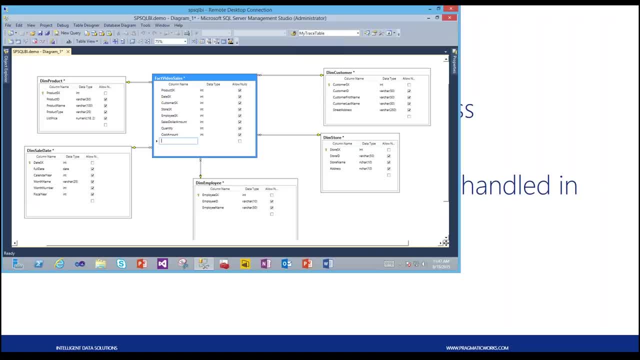 or your year-to-date quantity, or my year-to-date Or my last year year-to-date, so that way we can see: are our sales growing this year compared to last year? Are they actually increasing Unit price? Those types of measures are going to be measures that you want to handle in the data access. 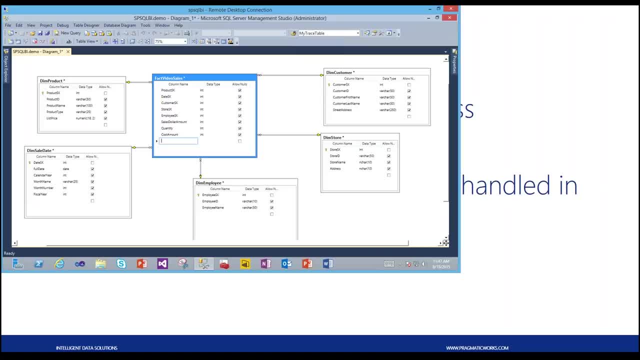 tool or SSAS. Also, if you have any type of KPI metrics that you used, kind of the red light, green light, yellow light type of indicators, that's something that's better handled in SSAS, And so when you're 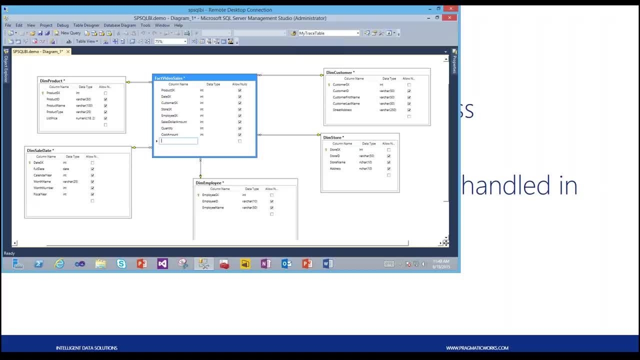 When you're, When you're planning your data warehouse, and if SSAS is in the picture. you want to keep in mind that a lot of measures can be better handled with SSAS: Those measures that are non-additive, like ratios or KPIs or time calculations that 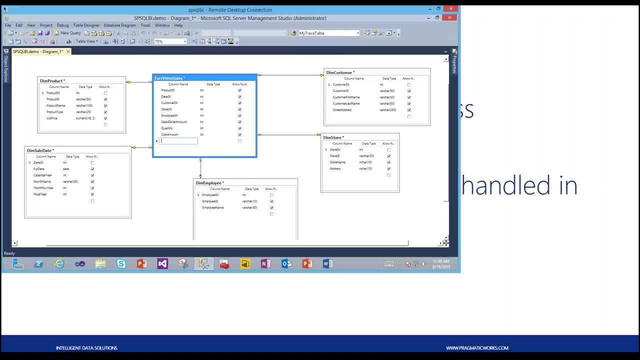 those are better to be handled with SSAS than in your data warehouse. If SSAS is not in the picture, then you're going to have to jump through a lot of hoops to build in some of these dynamic type time calculations that SSAS can spit out in no. 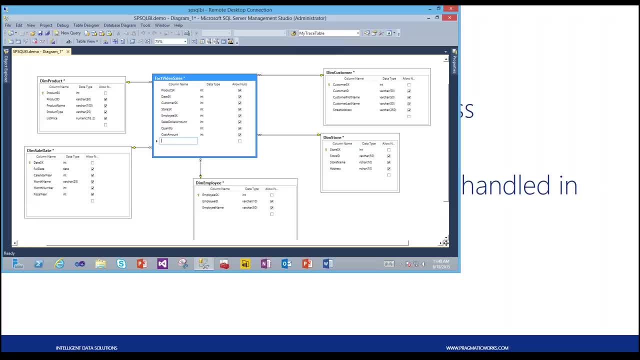 time. Also, at this point, it's also good to begin estimating how many numbers, What's the number of rows that are going to be in this fact table? right, And so it may be a small fact table You may have. 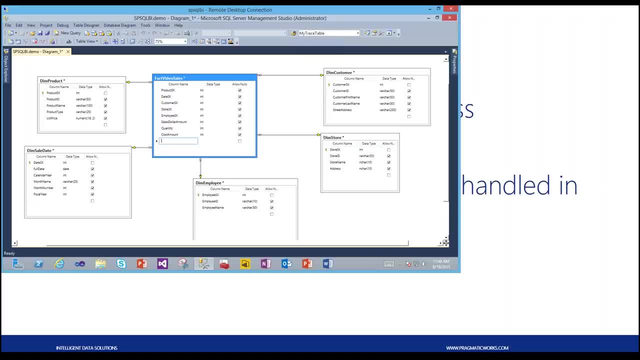 You may determine that you know what. we're only going to have 300,000 rows in this fact table, So that's not very big right. It's not. That's not a lot of data, And so maybe a clever partitioning scheme isn't appropriate in that scenario. 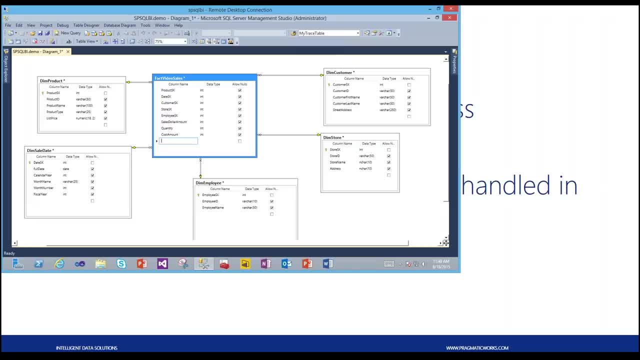 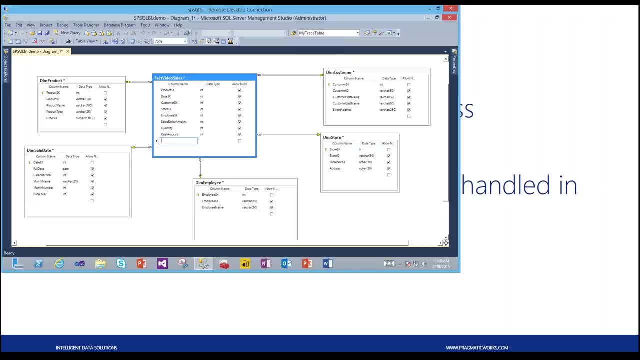 like that. You're going to have a ton of data in here And so you want to start thinking about: okay, what's my partitioning scheme going to look like? right, Can we partition this table down at a? If you're big like Walmart, you may even partition down at the hourly level, so that 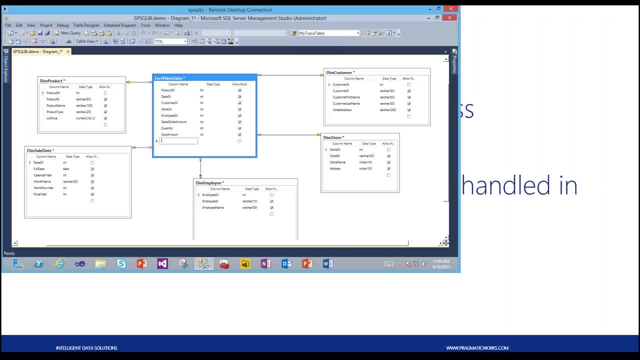 you may have 50 million transactions at an hour. if you're a company like Walmart And if you're going to be partitioning your table in your data warehouse, you can align those. You can align those partitions with partitions in the measure group in your queue. 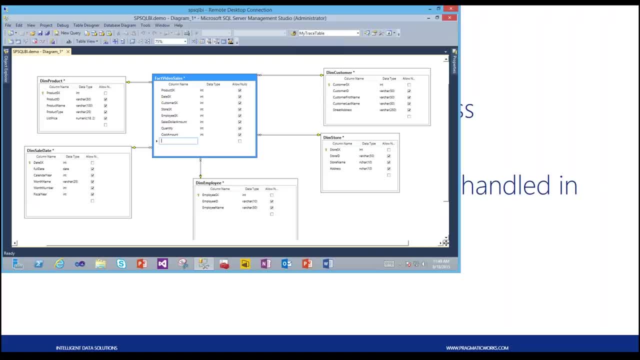 And that will give you a performance bonus. So aligning your SSAS partitions with your table, your SQL Server table partitions, will also give you a performance improvement there. Okay, And so at that point we've identified the dimensions, the measures. 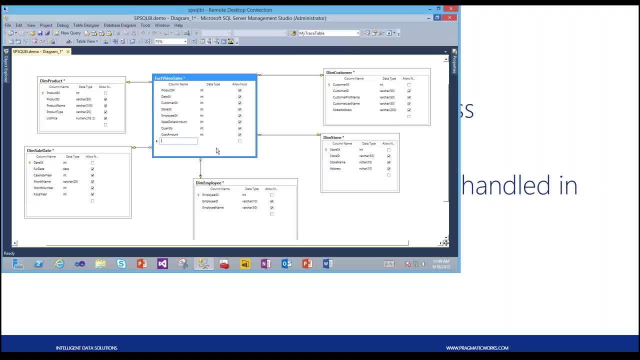 And so we've got a very basic star scheme in here that we're ready to start Kind of playing with and massaging and developing and moving on from here. So, Mitch, did you want to say something? No, 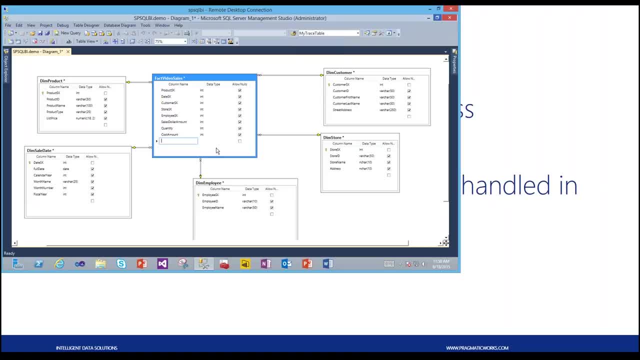 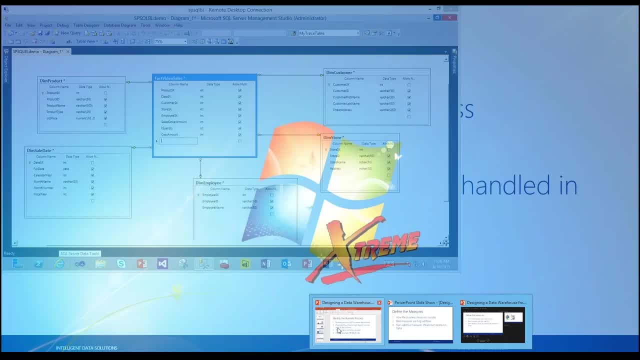 Well, we do have a lot of questions, Okay, So we'll get to the questions here in a few minutes here. So what I want to kind of do now is I just want to kind of recap really quickly And I want to make sure that we have plenty of time for the questions. 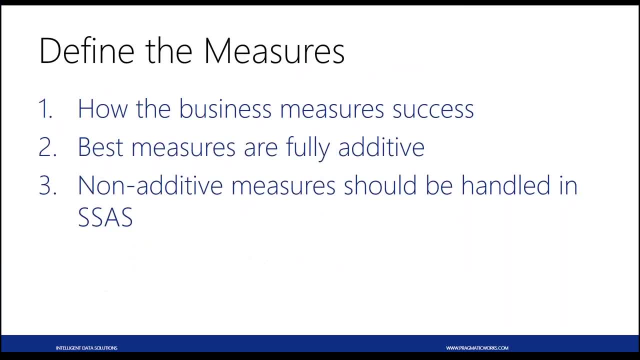 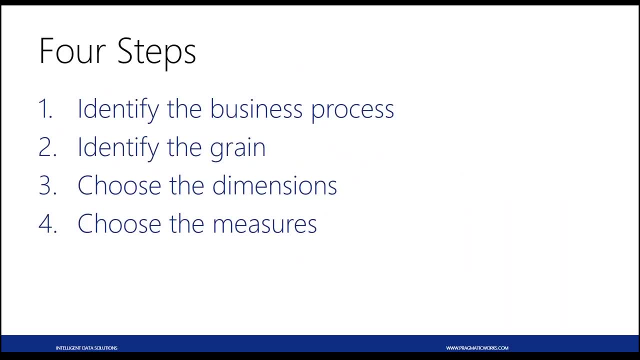 So we've got about 10 minutes left in the session here. All right, Okay, So let's recap real quick. So the four basic steps to designing your star schema are: identify the business process, And when we say business process, we're specifically talking about business process, not business. 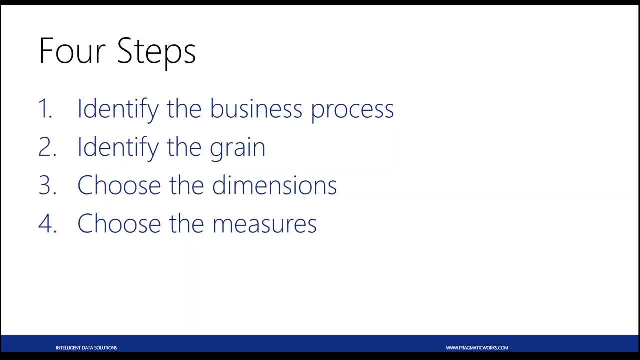 department. We want to identify the grain. What does one row in the fact table represent? We want to identify the dimensions. And if we get to this step and we decide, oh, we need a dimension that isn't represented by our grain statement, we need to go back to step two here. 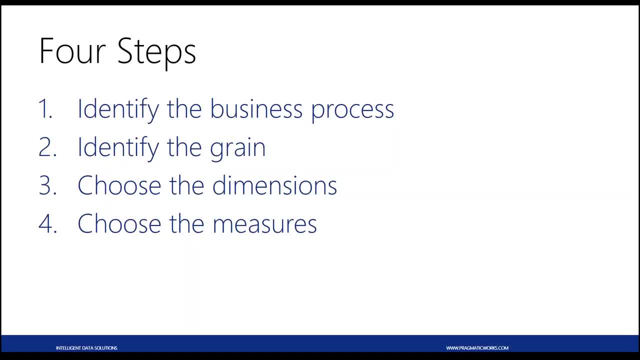 And talk about the grain, And then, if we make a change to the grain, then we'll come back to step three, choose the dimensions and the attributes and continue development from there. And then we want to go to step four, which is choose the measures that we want to represent. 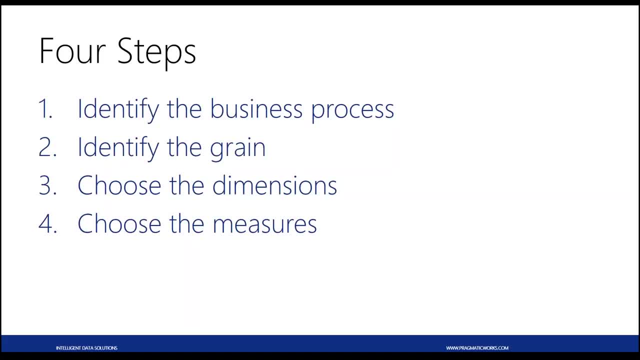 in our fact table Now. I've been consulting for eight years here at Pragmatic Works so I've done a lot of data warehouse design. I've done a lot of cube design. I've done a lot of ETL development. 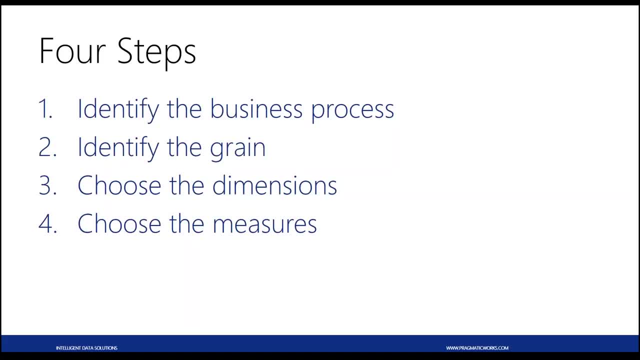 And one of the things we do at Pragmatic Works is we do what's called kind of a quick start. If you're not familiar with that is we go and we design a POC. We go from zero to cube in about a week. 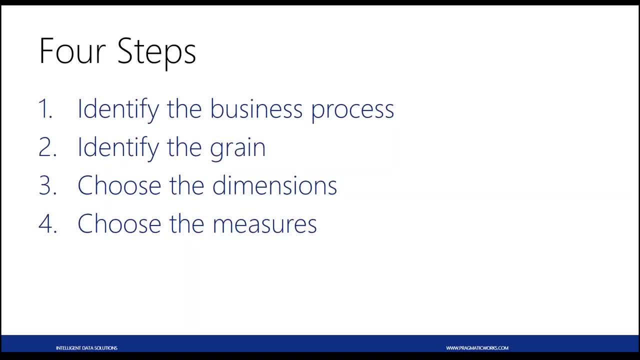 So we design the data warehouse, we do ETL, we do cube and we do reports in a week, And so it's a pretty crazy week. But I will say that this part here designing the data warehouse- we usually spend about. 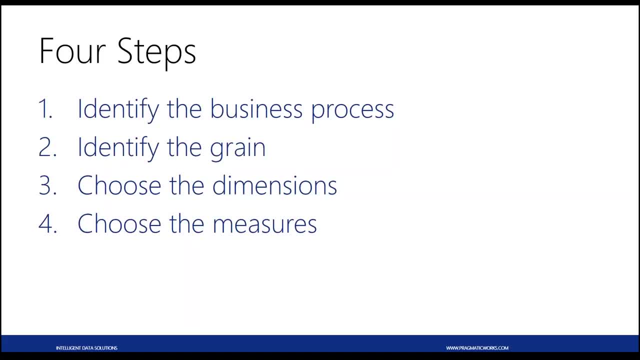 three days on it. It can be two to three days, depending on the kind of questions we have. And the reason we spend that much time, even though we still have ETL cubes and reports to do, is because this is by far the most important step. 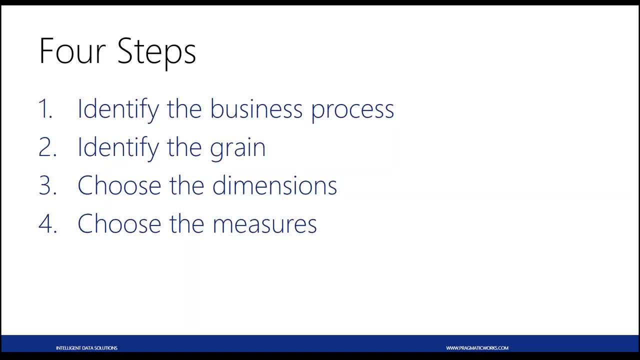 Getting the data warehouse right. If you don't get the data warehouse right, you're going to have lots of problems down the road. So this is the most important step, and that's why we spend two to three days discussing that. Now resources. 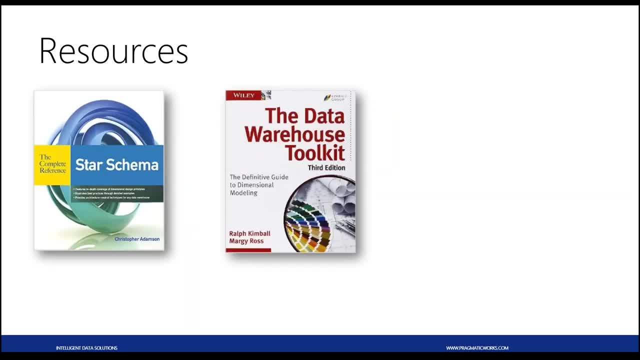 If you're new to data warehouse design, these two resources here are killer. These are the best resources, in my opinion, that you can find: The Data Warehouse Toolkit. you'll find. a lot of the material for this session came from the Data Warehouse Toolkit because it's an excellent book written by Ralph Kimball. 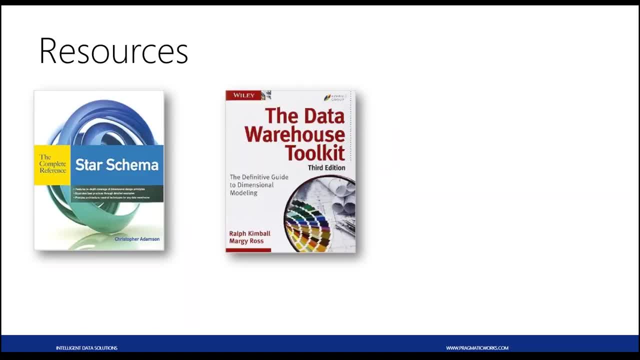 Margie Ross, Chances are, many of you out there have read this. This is a great book and it talks about these four steps and it goes into a lot more detail than what we can do here in a one-hour session. 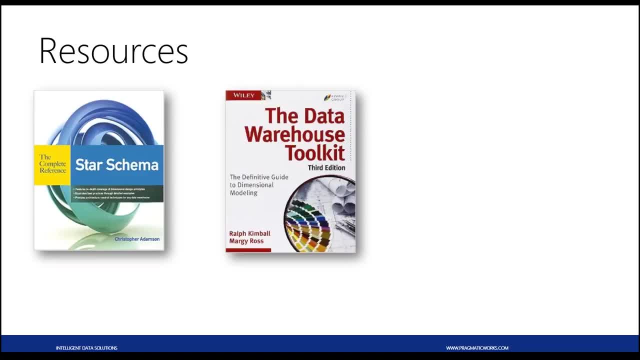 So I highly recommend this book, the Data Warehouse Toolkit, Also the STAR Schema- The STAR Schema, the complete reference excellent book as well. Both of these books, in my opinion, should be in every professional BI person's library. They're that great. 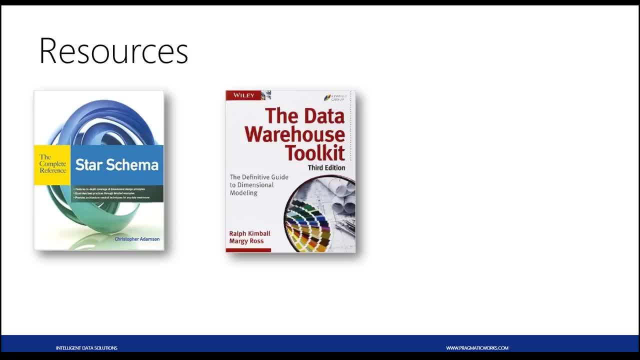 In my opinion, the Data Warehouse Toolkit is a little more instructional and the STAR Schema is a better reference, Because if you have special scenarios that you want to research, well, how do I handle a fact dimension or a degenerate dimension or a junk dimension? 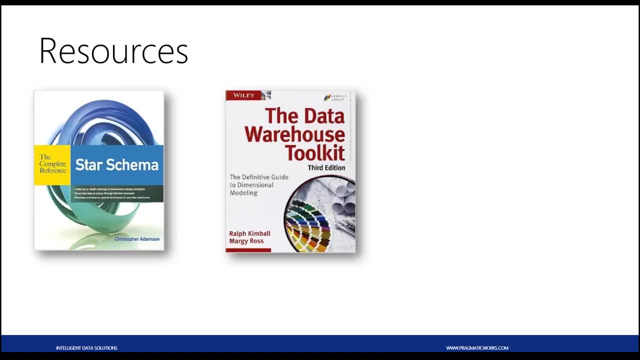 Those types of things. STAR Schema is going to be your go-to resource for that, So I highly recommend both of these as resources for you. So look those up. I have both of these books in PDF and in paper format. Mitch does as well. 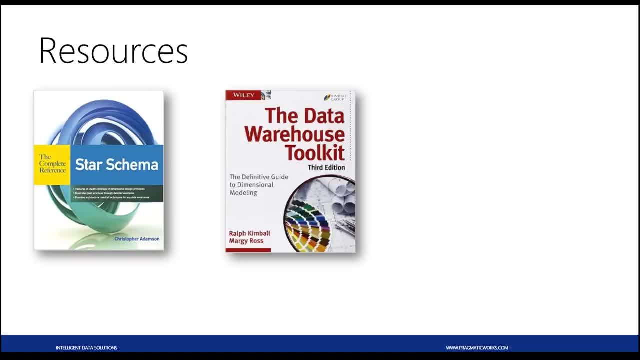 I agree, I like the STAR Schema the best. If you're an intro to data warehousing, I just think it's easier to read. I think it's an easier read. It's not. It's not heavy on the technology- The Data Warehouse Toolkit. though you will probably just read the first five chapters. 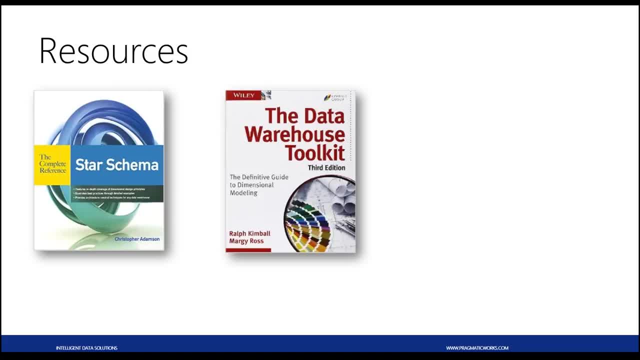 and really get everything that we talk about here and a lot more. And then the rest of that book goes department by department, So it has retail, human resources, finance and how you would model each of those different businesses. So it's an awesome book, an incredible book. 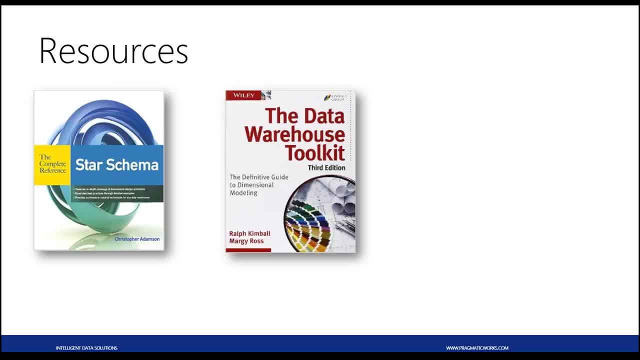 But I highly recommend both of those books. Yeah, they're great books. And one other thing I'll say- the last thing I'll say about those books is that the really nice thing about those books is, for the most part, they're technology agnostic. 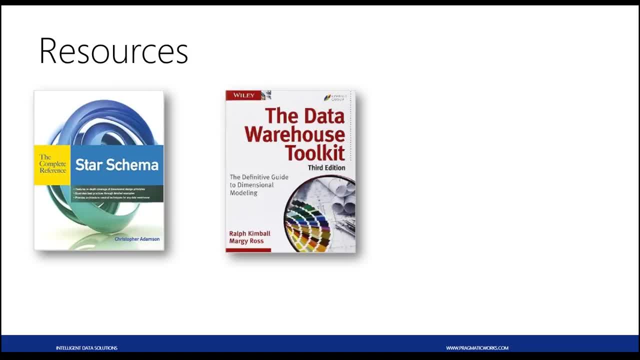 So you don't have to know a lot about SQL Server, You don't have to know a lot about Oracle, whatever your database technology is, because they don't approach it from a technology standpoint. They're talking about it from a modeling, conceptual standpoint. so that's really nice. 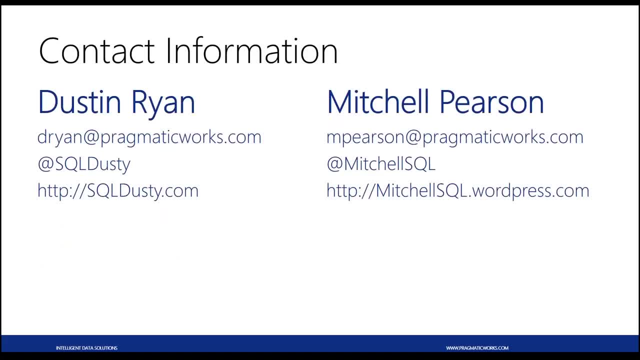 So thank you everybody for attending our webinar. I hope that you learned a lot. I hope that you got a lot out of this session And if you have questions, now is the time to start asking your questions. I know we've got questions piling up now. 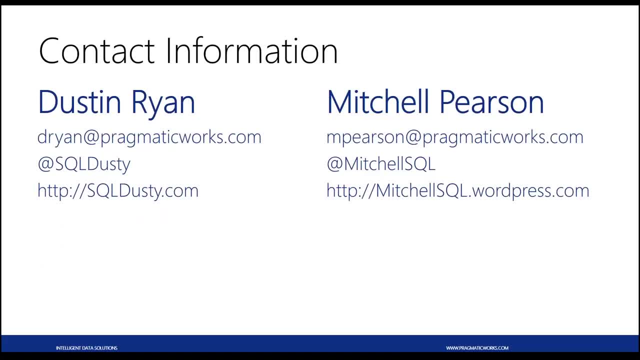 And we've got about 500 people in this webinar, So it's going to be impossible for us to answer every single question, but we'll get to as many as possible. I put up on the screen mine and Mitch's contact information. You can email us at those email addresses. 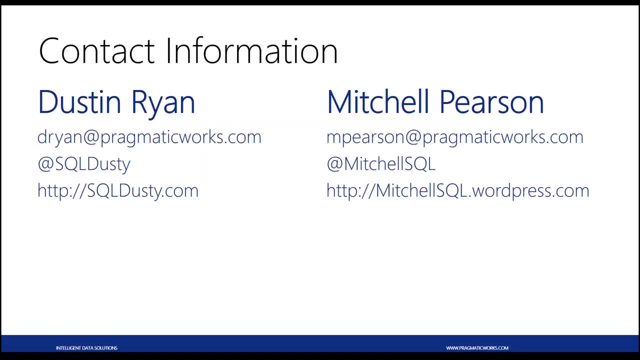 If you're a tweeter, you can tweet us there. at SQL Dusty is my Twitter handle. at Mitchell SQL is Mitch's, And then there's our websites. there We blog about all kinds of different Microsoft BI-related things: SQL Server scripts that. 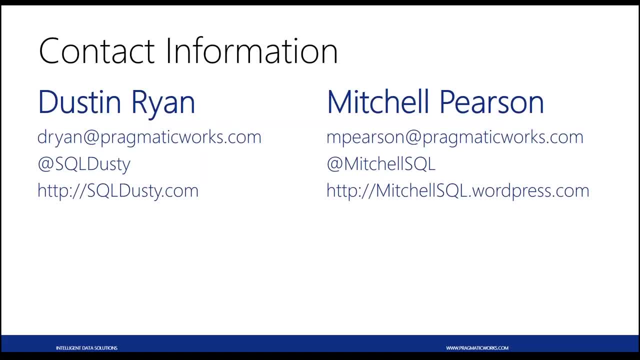 we think are useful: SSIS, design patterns, analysis services, stuff, MDX, Power BI, all kinds of stuff there. So check out those blogs. You can ask us questions there as well. If you have a question and you can't get through on the webinar, there's the Twitter handle. 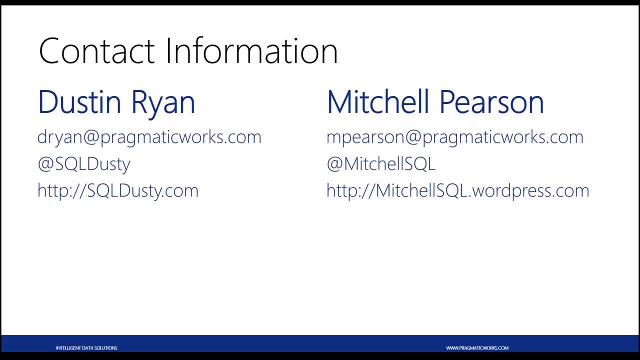 at pwquestion or, I'm sorry, hashtag pwquestion. You can use that for your and you can log onto Twitter and you can tag your question with that hashtag and we'll go and take a look and we're going to answer questions here. 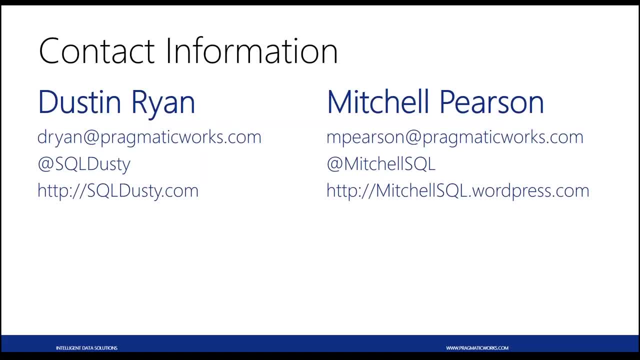 in the webinar for now, But then, when the webinar is over, we're going to take the remaining questions on Twitter, So check that out as well. So, Mitch, Do we have questions? We have more questions than I've ever seen. Oh my goodness. 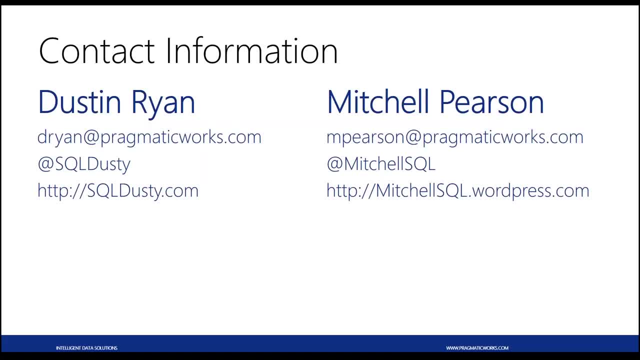 I cannot keep up with these questions. We'll handle these as best we can. Let's try this one right here. All right, Easy question: How did you get to the database design window? How did you get to the database design window? 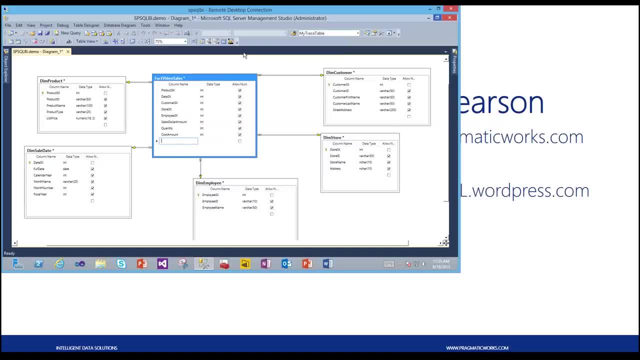 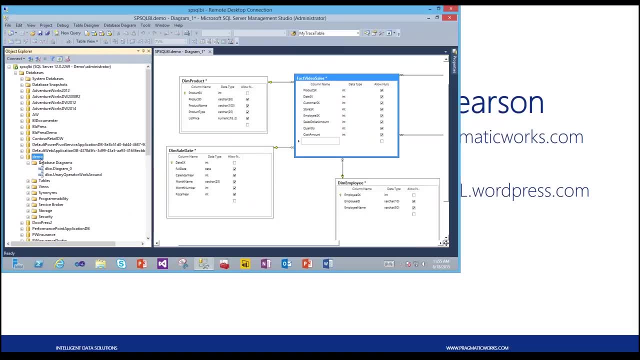 Okay, Database design window. So this is in SQL Server Management Studio. So that's a good question. I'll just pull that up real quick. All right, So there's my database design window, Whatever, And I went into my database. 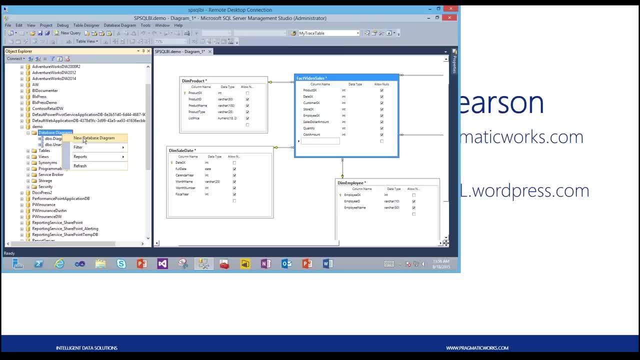 I just got a database here set up That's called demo, And I went to my database diagrams folder and I just right clicked and set selected new database diagram And so if you have tables that are already in your database that you want to add you. 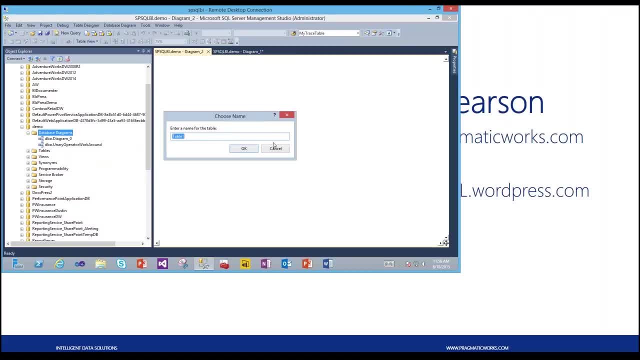 can select those here and click add, or you can just right click and start naming new tables and creating them from scratch. So pretty, pretty simple, All right. So another question we had was about using the surrogate key, using an integer value for the date. 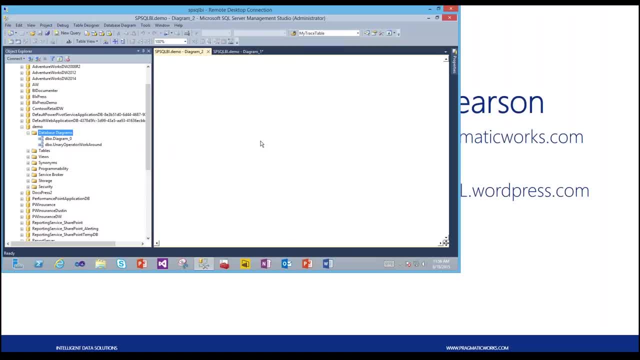 Why do we do that? Why would you recommend that over using the date? One person, I believe, said that they think that the Kimbell book- actually the one you recommended- actually recommends using it. The date: Well, the reason that we go with the integer- and I can't remember specifically why the 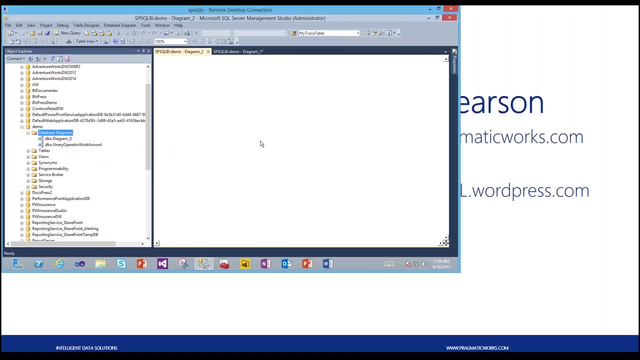 Kimbell book said to go with a date data type and I'm going to guess here and say that it's because it's a more user friendly value. But the surrogate keys are important in an integer type format is because they're going to perform the best right. 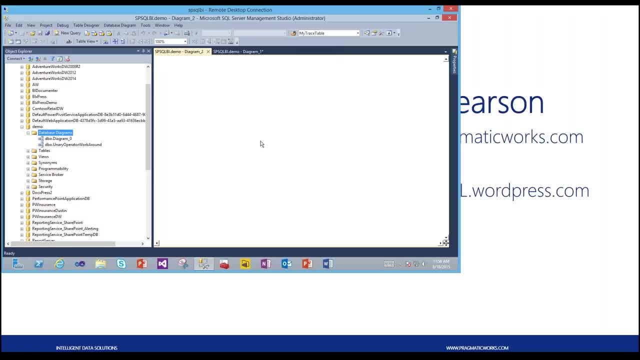 And they're the way that we create relationships between the dimensions and the fact tables. And remember, the whole goal of the data warehouse is high performance, And so a single field, non-nullable integer key is going to perform the best, And so that's the reason we go with an integer field for our date key in our date dimension. 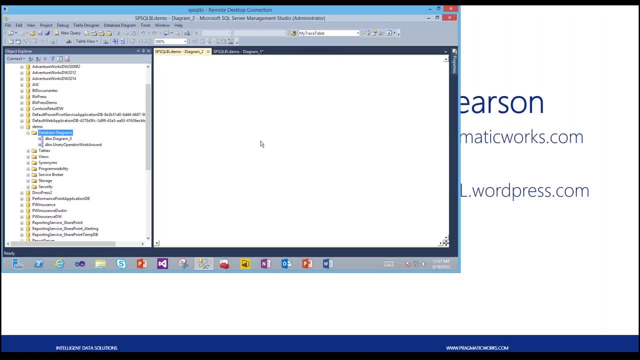 Now I'll also mention here that this date key is a little bit different than our other keys in our other dimensions, because instead of going with just an identity column where we're just going to auto increment it one at a time, we're going to go with our date. 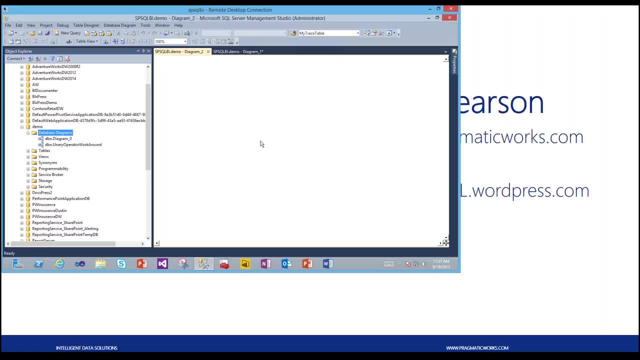 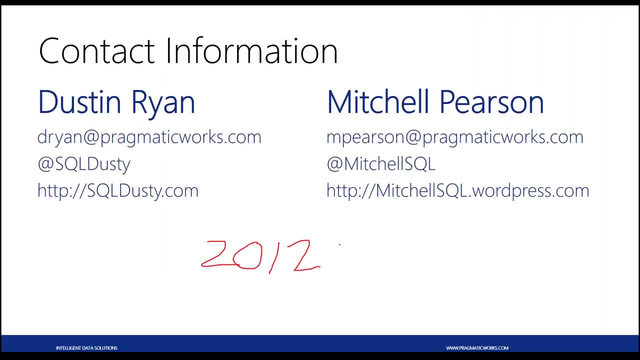 dimension with what's called a smart key And basically the format looks like. it'll look like something like this: right, If you're looking at my screen: the format for January 1st 2012,. it's going to be an. 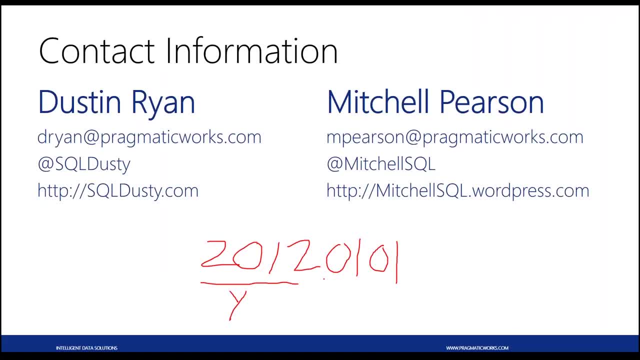 integer value, but it's going to be formatted to look like a year, a month and a day, So it's still going to be user friendly. but then at the same time we're going to get the performance benefits of having a non-nullable single field integer key in the date dimension. 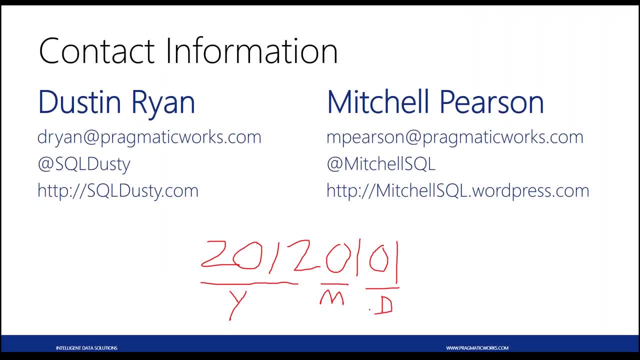 So that's why we typically go with the smart key, The date Plus. if you're trying to find a record in your date dimension or in your fact table, you don't actually have to join to the date dimension to get it, because your fact table 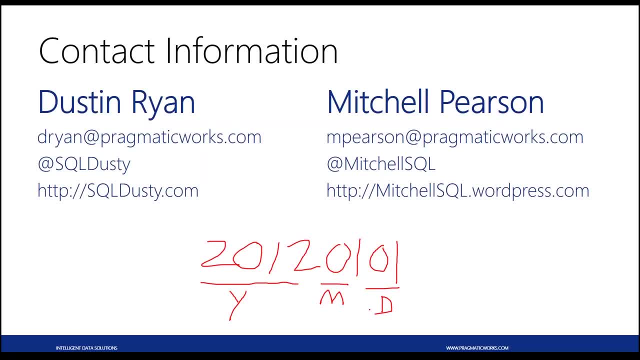 already has the date stored in the date SK and so you can read that, and so that's kind of nice too. But that's a good question as well. Do you want to try to take one more? This one's a little tough, but there was a lot of questions around this one. 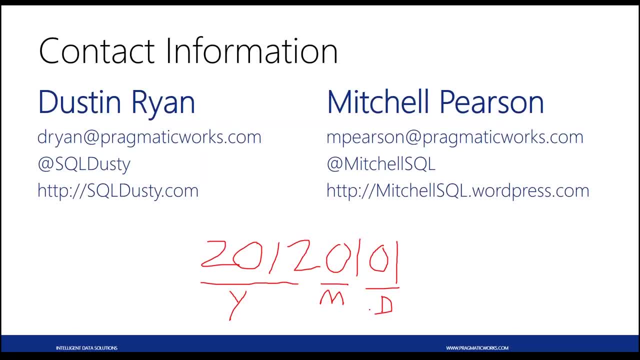 It's something that Dustin will have a blog out there with a lot of these questions answered for you, but they wanted to know when you would have a dimension with a dimension. When would you break off For a snowflake? And there was a lot of questions around that. 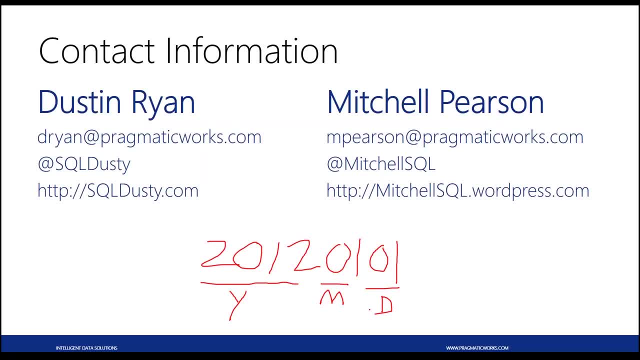 Yeah, and that's kind of a big hot debate topic because some people will say: well, you might want a snowflake, right, if you want to. Maybe you want it, for instance, something like product and product category right. 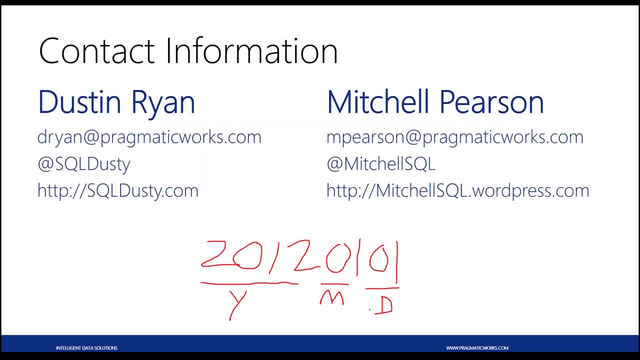 Maybe you want to break product category out, because we might have another fact table that doesn't relate to product but it relates to product category. Maybe we've got a forecast fact table right That we don't forecast at the end At the individual product level. we forecast at a product category level, and so we might. 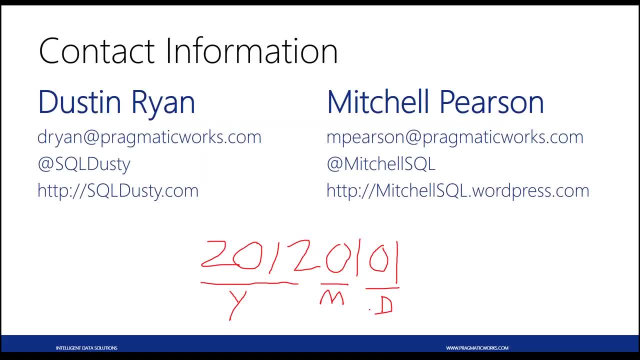 have a forecast fact table, And so that may be a case where you'll see some people say, hey, we want to snowflake that out Now, that's fine, and you can convince me that you may want to do that. but one thing that 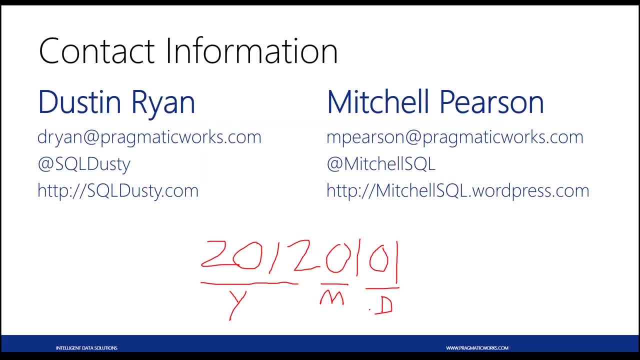 I'll mention in regards to analysis service is that when you begin snowflaking in your data warehouse, there's going to be an impact on the design of your cube. So, analysis services- you have what's called a reference dimension right where you use. 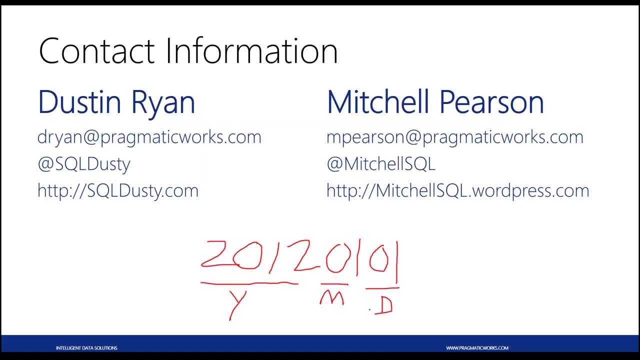 an intermediate dimension to relate that product category to our fact sales table, And so there's some impact there with having a reference dimension which you can find on my blog sqldustywordpresscom. If you do a quick search, let's see I've got it up here. I'll pull it up real quick. 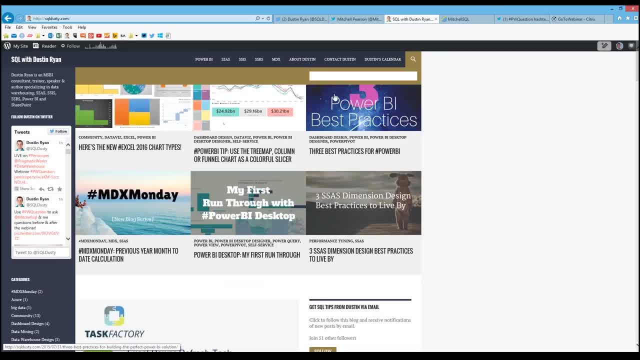 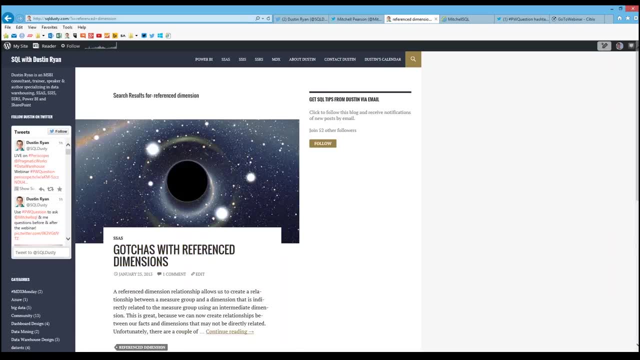 So there's my blog, sqldustycom. So if you go to sqldustycom, you search reference dimension. Okay, Great, That would be great, So let's see. so what I got over there is: I've got a reference. 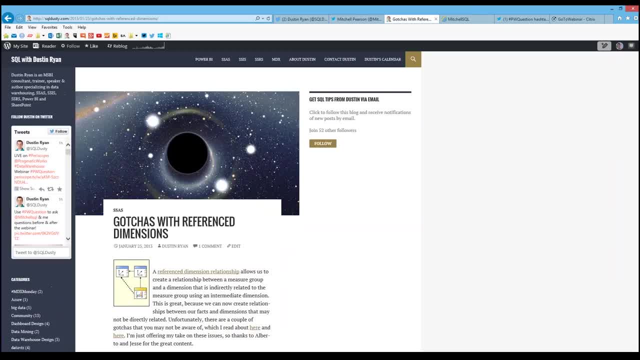 dimension. Okay, I want to create only that reference dimension. I want my collection or 25, but if I'm going to create the whole Sachen collection all at once and combine most of it with the reference dimensions, this is going to create. 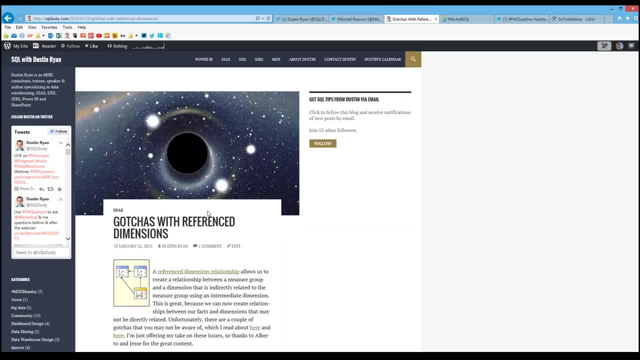 a reference dimension, All right. There's a lot of reasons why you might consider going with a star schema and typically you see that with people who are more come from a transaction or an OLTP development side because they want to. they tend to want to kind of normalize things a little bit because 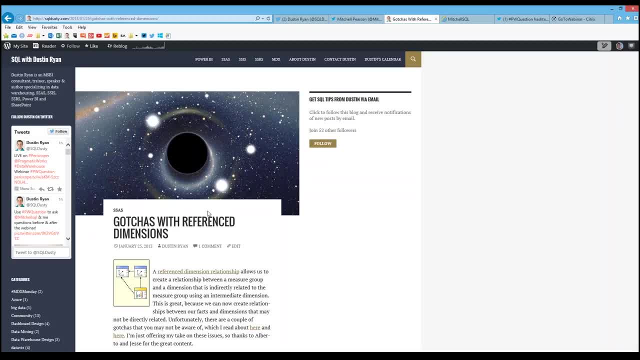 that's what they've always done. It's kind of leaning towards that more third, normal form kind of way of doing things. But you'll get better performance and you'll get better performance with your data warehouse, loading your data warehouse and querying your data warehouse. 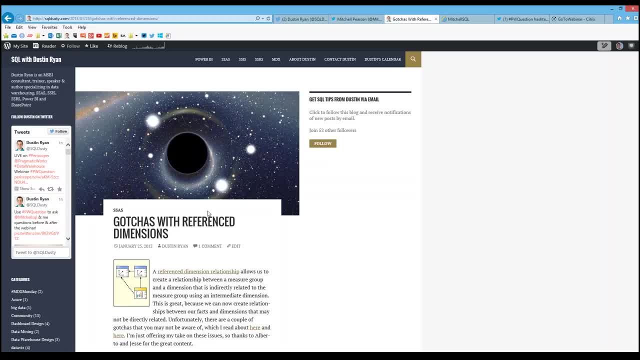 If you try not to normalize things, if you stick with a more denormalized design because, remember, the bottom line is we want good performance, right, We're willing to sacrifice some storage, we're willing to sacrifice some redundancy or some duplication of data, rather for better performance. 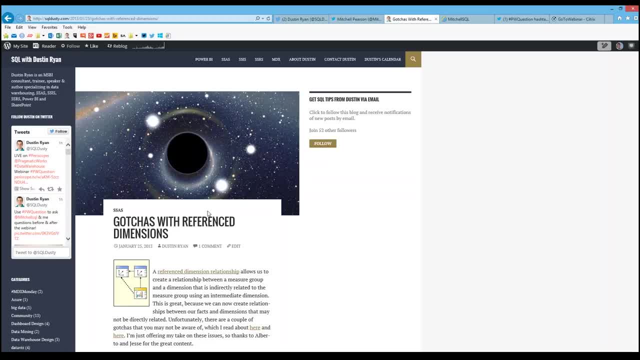 That's really the end goal here is query performance, query performance, query performance. That's a good question as well. All right, I think that's all we have time for today, but we're going to be doing some questions afterwards, Is that correct? 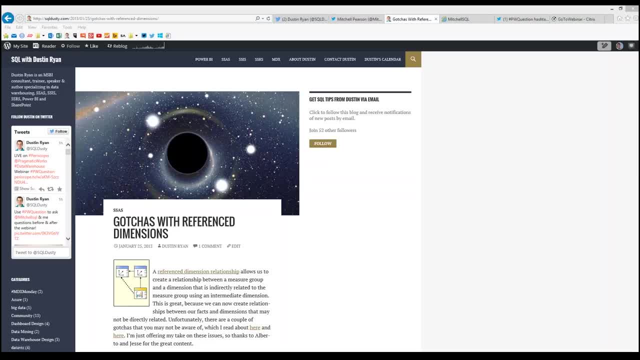 Yep, yep. So if you have further questions, we'll take questions for about 15, 20 minutes or so on Twitter, Depending on how crazy it gets. we'll try to get to all the questions on Twitter. There's the hashtag- hashtag PWQuestion. 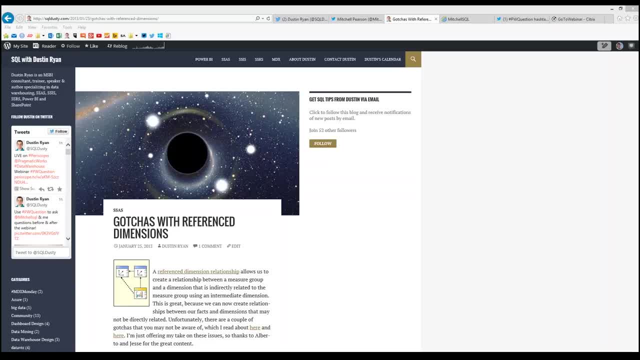 If you have further questions that we just didn't have time to get to here in the webinar, log on to Twitter hashtag PWQuestion. You can hashtag your question with that and then we'll try to get to those as many as possible. But thank you so much, everybody for coming to our webinar. 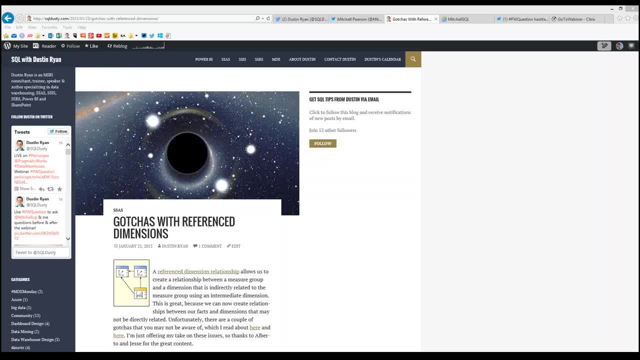 We hope that you found it useful. We enjoy doing these kinds of webinars, So if you have further questions about any of this kind of stuff, log on to Twitter, check out our blogs, go to pragmaticworkscom. Lots of great resources at pragmaticworkscom, and that is where the recording will be posted. 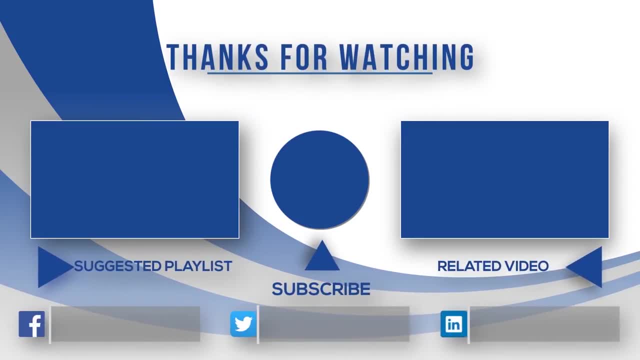 on pragmaticworkscom. Have a great day. Bye, Bye, Bye, Bye, Bye, Bye, Bye.